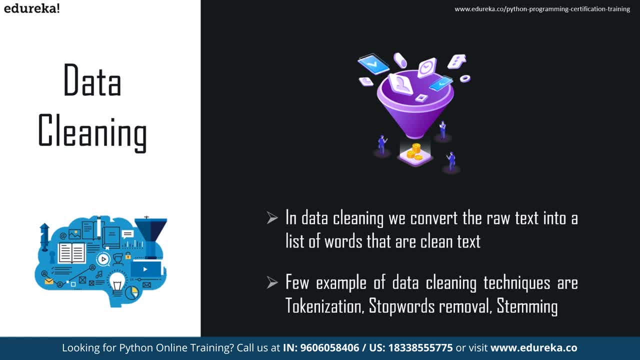 as mentioned earlier here, The goal is to convert raw text into clean text data. This involves steps like tokenization, stop-word removal, stemming and many more. speaking about tokenization, tokenization is essential for splitting a sentence or a paragraph. This is a process of filtering words or entire text documents into smaller units, such as 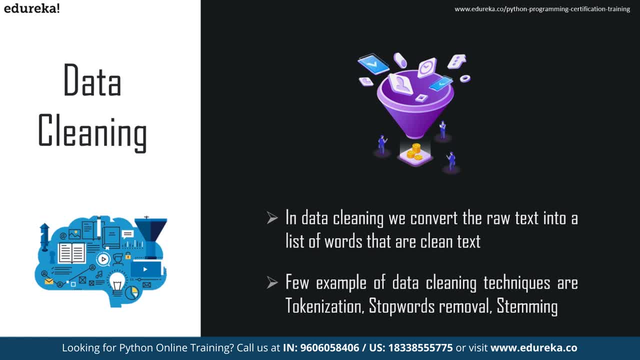 individual words of phrase. each of these smaller units are then called as tokens. Then we have stop-word removal. stop-word removal in general refers to filtering words whose presence in a sentence make no difference to the analysis of our data. So why do we have to remove them? 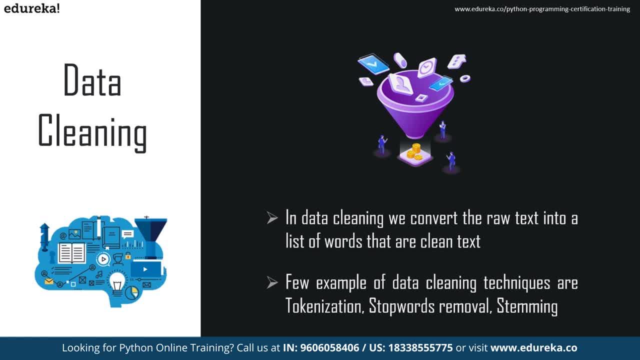 when we remove the stop-word, just so that you know our model doesn't get more complicated. in the next step We have something called a stemming. stemming is a process of reducing a word into its root form. What I'm trying to say here is which stemming? we are basically removing the prefix. for example, consider a word: giving. 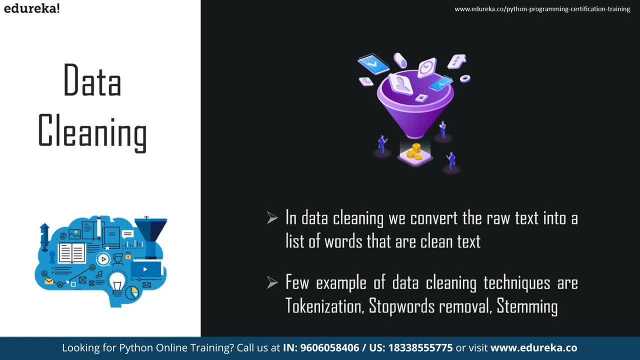 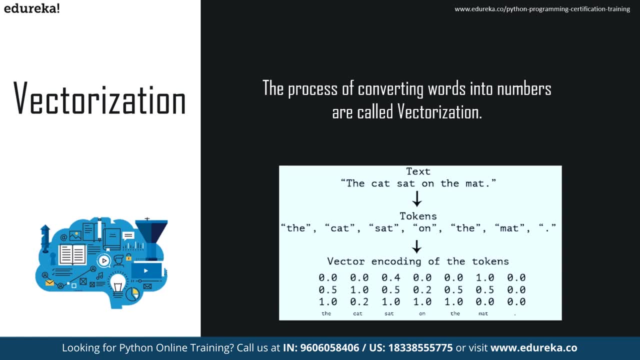 right. So once a stemming is performed on giving, the giving ends up becoming gift. moving ahead, We have vectorization: text vectorization is a process of converting text into numerical representation. here We end up creating something called as bag of word model, which is a model. 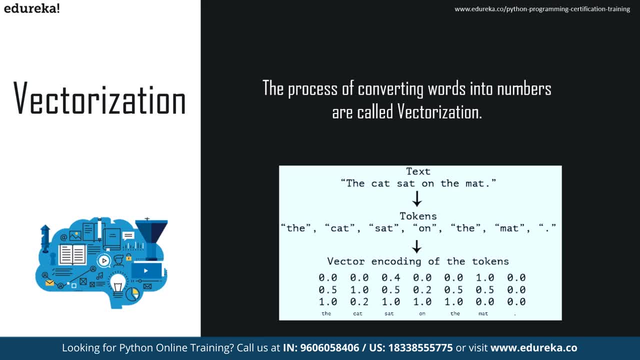 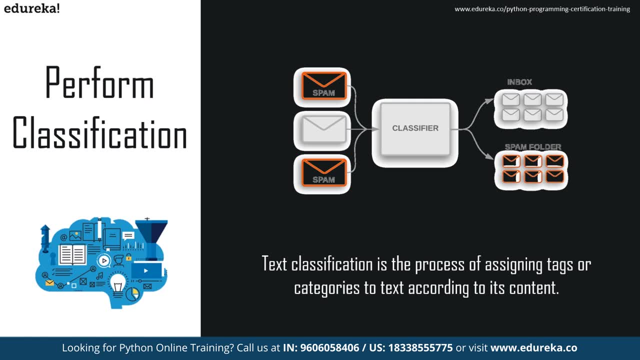 that signifies or represents a text and describes the occurrence of text in that word document. finally, coming down to classification task, text classification, Also knows as text tagging or text categorization, is a process of categorizing text into organized groups by using natural language processing. text classification can automatically analyze: 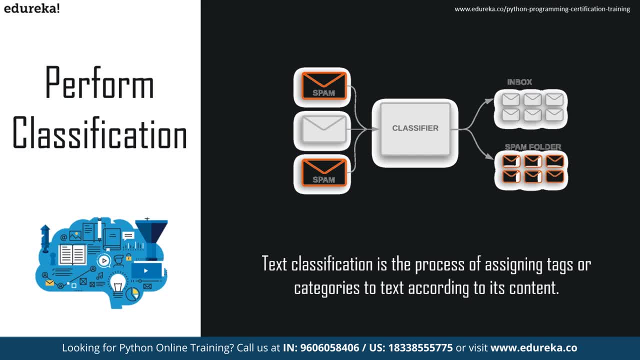 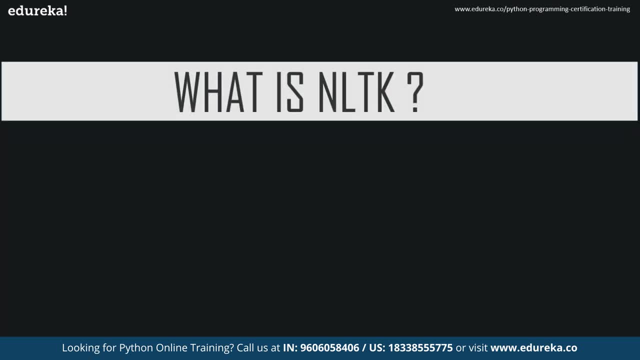 text and then assign a set of predefined tags or categories based on the content. Now let's move ahead and understand an open-source tool called as NLTK. NLTK stands for natural language toolkit. This toolkit is one of the most powerful NLP libraries, which contain packages to make 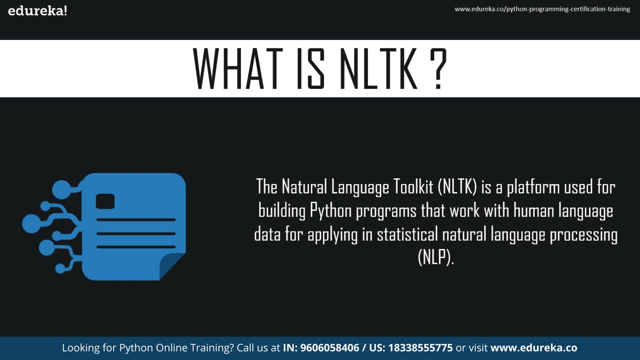 machine understand human language And reply them in an appropriate desired response. So why do we need NLTK? You'll see, NLTK has many built-in package to process our textual data at every stage. We can perform tasks like data cleaning, visualization, vectorization. that will help us in classifying our text. 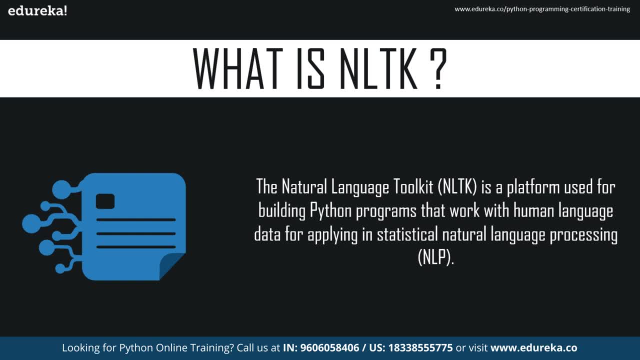 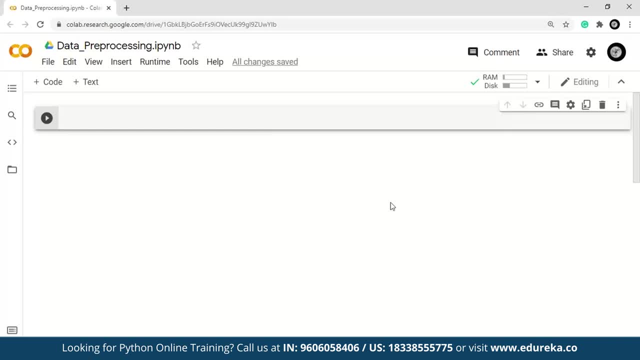 So let me now move to my code editor and show you how we can pre-process or clean our data using NLTK. All right, guys, as you can see, here I'm going to use Google collab- Okay, although you can use any of the code editor. 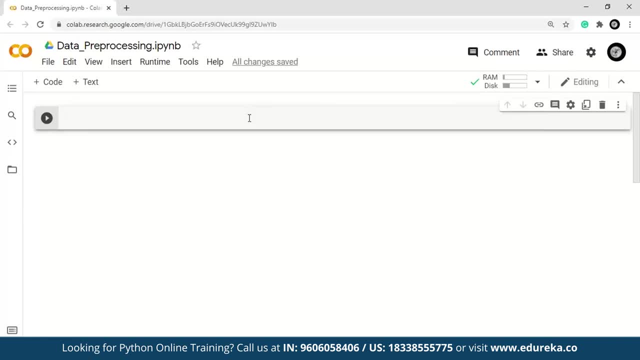 Keep it a notebook or Visual Studio code, but I would prefer to go with this. Okay, so the next stage. now we need a data set, right? So where will I get that? So, in order to get a data set, what I'm going to do is from sklearndataset import fetch20 news, right. 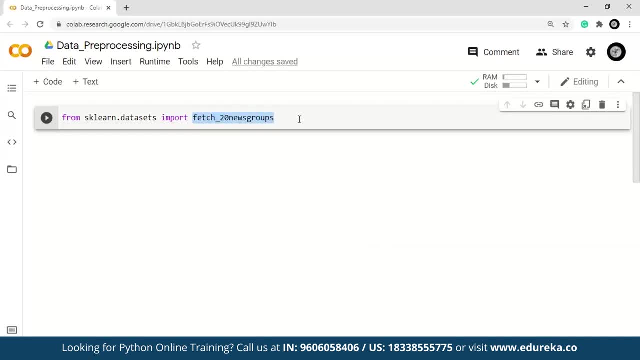 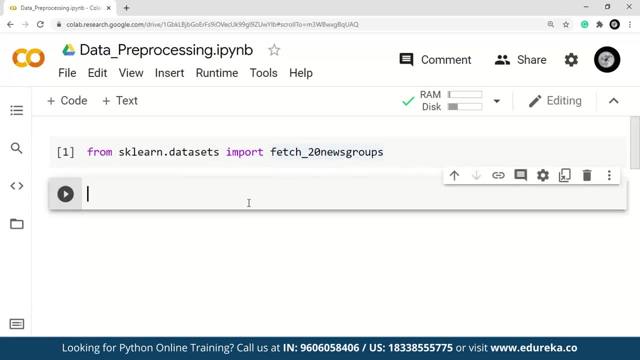 This fetch20 news groups will give us a data set, So let's quickly see how that would look like. All right, So if I have to execute this, I just need to press shift, enter. Okay, so let's see our textual data. 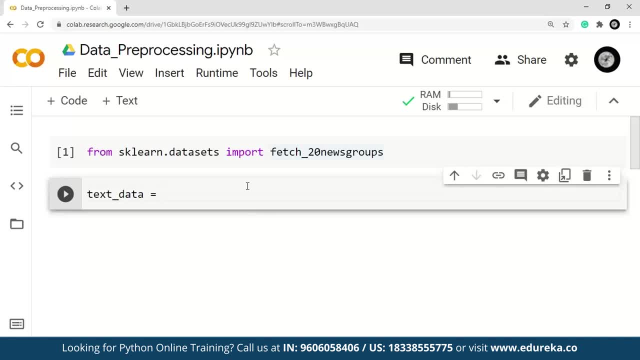 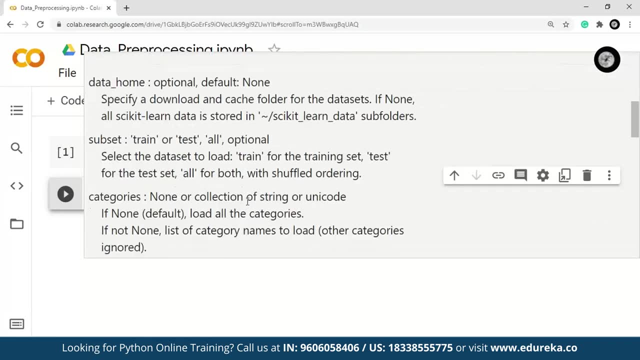 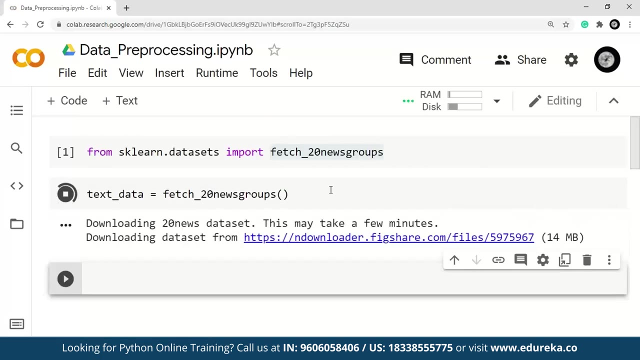 Okay, text data is nothing, but we are going to create instance of our fetch20 news group, So we'll copy this here and call it. So what would this return? this would return as a bunch- right, bunch- of object, So let's not quickly execute this If you're downloading this for 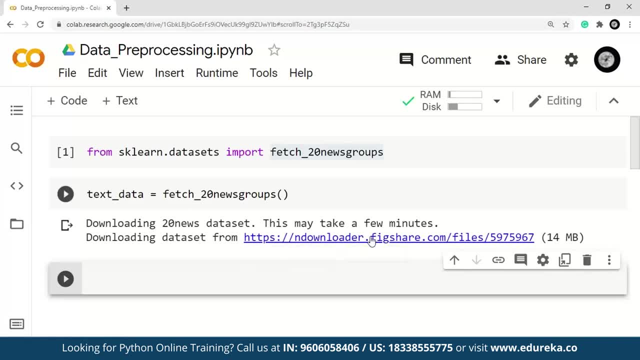 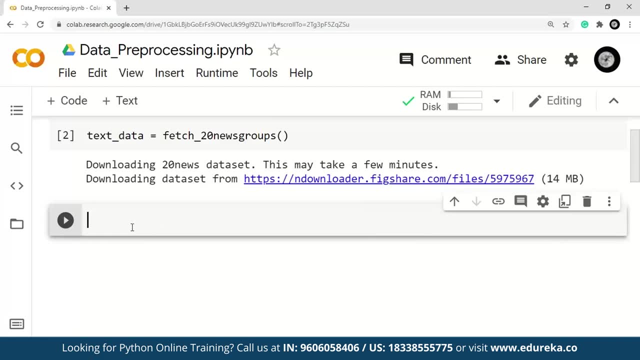 the first time, it will take some time to download our data set. Okay, and this data set is present in this particular link. fine, So this is done now. So let's quickly look at how this data would look like. Okay, So, in order to do that, we are going to use our like type data text, underscore data and. 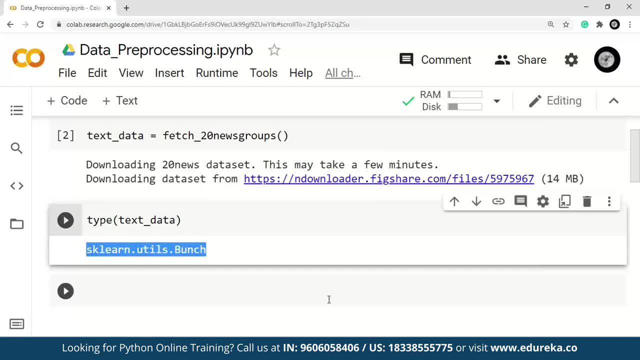 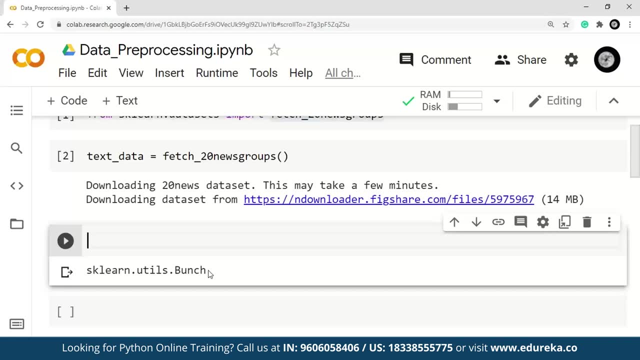 then you will see here This is a bunch. So let's now import our numpy and convert this back to a list, because we cannot perform any operations on punch right, We have to convert this into a list. So import numpy as NP, Let's execute this. And now what we're going to. 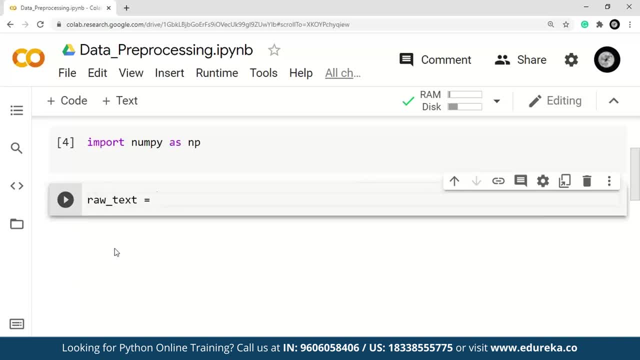 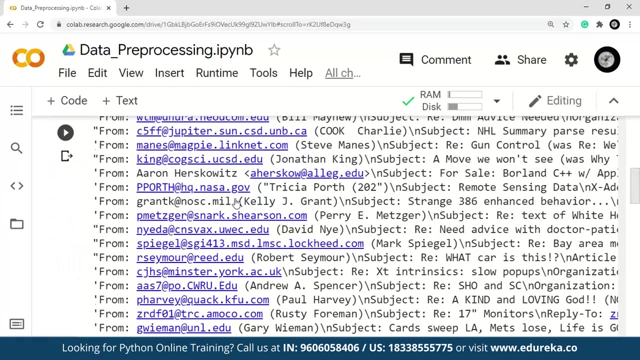 do is: let's give it as raw text. So raw text over here would be equal to text data. Okay, dot data: Okay. so let's print how this data would look like raw text. Okay, so, as you can see, here we have a huge amount of data set, fine, and all of these are 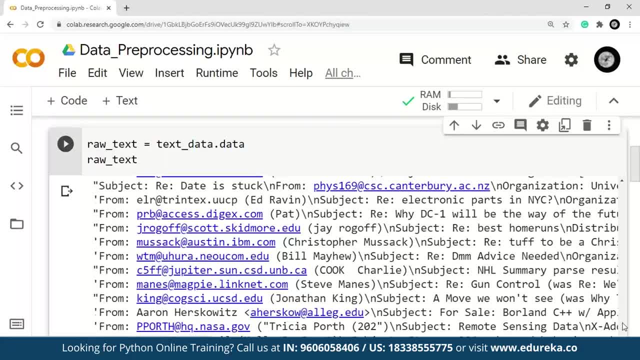 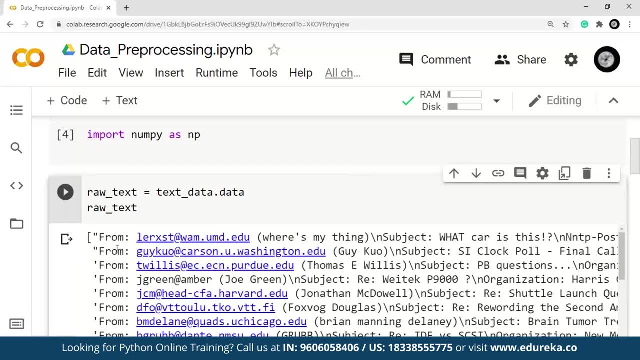 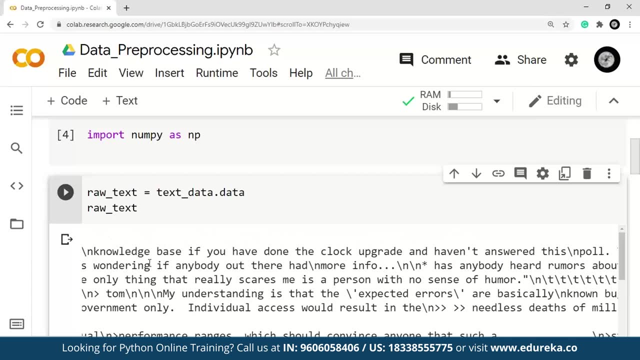 separated by commas. Let me quickly show you here. Okay, So, as you can see, first off we have a list, Okay, Okay, So we have a list. and then we also have a huge sentences, or you can say a paragraphs, which are separated by commas, and make sure you don't confuse this to CSV. and now what? 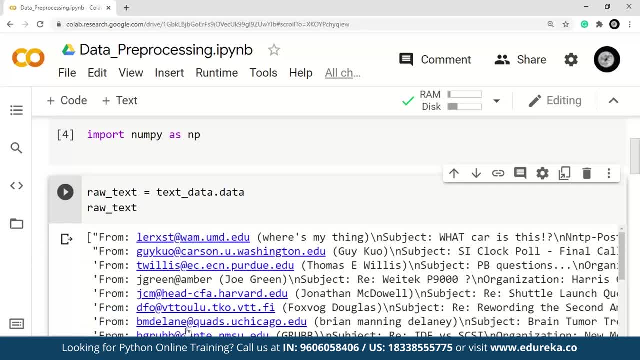 we're going to do is, as is a list right, We don't want to take the entire data set because it's going to be competitionally expensive and, apart from that, it will take more time to execute right. So, and to get a better understanding of what we're doing, We're going to take only first. 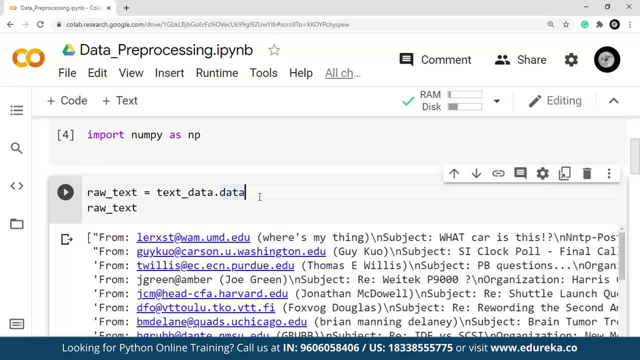 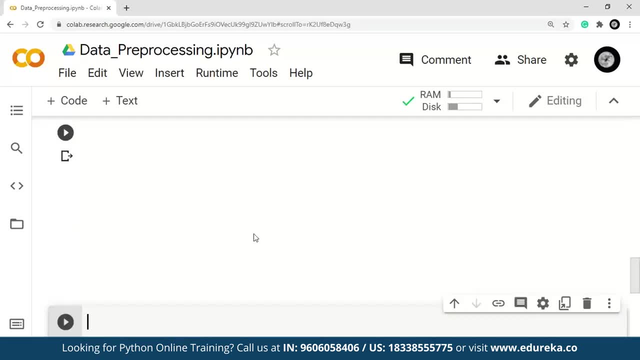 four paragraphs or sentences out say fine. So in order to do that, all I'm going to do is I'm going to use slice operation. I will call in and put four. So let's see how this would look like now. Okay, 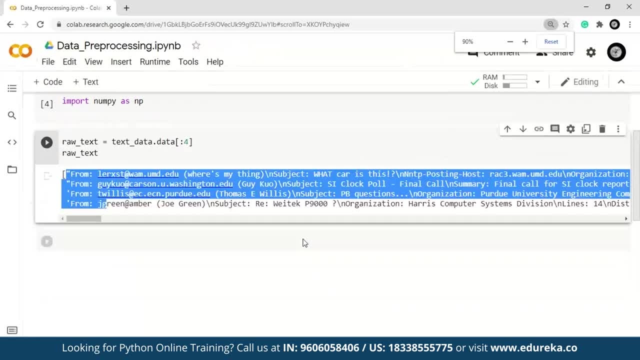 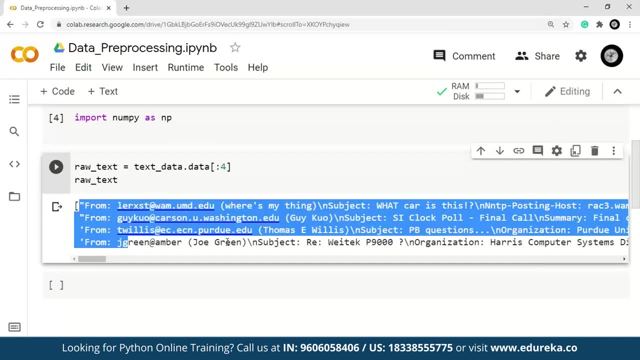 So, as you can see here we just have first four paragraphs or sentences. Let me zoom out here just so that you get a better view. So, yeah, fine. So now we have a text data and we are supposed to start cleaning our data, right? 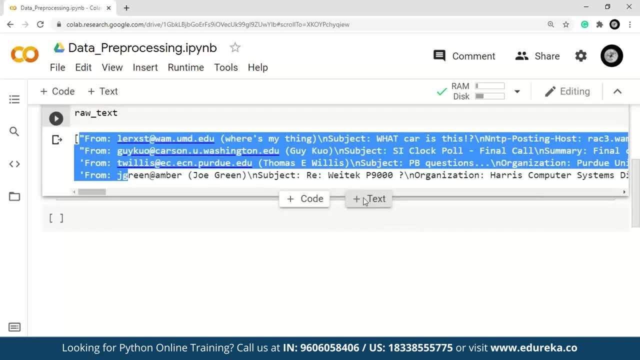 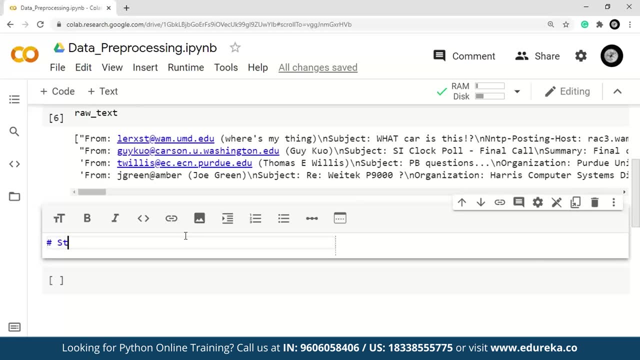 So let's start doing that. What we're going to do is, first off, let's reduce all the upper cases into lower case. Okay, So let me just give here a text and give a heading step, stage one: Okay, Convert into lower text, fine. 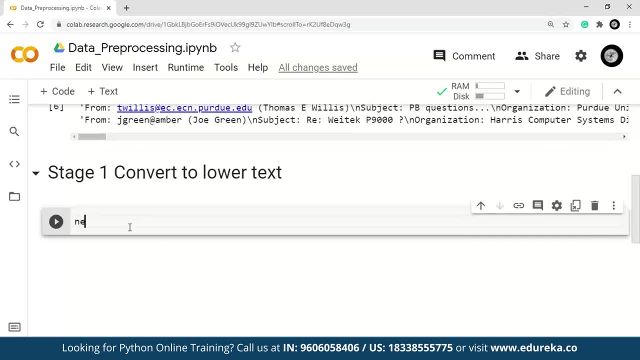 And now what we're going to do is in order to convert to a lower text. So we'll just give your lower text. So this is just going to be an array. Let's ignore this for now. So, as we're supposed to do this, like we are supposed to, no matter what input you take, 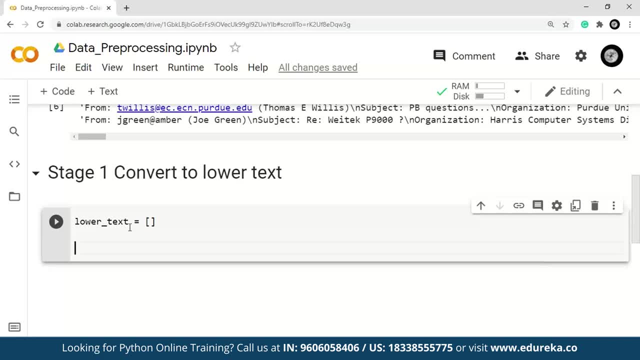 right, like whether it's for a training or a testing data set. you obviously have to convert it. rather than writing the entire code here, Let's give it a method so that you know next time if you want to lower our text. we just call the method. 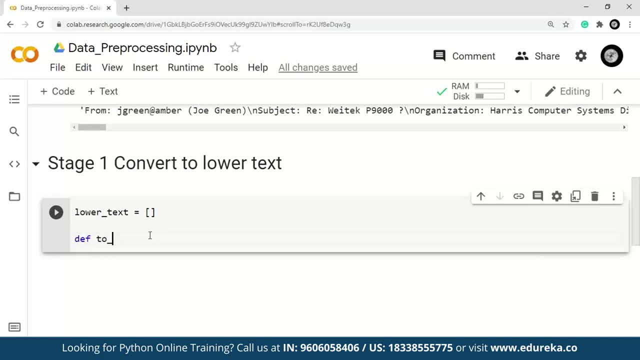 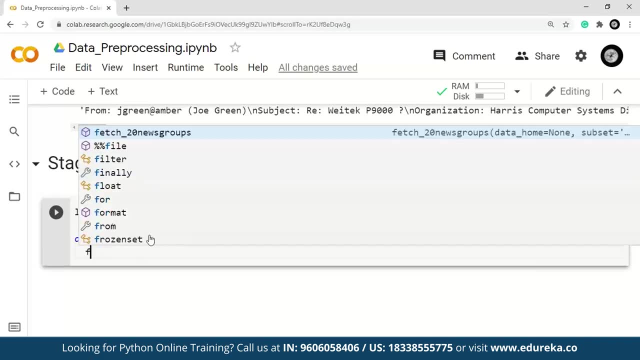 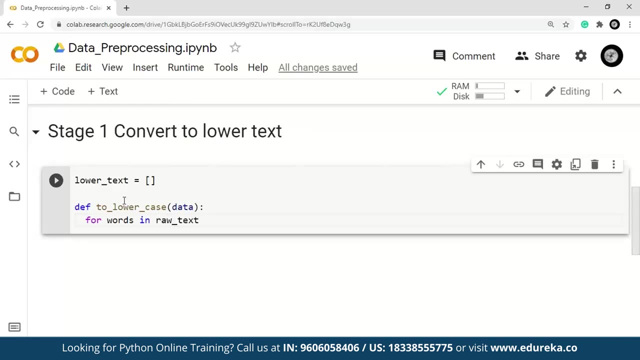 So def to lower- this is the name of our method- and then we are going to pass data here. That would be an argument. Okay, And we have a for loop now for words in this data set raw text. fine, for words in raw text. 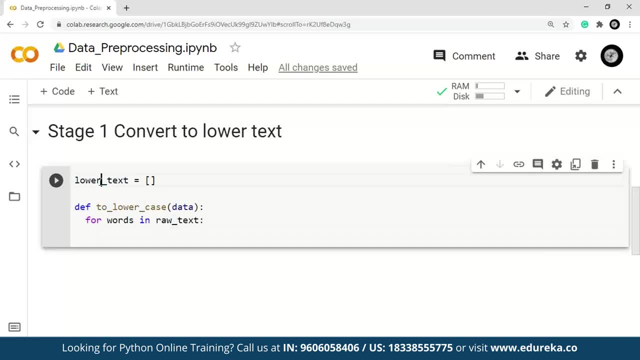 What we're going to do is we have to append it to this part, So let's give here as clean text in order to get a better understanding. clean text, stage one. So I hope this is fine. Okay, Let me quickly copy this: and we're going to append this part, not up in, okay. 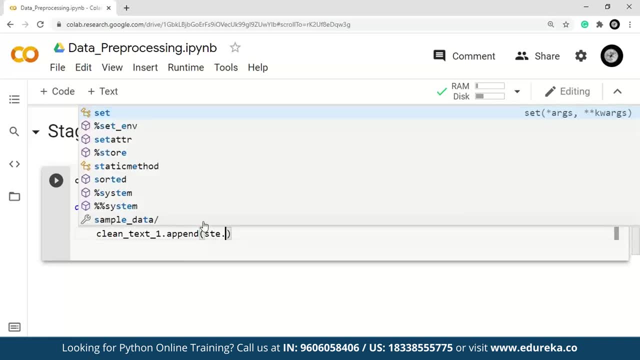 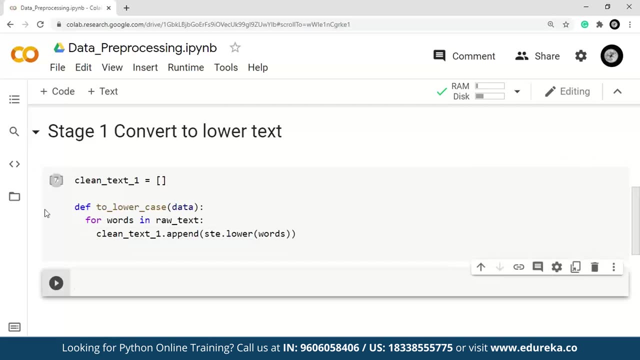 So we're supposed to convert our words into lowercase, right. So it's going to be STR dot lower is a built-in method and all we're going to do is we're going to pass this words. Okay, So now we have a method. 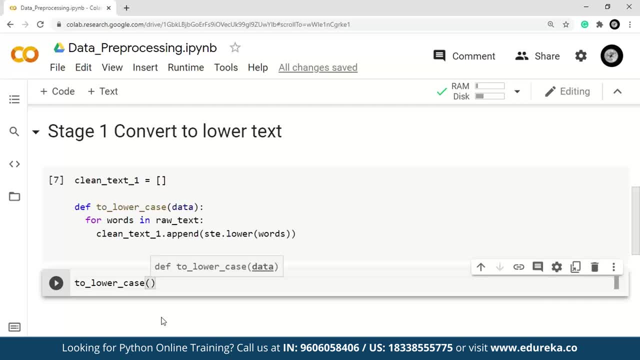 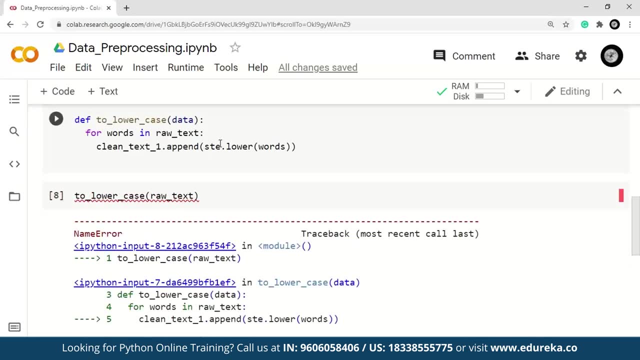 So let's call this method So to lower, and all we're going to do is we're going to pass our raw text input data raw text. Okay, so it's not. ste is going to be STR here. Let me quickly execute that once again. 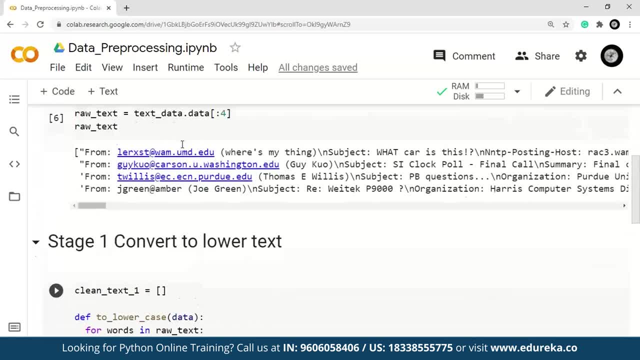 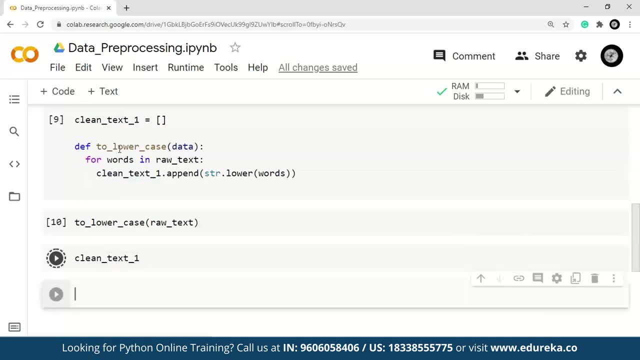 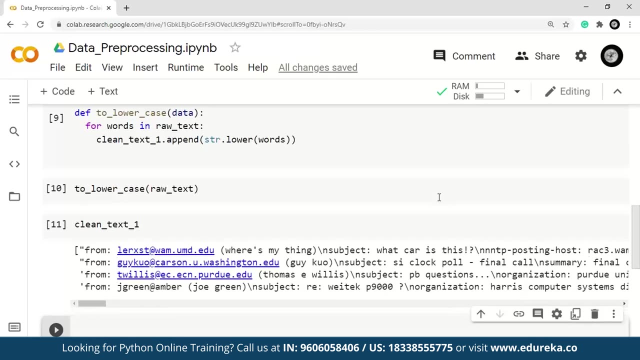 Okay, perfect. So now what we're going to do is let's compare our raw text with this, So we have something like clean text, stage one, right, CL en text. So let me execute this. So, as you can see, we have from, which is capital uppercase, and we have what car is this? and? 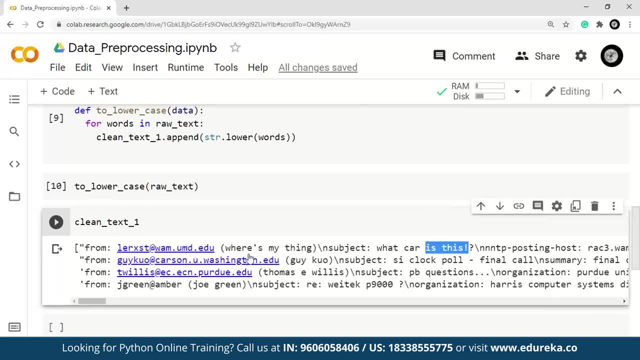 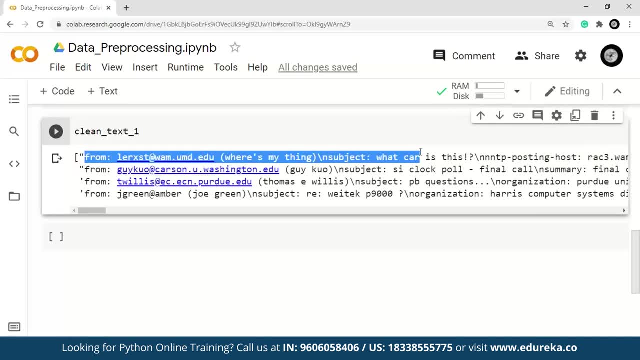 here everything has been converted to a lowercase. Okay, in the next stage we have tokenization, as I've mentioned earlier. What we do with tokenization is, whatever the sentence is there, Or a paragraph, we convert that into either, you know, individual sentences or into individual. 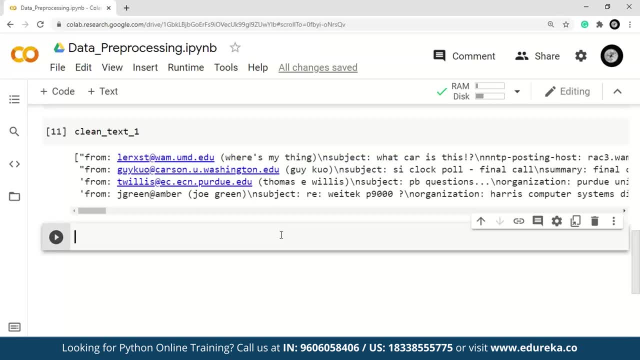 words. So in order to convert this into words, we have something called as word tokenizer, and to convert this into a sentence, we have sent tokenizer. So let me quickly go here and give this name of the next block as stage 2, and this is going. 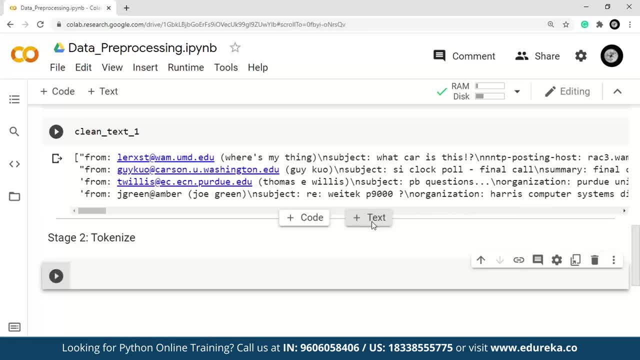 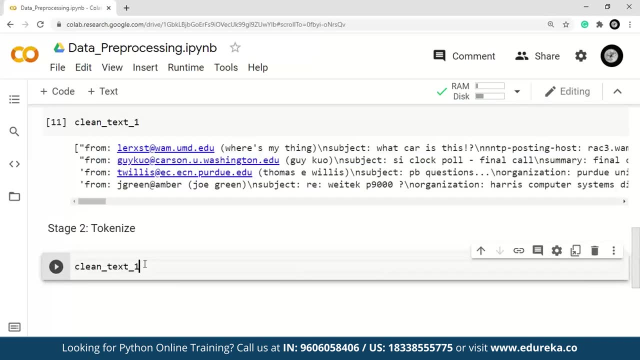 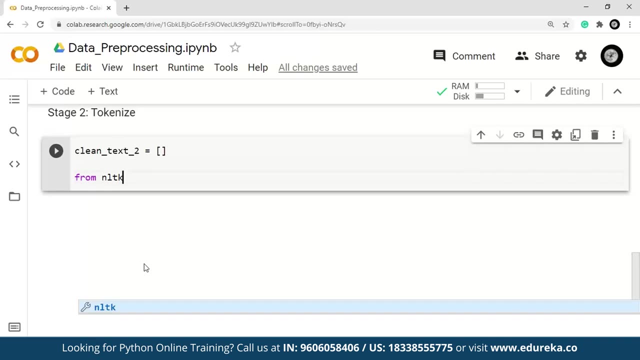 to be tokenized. Okay, and let's see how our tokens would look. like fine, same like before. we have to write one array here, So let's give it as clean text stage 2. And this is going to be empty. right, and now what we're going to do is, from NLTK dot, tokenize. 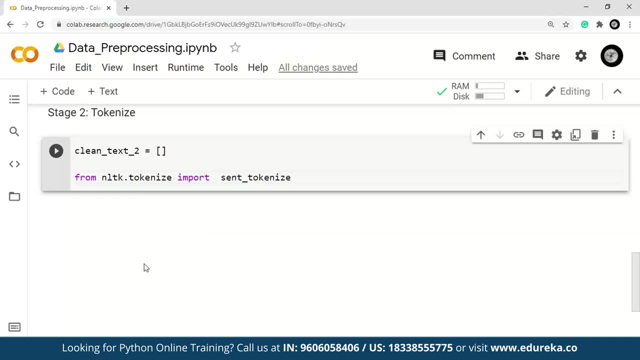 import sentence tokenizer. Okay, and then we also need word tokenizer, or? yeah, I'm going to show sentence tokenizer only for the demo sake. we are going to use word tokenizer in future, Okay. So before this, we also have to download something that's called a spunk. it. 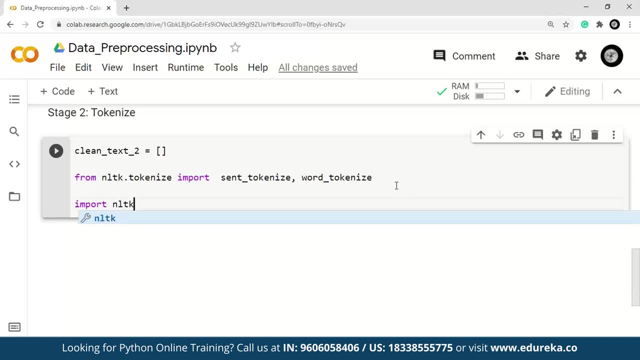 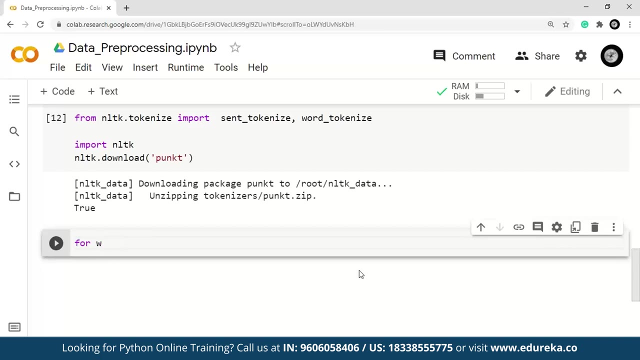 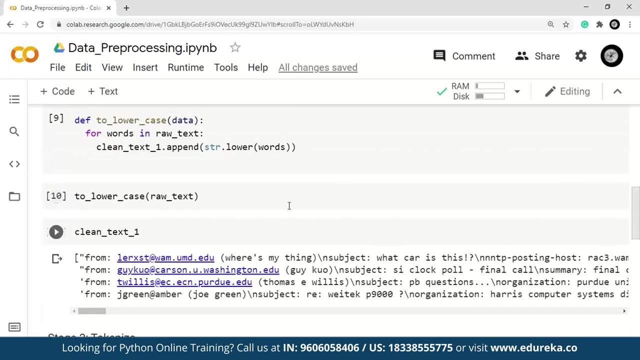 Okay, So import NLTK And then we have NLTK dot download. you have something called a spunk it and let me shift enter. All right. So now what we're going to do is we are going to perform sentence tokenizer. Okay, for words or sentence in. obviously we need this data right, clean text one. 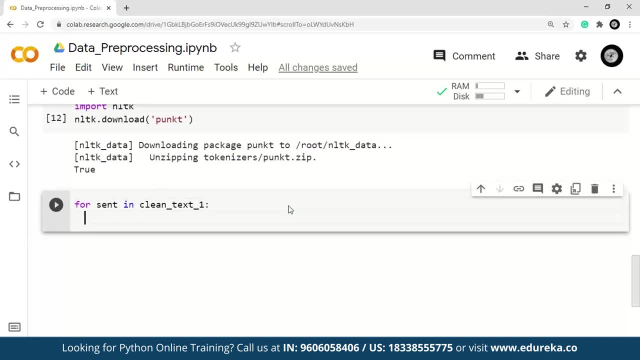 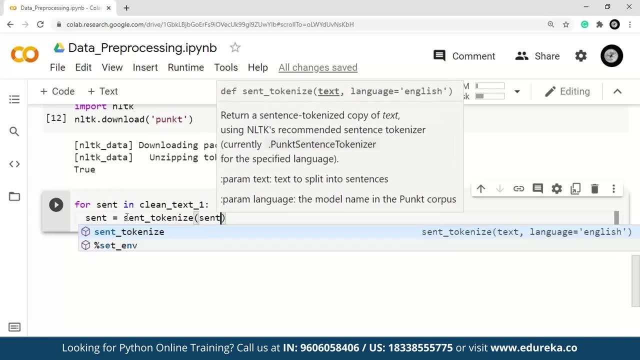 So clean text one. What are you going to do is sentence. you're going to use sent tokenizer, as simple as that, and we are going to pass this sentence. Okay, And now, in order to, obviously we have to store this somewhere. we are going to store this. 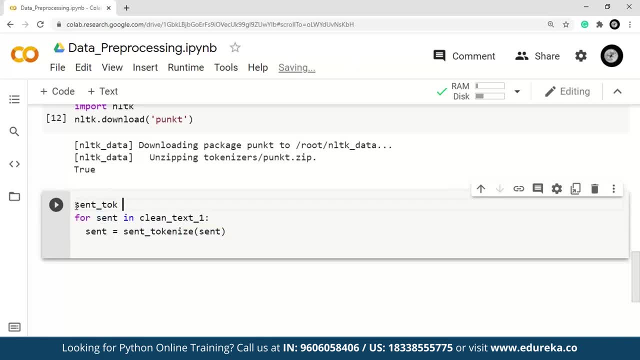 in a new variable here. sent tokenize. and this is just for showing you right, this is just for the demo. That's why I'm not going to use clean text. 3 over here, or two. Okay, So we'll append this. sent underscore you okay, dot append, and we're going to append sentence. 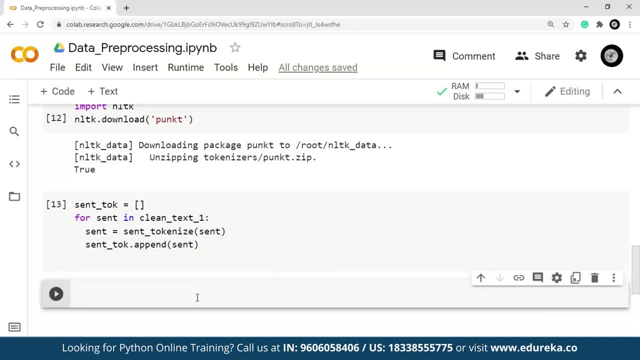 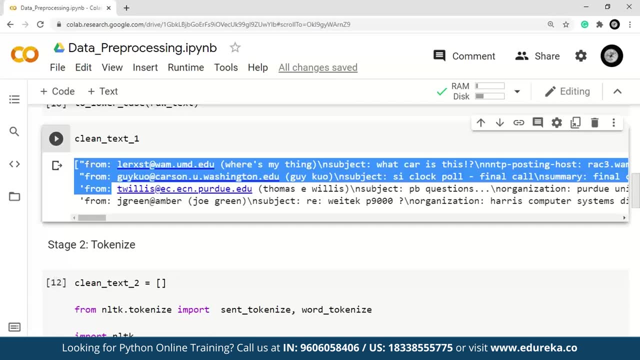 here. Okay, so looks good. So let's see how this would look like. So, as you can see here right earlier, We have a single dimension array, Okay, and here this, each of these over here, represents a paragraph. now, within a paragraph. 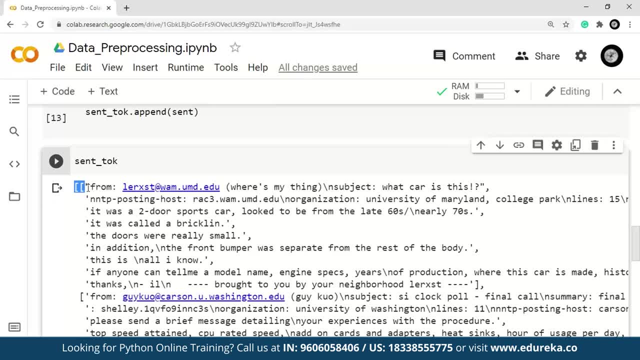 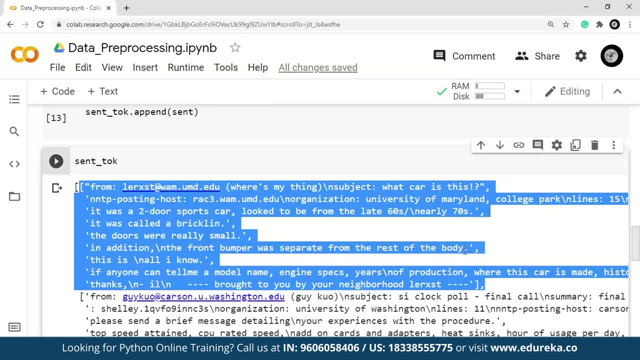 We all know we have multiple sentences. So, as you can see, now we have become two dimension array and each of this within this array represents a paragraph, and each of the sentence in this paragraph has become a word or one particular character. Okay, So now we'll do word tokenize and we move ahead. 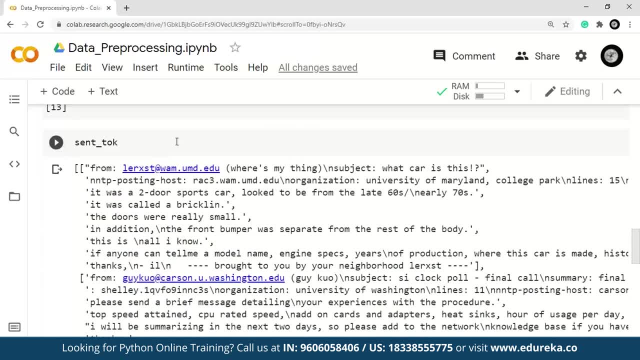 We need word tokenization, So we'll add this to a clean text to okay, because this is a part of our this thing. So what we're going to do Is we're going to perform word tokenization. So let me give a comment here. 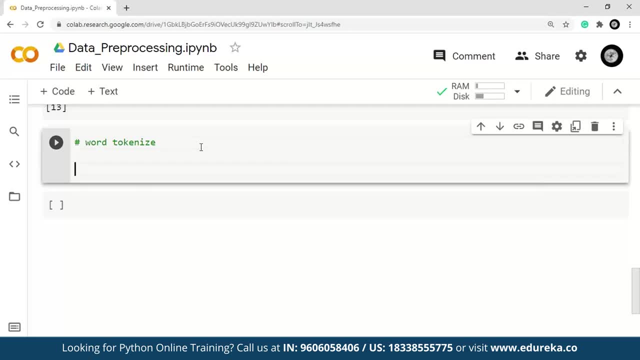 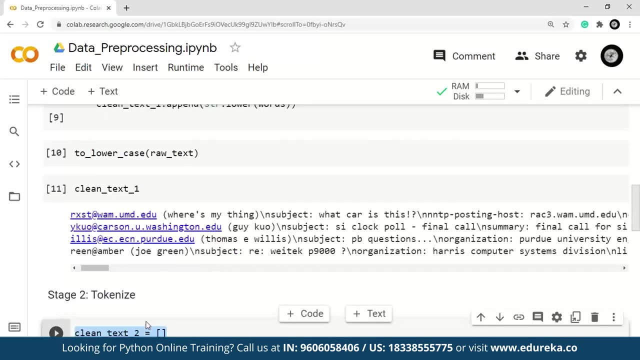 Okay, So now what I'm going to do is for word tokenize. you know, rather than writing this for loop, I'm going to show you a simple and easy way. what we were doing so far is we are initializing this array here and then writing a for loop and appending it right. we can also do something. 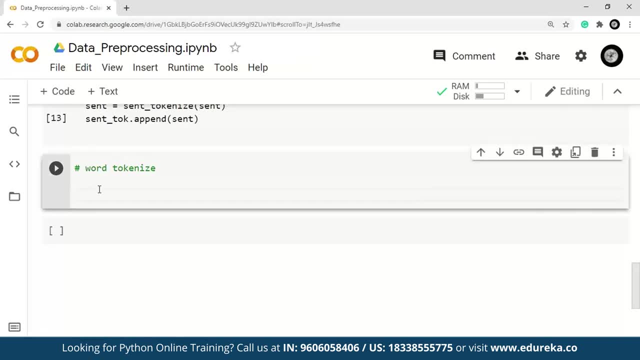 called, as you know, list comprehension. Let me just show you what it is. So we have this right, clean text to now in this comprehension, What will happen is the for loop. we write it within our list. Okay, So let's see word tokenize, and we obviously want some kind of textual data over here, which 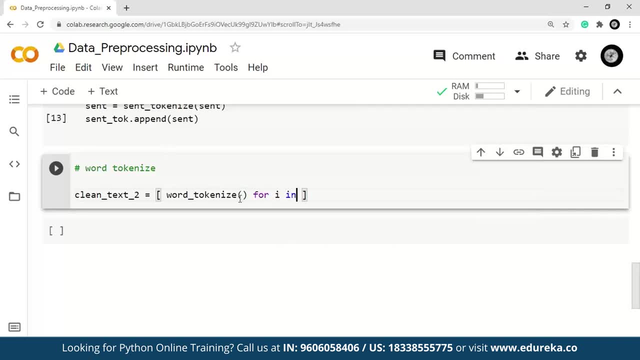 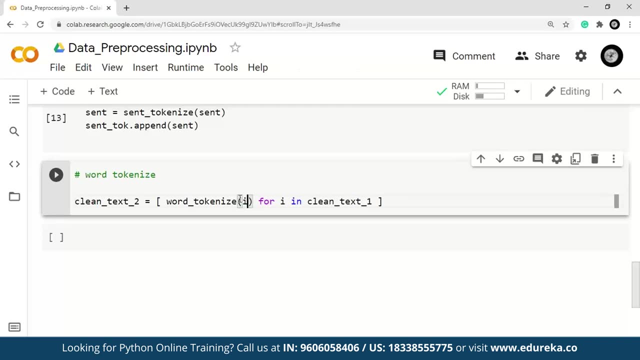 will fill it in a while, So over here I'm going to write for loop for I in clean text data, Okay, and now? whatever words that come out, or sentences, I want them to be tokenized. Okay. so let us now see how this clean text would look like. 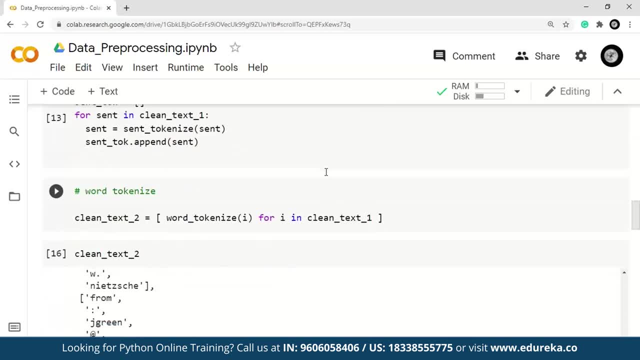 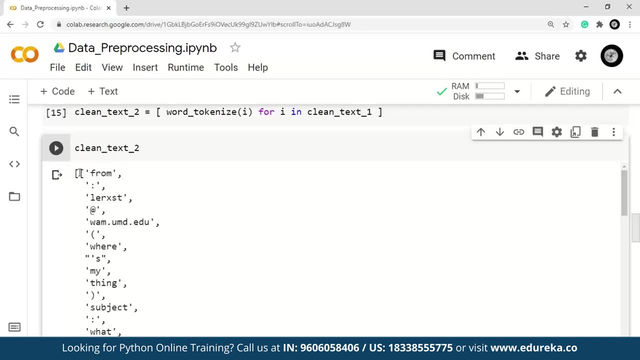 So, as you can see, here we have every word within the sentence converted into form of tokens. Let me scroll this up so that you can see how it looks. So still, it's a two-dimensional array. you know, whatever is there within this first, 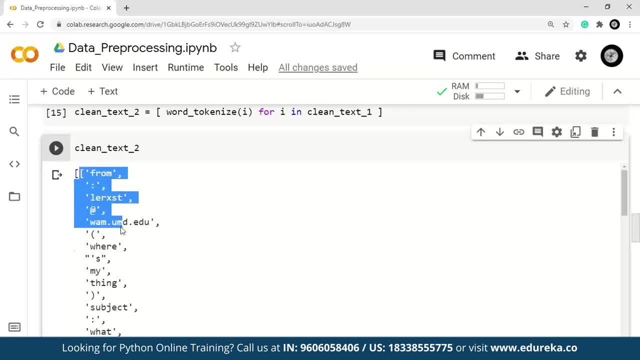 array here. within this array represents a paragraph. Okay, So everything over here has been converted into a single word: tokens. fine, So next stage. right, we want to remove some punctuations. you see, in our data set We have some special characters- punctuations. 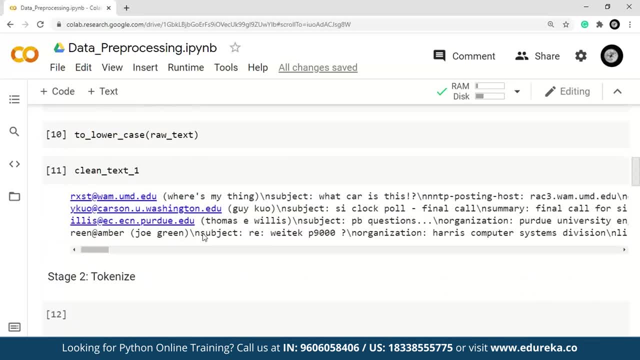 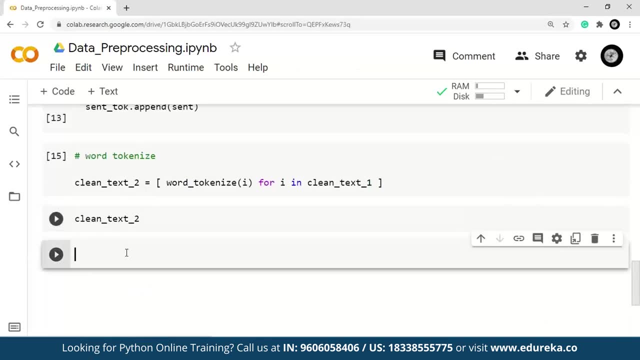 We don't want these edu's and dots. So in order to do that, we are going to use something called as regular expression. Okay, so let me quickly show you how we can implement this using regular expression. So, to do that, what we are going to do is we are going to import regular expression. fine, 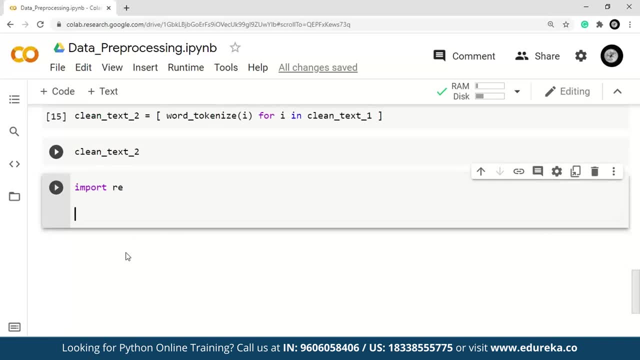 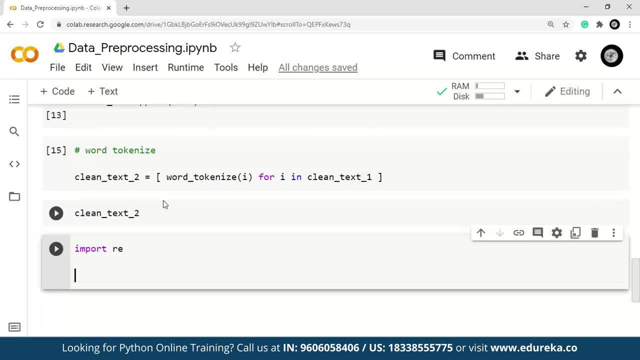 and now what we want is, as this is a two-dimensional data, So we need to for loops, unlike previous, had only one one dimension data, but now it's going to be 2d data structure. Okay, so we'll create something here, an empty list, which is clean text 3, and then we're. 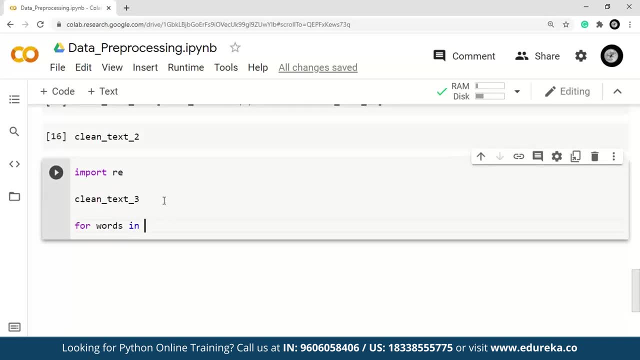 going to have a for loop, So for words In clean text to. we're going to create one array here and now. we're going to have another for loop to access inner words. right, So for W in words, now for regular expression. what we are going to do is we're going to 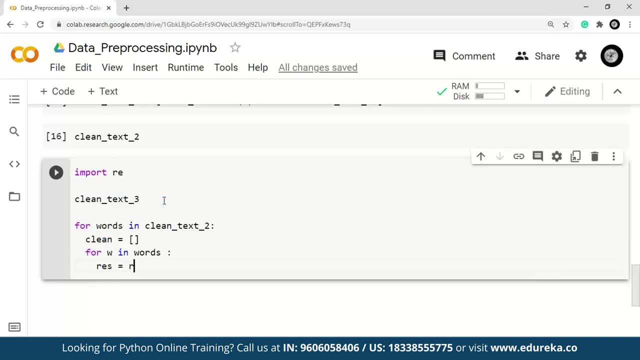 show a pattern. Okay, So re is equal to, so re dot substitute. So wherever that particular characters that we want to substitute it with something else, So re, dot substitute. then we have R, which is going to be obviously a comma. Oh, here, then we have a caret symbol, followed by W, followed by s. you want to replace this. 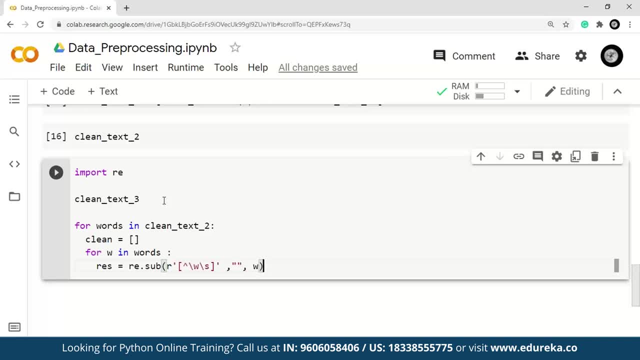 with an empty string here and then word: all right. and now what we're going to do is: if re s is not null, if re s is not empty, then what we want to do is we want to append that word. Okay, clean dot. append W. finally, we have to add this clean to our mean. 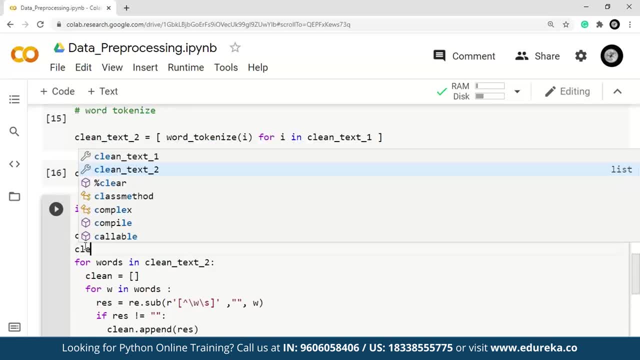 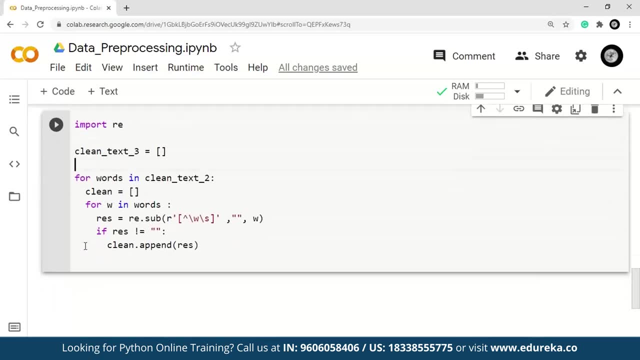 Array: Okay, So let's define that array as well. Clean text: Oh yeah, You have to give it an array here, correct? Fine, So let us now append this to our array, So it's going to be clean text. 3 dot append, and then we're going to pass just this clean. 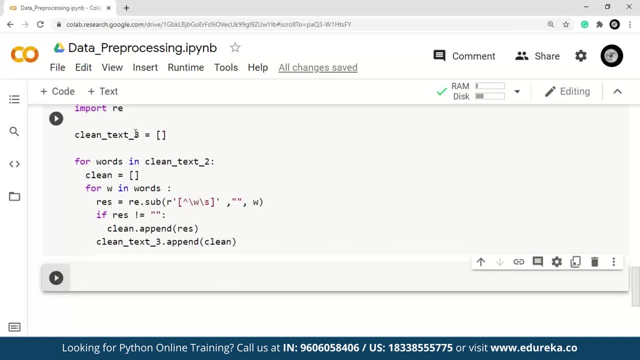 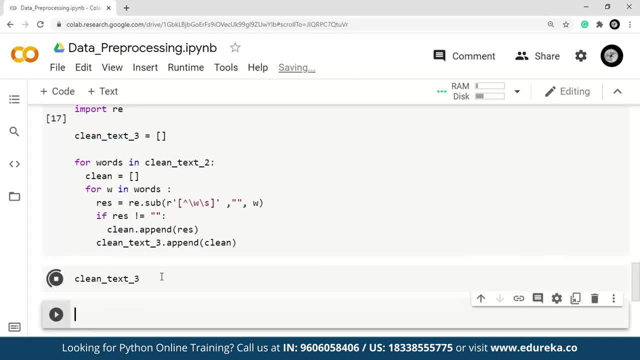 array here. Fine, Okay. So let's now see how our this thing looks like. So we have clean text 3, right, So clean text 3,. you know, according to our analysis, All of these semicolon, everything should disappear by now. 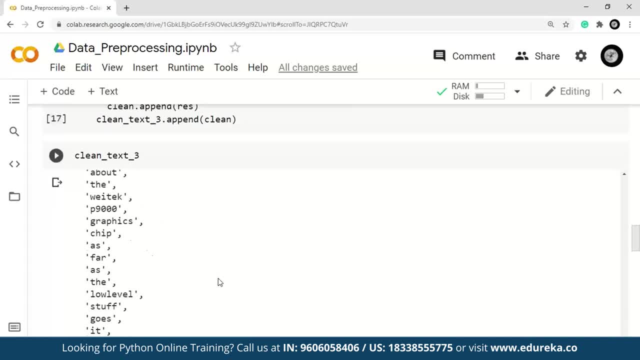 Okay, So, as you can see here, we don't have any special characters within our data set. Okay, still, this is a 2d array, but we don't. only difference over here is that we don't have any special characters, They have only alphanumeric values, right? 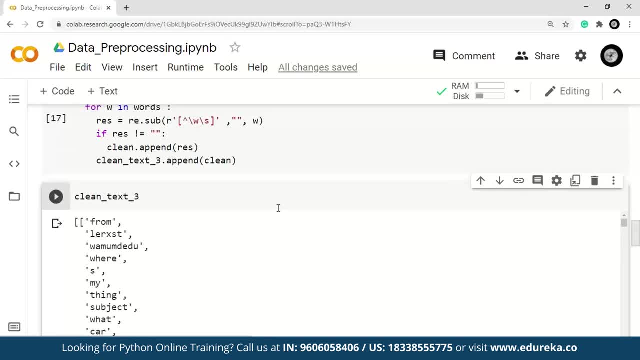 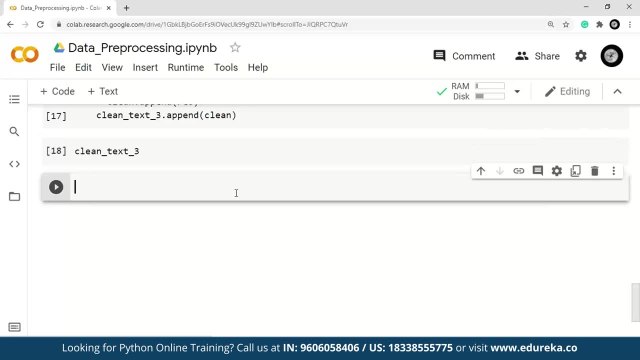 Okay, this is great. So in our next stage, we're going to remove stop words. I hope you remember what is stop words. As I mentioned earlier, stop words is nothing, but you know those words which are most commonly repetitive. Okay, So let me know. in order to do that, 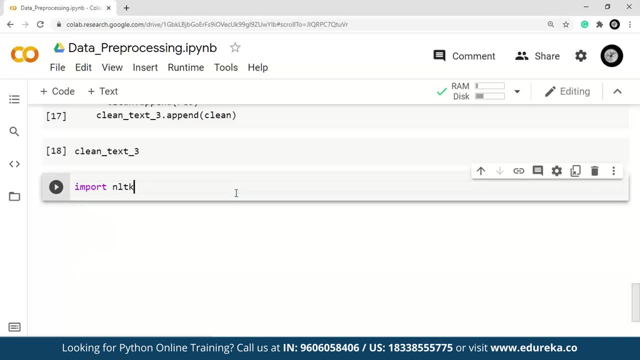 Let me just show you: import NLTK. Okay, we are obviously going to download this stop words. Okay, so we have an NLTK dot download and we'll download stop words. Although we can find the stop words on Google, what we can do is we can copy those stop words. 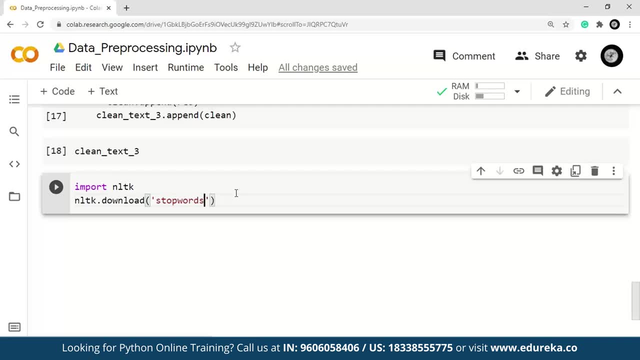 put them in the form of a list and if that stop word is present within our data set here, make sure you don't. We're going to put that in our clean text for stage wing. I had let me just give a title here for stop water removal. 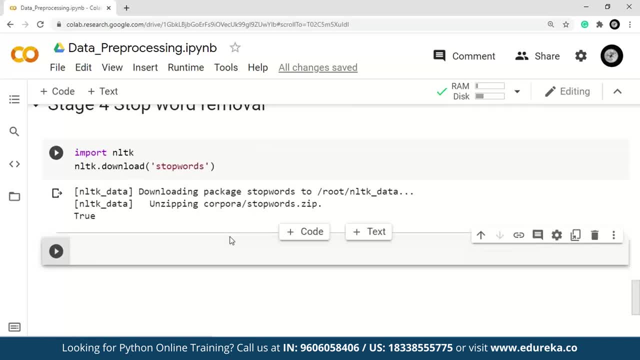 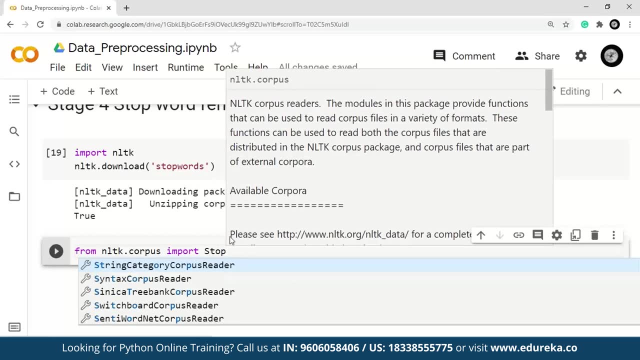 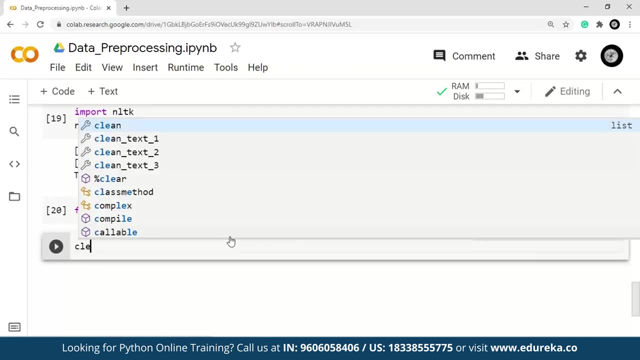 Okay. So now that we have downloaded our stop word, what we're going to do is, from NLTK dot corpus, import stop words. Looks great, right, Okay. So now what we're going to do is: we'll have clean text for okay, similar to the previous. 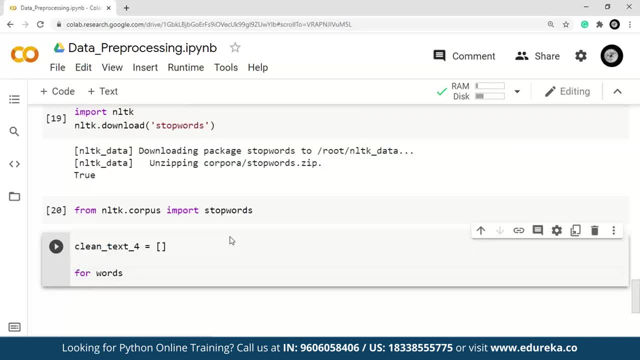 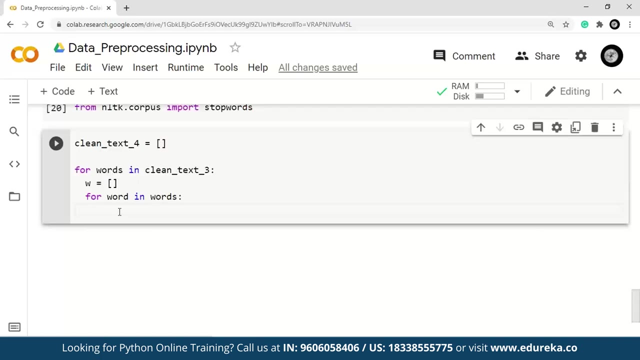 for loop. We are going to have for words in clean text 3 and then we'll just create an empty list which is going to be appended to clean text, for will have for word in words. If the clean text 3 contains this words right, the stop words you're going to eliminate. 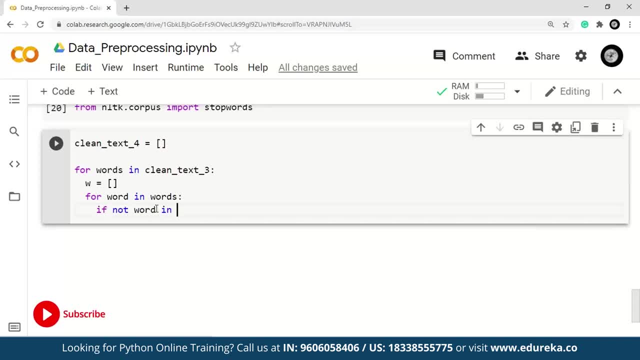 that Okay. So if not word in stop word, dot words here, we're going to pass the language, Okay. Okay, If the word is not present in this list, what are you going to do? is we're going to happen, because that means that word is not a stop word, right? 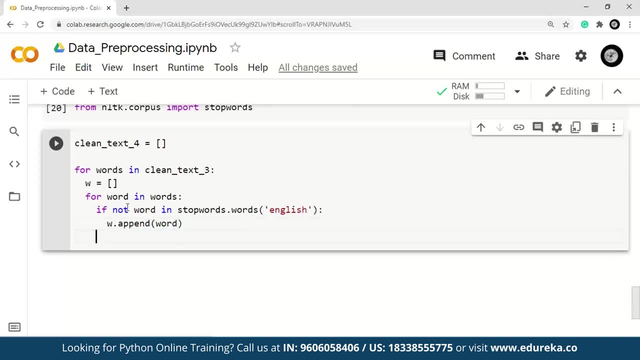 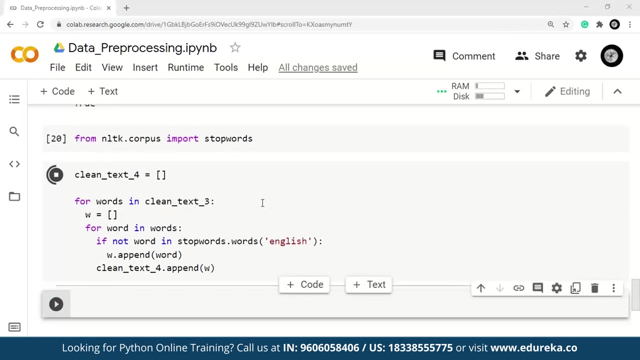 You're going to up in that word, Okay, And now we have to append this to our clean text for so clean text for not up in this list W. So let me quickly execute this. it would take some time to execute because it has to go through a lot of data set, right? 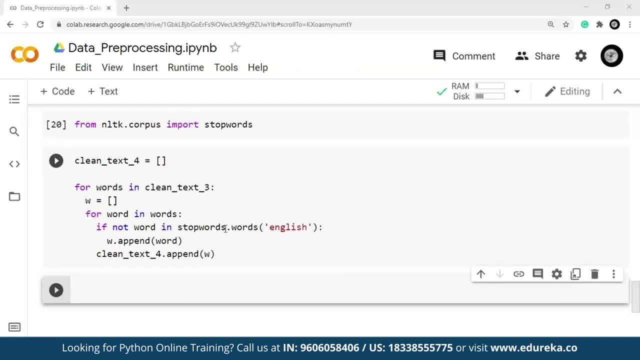 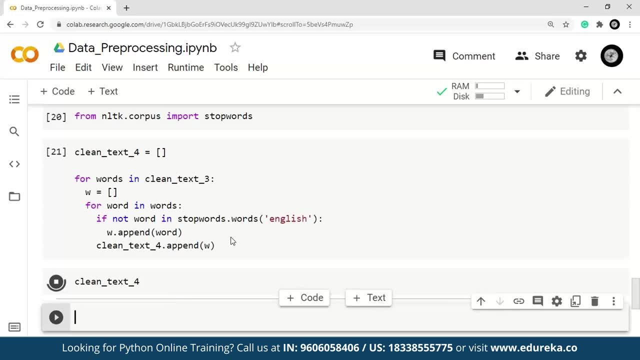 So please be patient And let's see What would it look like. Okay, So this is it finally executed, and let's now see how this would look like. So clean text for okay. So, as you can see, here we have removed a couple of unnecessary words and we have just 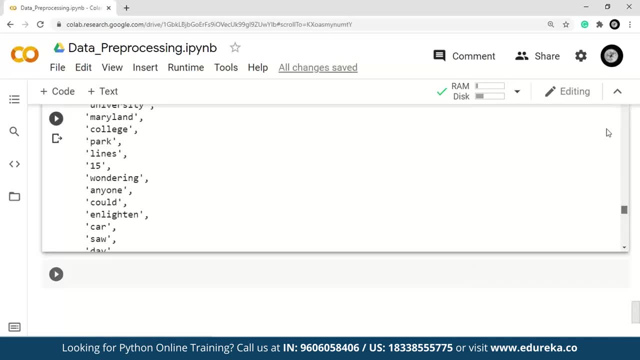 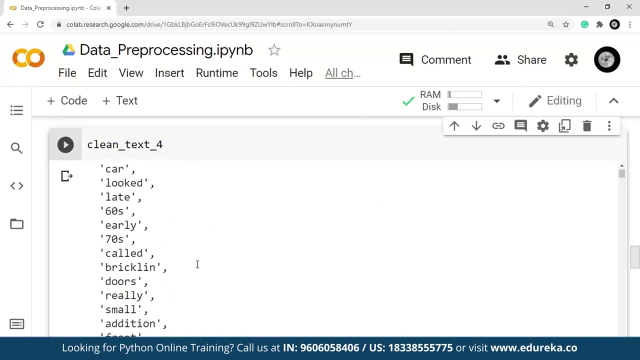 the important ones. All right now. so, as you can see, we have removed couple of words over here. Okay, So let's go back to our system. and yeah, so now moving ahead to our next stage, that is stemming. I hope you remember what is stemming. stemming is nothing, but you know whatever word we 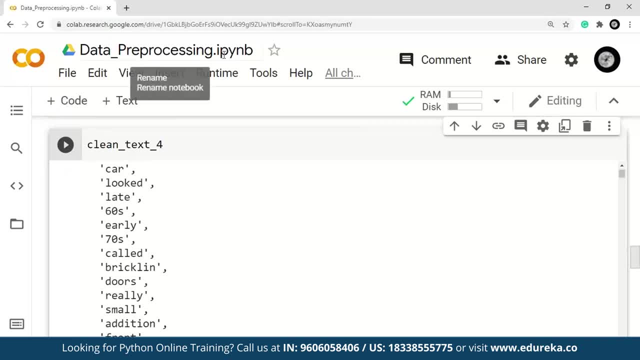 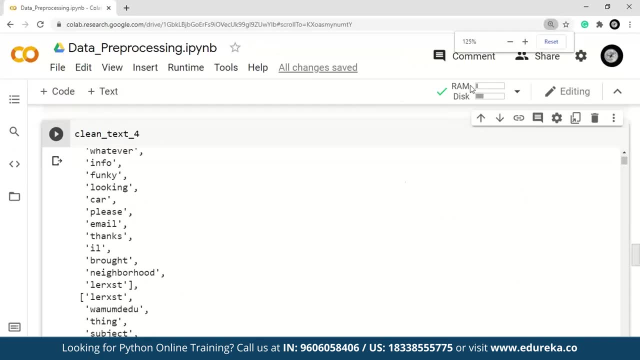 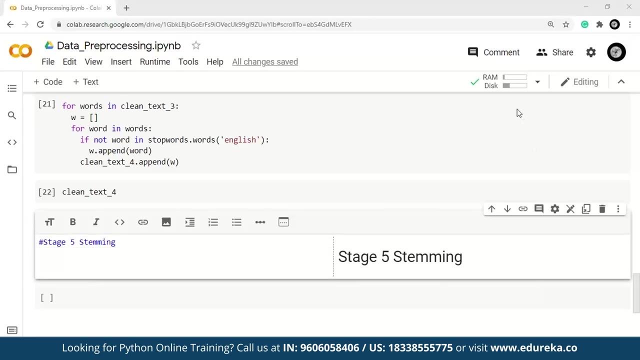 have. we have to convert that into a root form. So, over here, data processing is that after stemming, it becomes data preprocess. Okay, That's what is stemming. So let me quickly show you how we can perform stemming here. Okay, so, as I mentioned earlier, we use stemming. 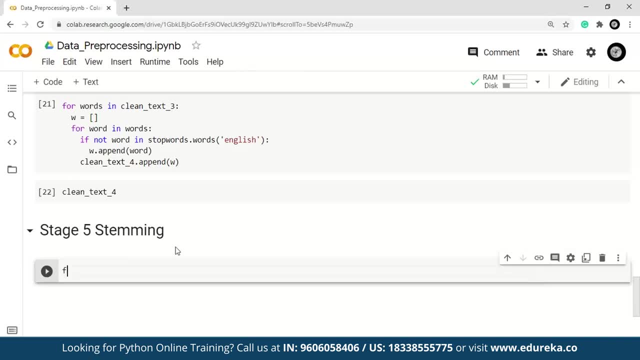 We use stemming just to remove this prefix right. So for, in order to perform stemming, we have various types of stemmers, So we have something like Porter stemmer, snowball stemmer, Lancaster stemmer. So today we are going to use Porter stemmer, right. 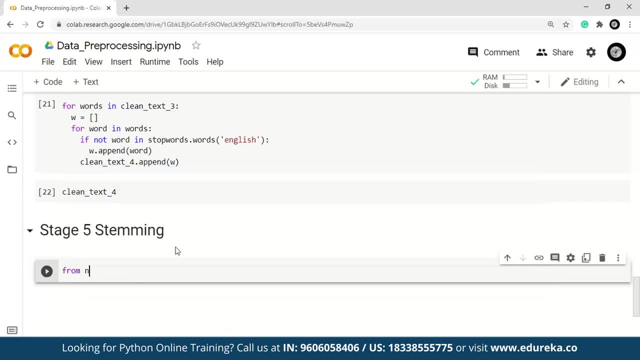 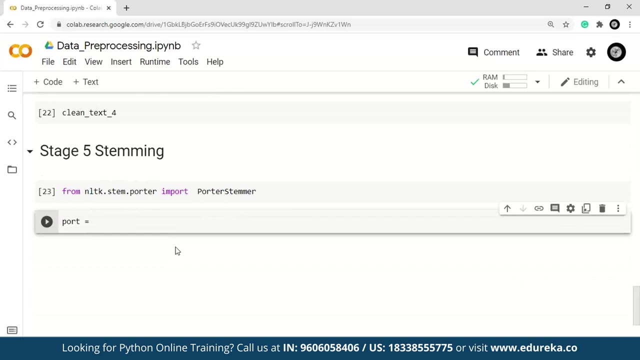 So in this particular example. so let's get that now from NLTK: dot stem, dot Porter. import Porter stemmer. All right, so once we have imported this, we are going to create an instance of our Porter stemmer. So port is equal to Porter stemmer. 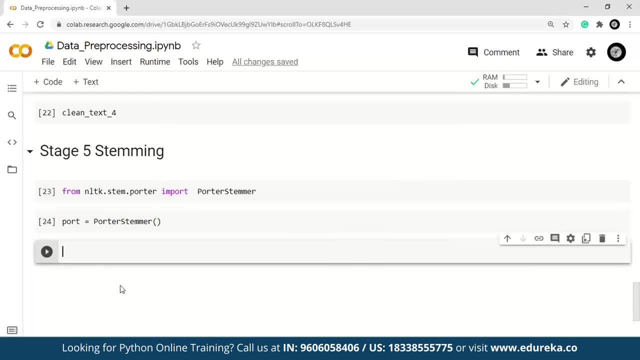 Okay. so just to give an example of what we're going to do here, Let's take three words, Okay. Let's take a list. Let's say: list is a right, So a has couple of words. rather than having words, Let's pass a list within our list. 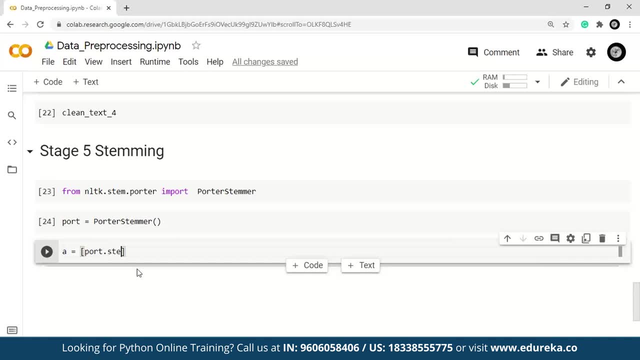 Okay, so we'll have port dot stem. This is how we call a stemmer. Okay, and here we're going to pass the word that we want to stem, right, and now we are going to have for loop for I in. okay, So now let's pass couple of words like it should be, like reading washing. 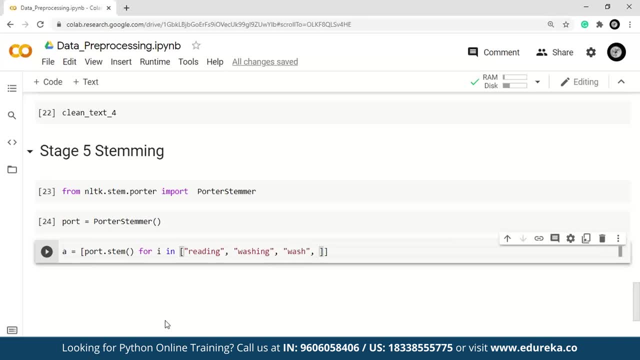 Let's give one word which doesn't have a prefix like wash and let's give driving. Okay, so let's now print this. So this is going to be I here, and what output that we are I'm expecting over here is that reading should be converted into read, washing will be converted to wash and then wash should. 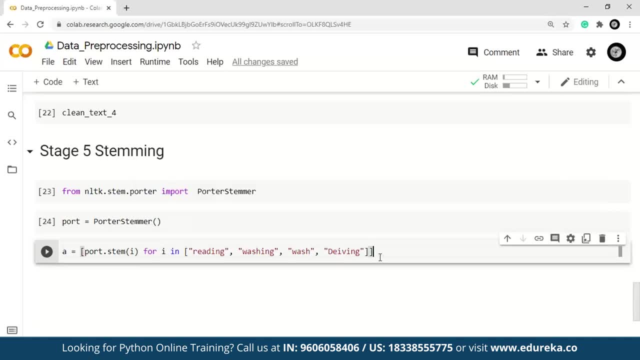 remain the same, because there's no prefix and driving would be converted to driving drive. So let me just print here and execute This part. I hope you can see this. it: read becomes read, wash remains wash and rest. everything remains the same. Okay, I have done a small typo here. 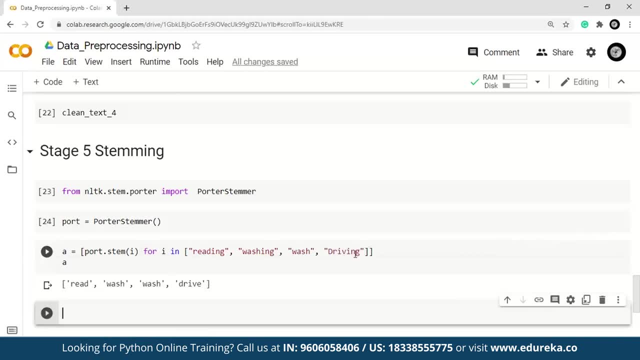 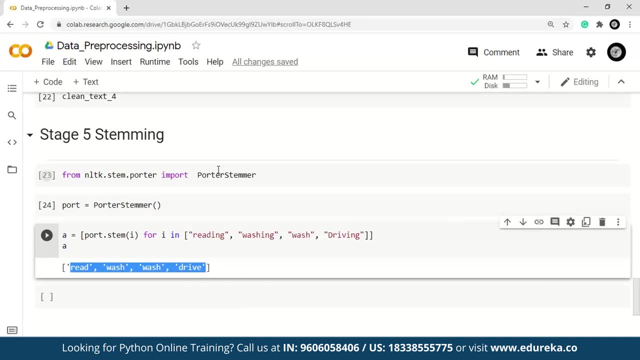 So it's going to be driving, Okay, So let me execute this once again. So, as you can see here, we have successfully removed all the prefix and they do make some sense. Okay, This is the case in case of port stemmer, but this doesn't hold good for when you're. 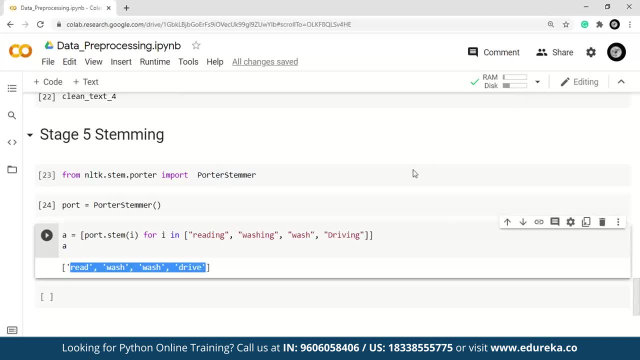 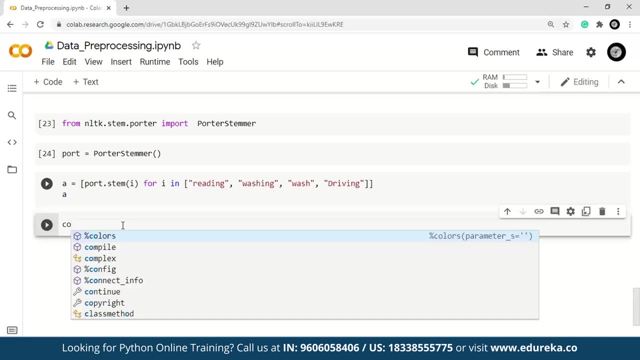 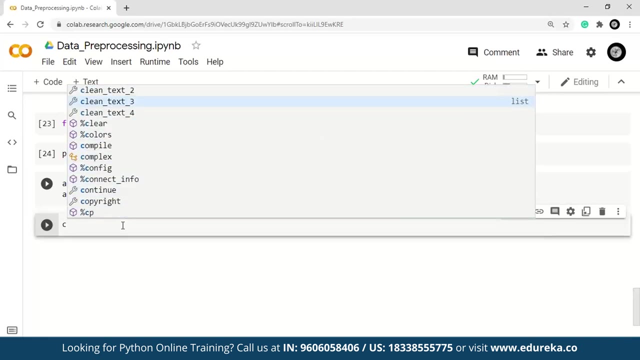 trying to use Lancaster stemmer or snowball stemmer. So let us know, quickly move ahead and see how we can implement the stemmer in our data set here. So we all know we need our loop here. Okay, so before that, we're going to have array, so clean text five and it's going to be an 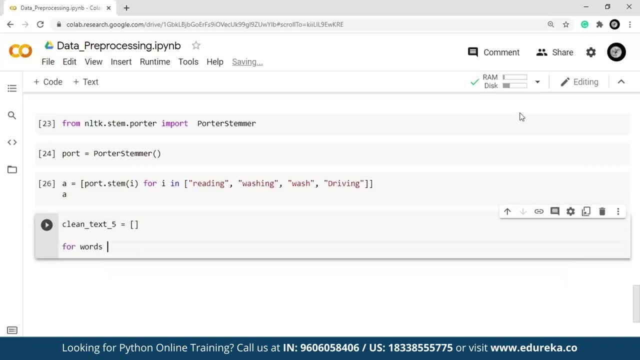 empty list. So now we'll have a for loop and another empty list, Okay, so now we're going to pass this list and we're going to append- so it's going to be W dot up and it's going to be word. Okay, and now we're going to append this smaller list to this one. 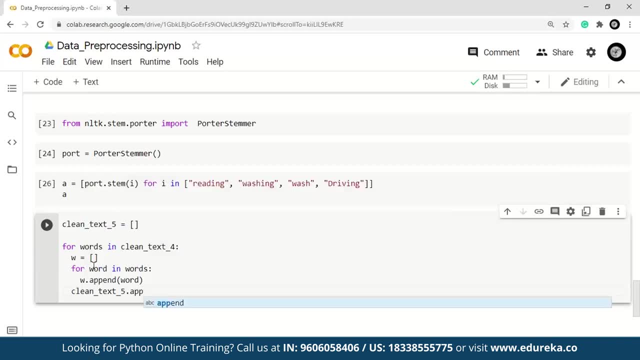 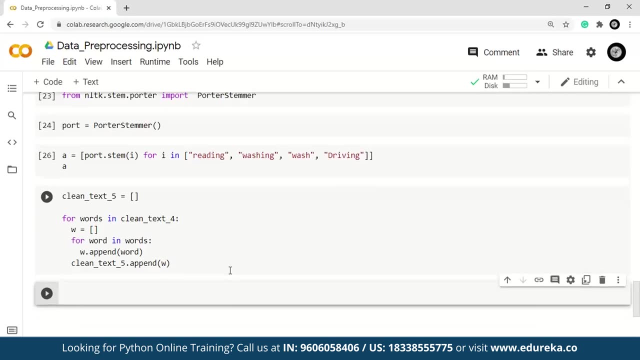 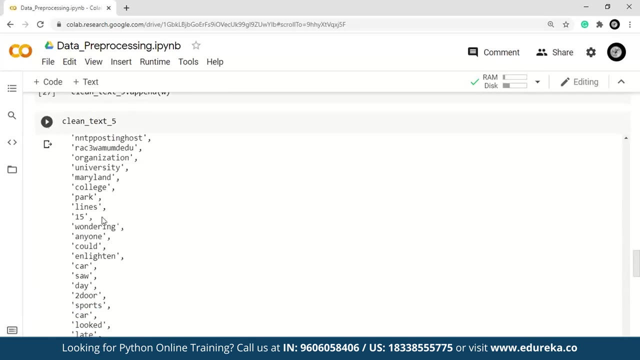 So clean text: five dot up and W. Oh, this is done. right, Let me quickly execute this, Okay, and let me see how this clean text file looks like. Okay, so, as you can see here, we don't have any more. 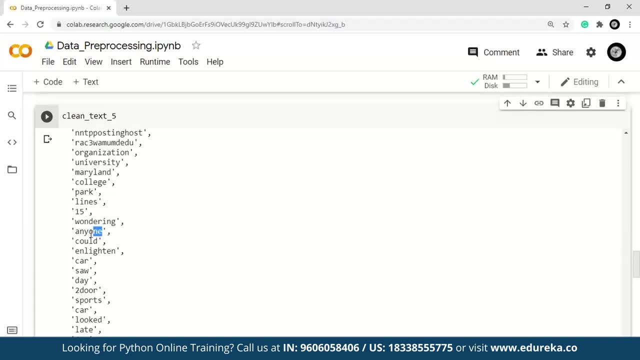 Yeah, Obviously there are some errors. That's because You know this timer might not recognize it. That's why we have multiple other stemmers. but most of the places you can see, you know our words have been converted down to the stem words. 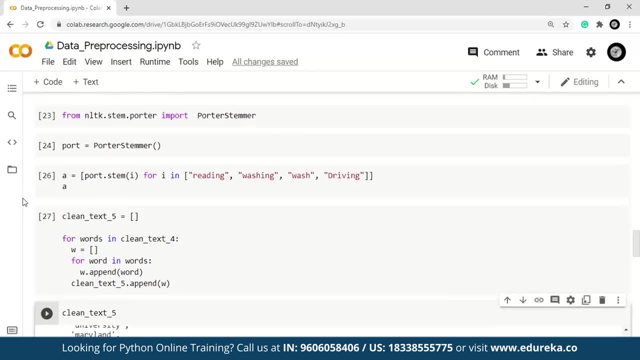 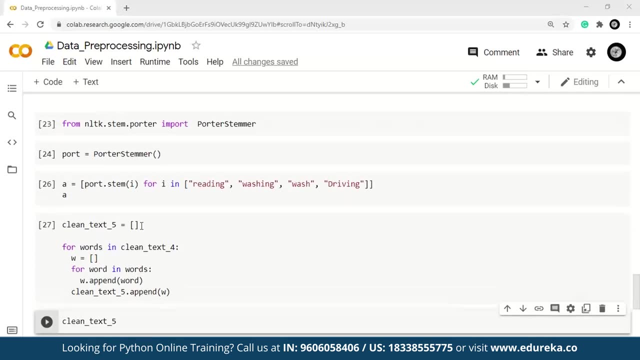 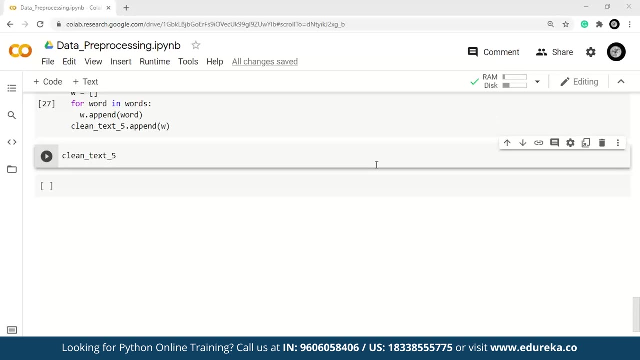 All right. so I hope now you understood how to perform stemming. but you know, as I've mentioned earlier, we have multiple stemmers. We have like Porter stemmer, We have like Lancaster stemmer, and each of those stemmers are unique in their own way. 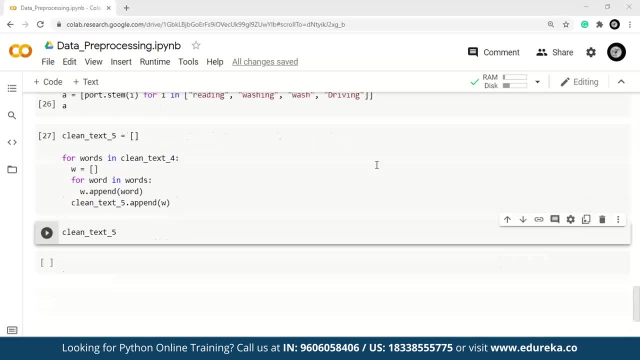 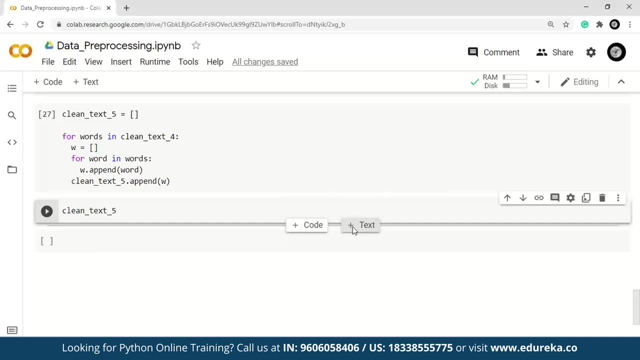 Sometimes what happens is, when we perform stemming, We get words which makes no sense right, and that thing can sometimes be a really annoying. So in order to overcome that, we have something called as limit ization. So let me quickly show you what limit ization is. 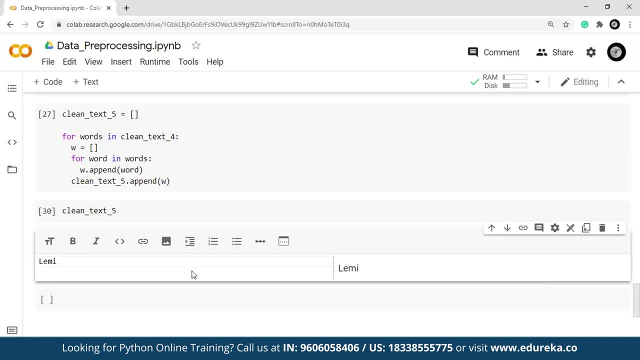 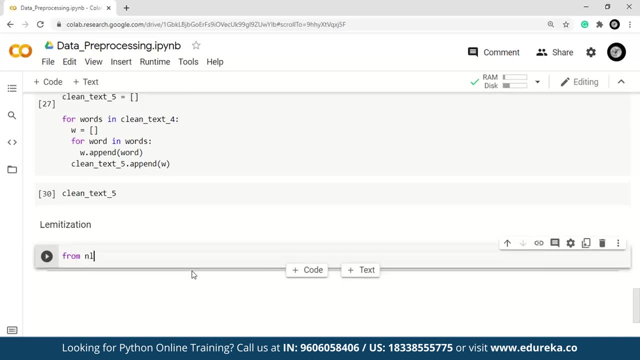 So let me just give limit ization here, Okay. So, in order to get this limit ization, we use something called as word net. Okay So, from NL, TK dot stem when there's a form of stemming, but it makes sure the word which 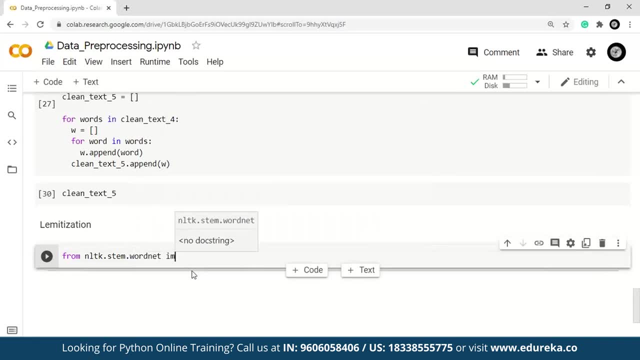 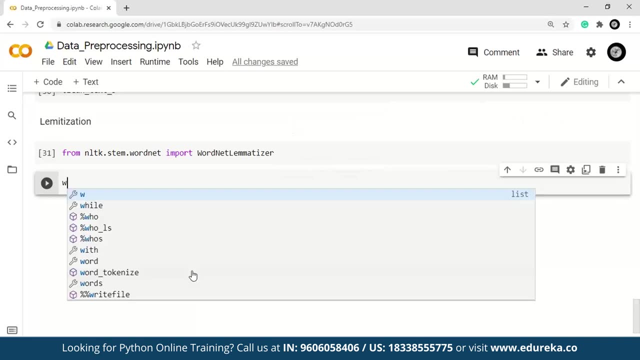 is being outputted has some sense. Okay, So import word net limit ization: okay, and we're going to create an instance of this. So it's going to be word net. or let's give word net w any T, It's going to be word net. 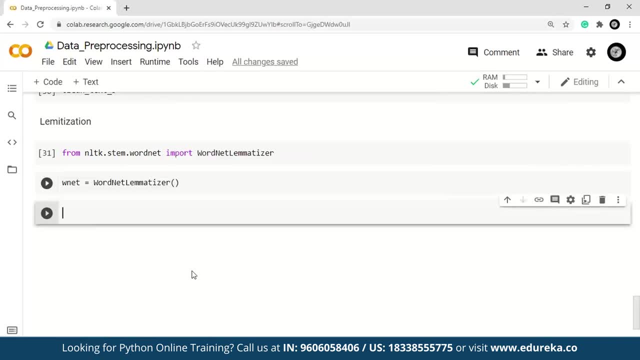 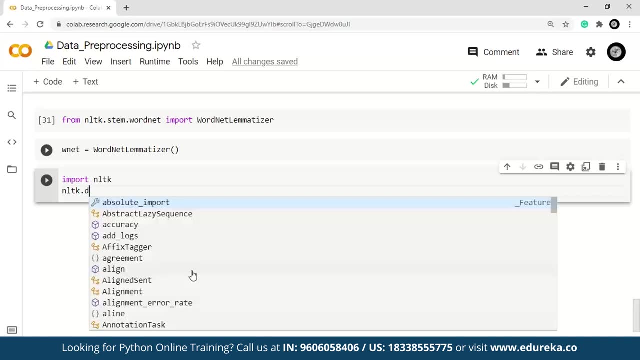 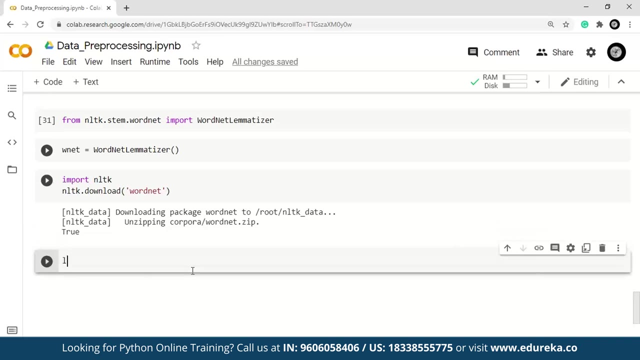 limit ization. Okay, and now we obviously have to download couple of packages. So import NL TK, and then we have NL TK dot, download word net, fine, perfect. So now, in the same way, what we're going to do is We'll create just limit ization words. 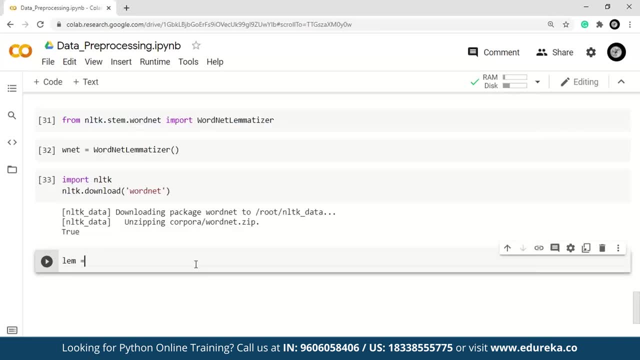 All right. so we have limit ization words here- L E, M, M, till be, L E M- and then we have an empty array and then we'll have a for loop for words in clean text, for it's not going to be five, Obviously. it's going to be a clean text for, because this is a form of stemming right and 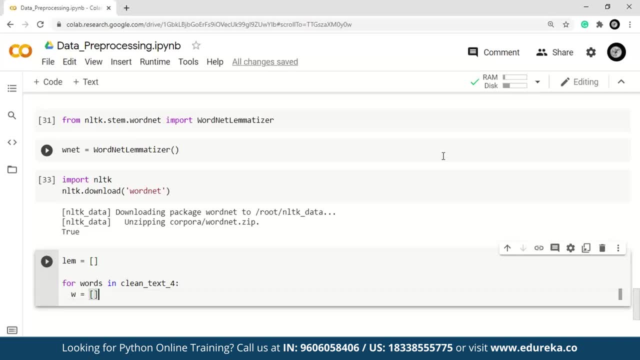 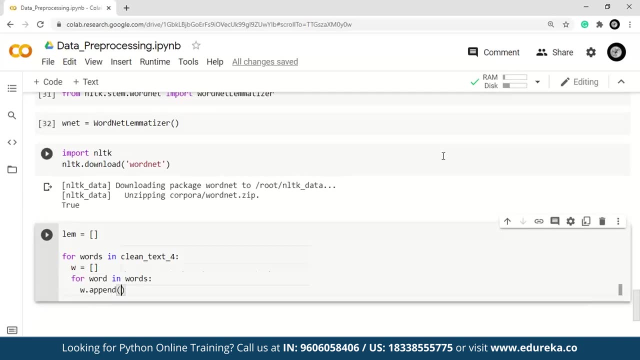 now what we're going to do is just the same drill. we have W, which would be an empty list, and another for loop, And we are going to up in whatever is there w dot up in the limit eyes words. Okay, so word net, not limit eyes, and whatever word we want to limit eyes. 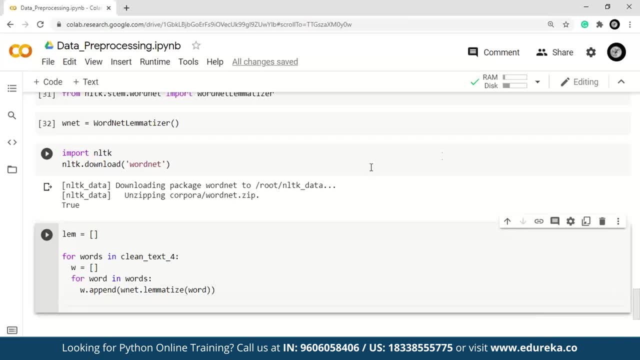 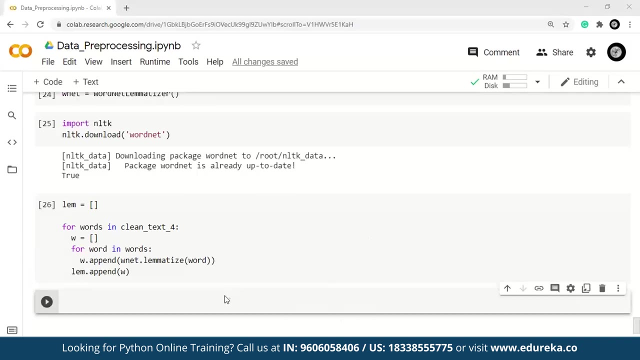 So it's going to be word here and now. once this is done, we're going to up in this w to our bigger lem L E M dot up in W and let me execute this Now that this is done. So let's see how this would look like. 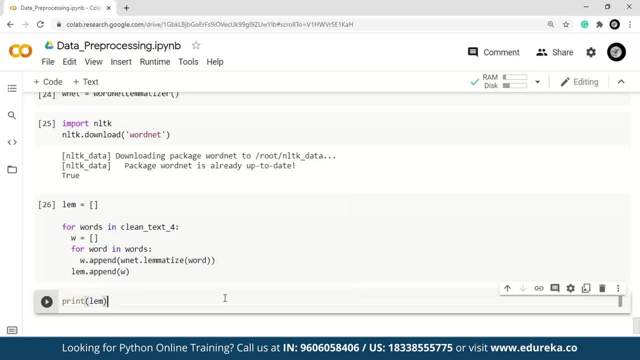 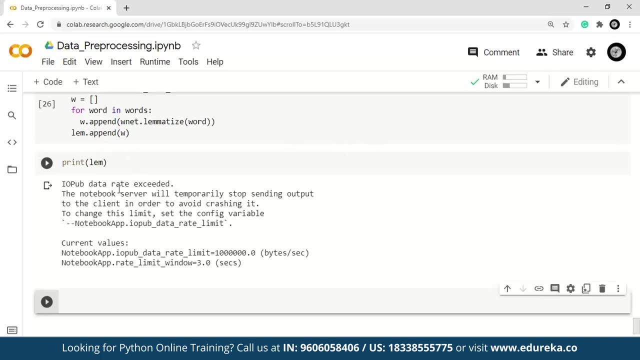 Okay. So, L E M, let's print this. Okay, and let me just execute this part here. Okay, we cannot print this, that's because it's saying data is too long. So, rather than printing, I'll just do this part here, L E M, so that we can just see some. 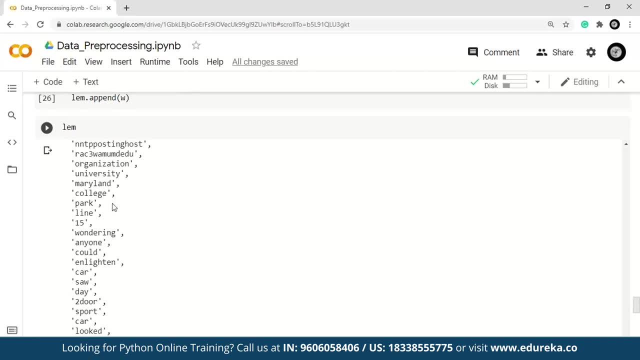 glimpse of how our data looks like. Okay, So, yeah, so, as you can see here, although we are performing limit ization, but now the words make sense- just to give you a brief insight. right, Let's compare Our data: look earlier and how it looks now. 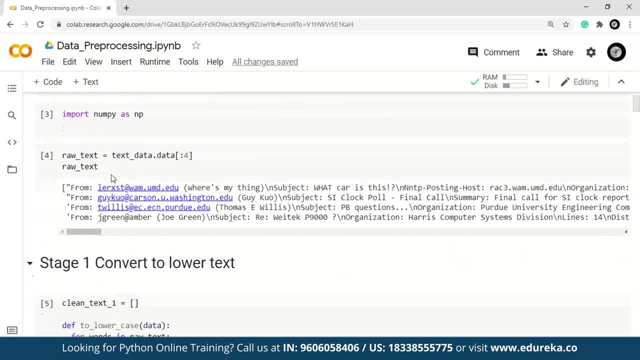 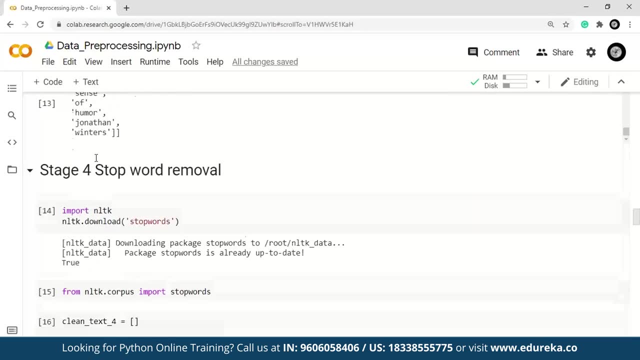 Okay, So what we'll do is we'll take our raw text, that is, this part here, and we'll compare this with our final text, which is nothing but clean text for right. That is after stemming. Sorry, it's going to be clean text five. 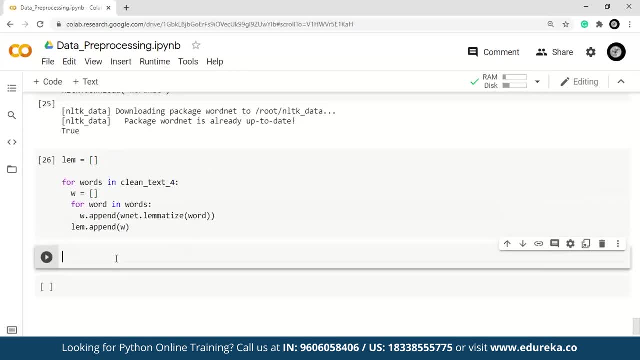 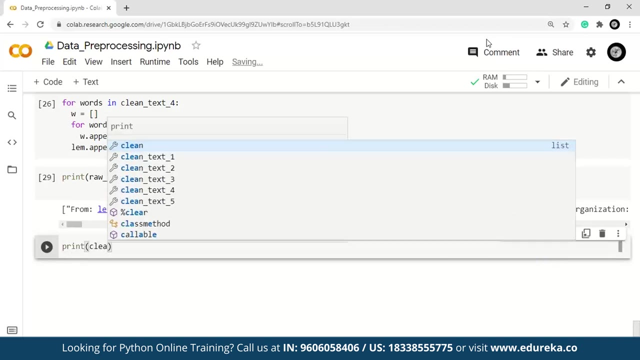 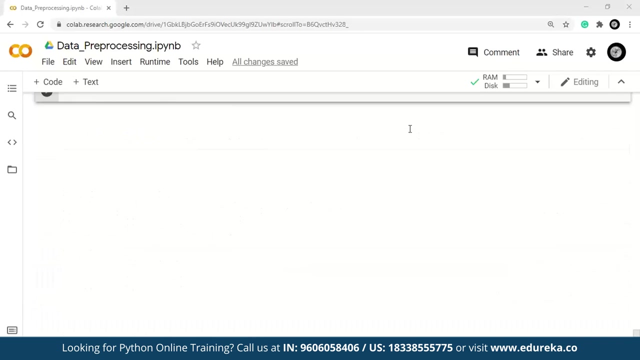 Okay, so let's now see how it would look like. So let me quickly print them. print Raw text. Okay, let me execute this first. All right, And now let me print clean text. 5 Okay, as the data is pretty huge. 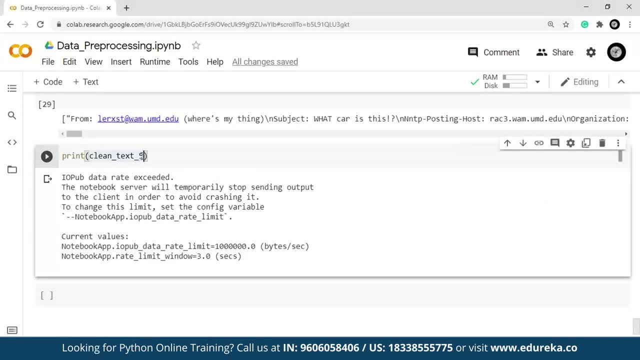 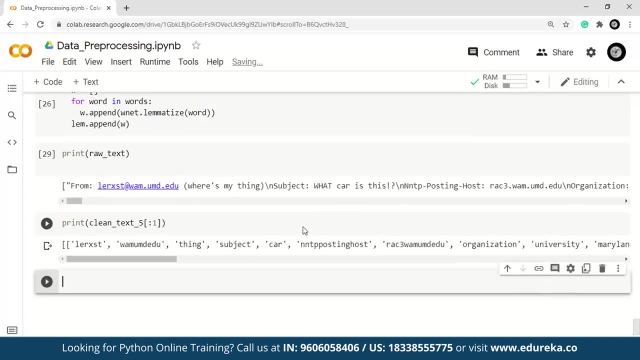 What I'm going to do is I'm just slice this up over here. Okay, Let me just take our first one data. Okay, this is going to be the first sentence and, as you can see, here we have all the words which have been tokenized, and it's unlike this part here. 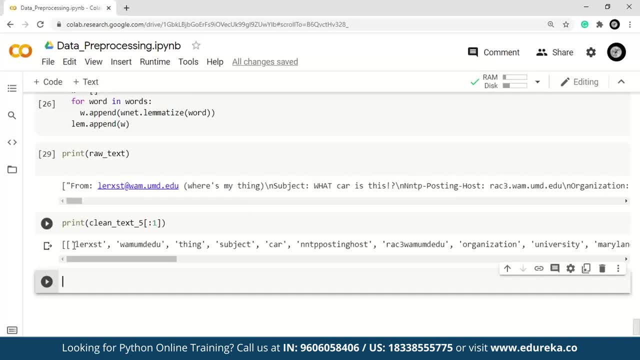 We have everything, which is it looks organized Okay. So obviously we want to pre-process this data right, because this makes more sense and it is more easy on a system to analyze and the classification would be pretty accurate as compared to what it would be over here. 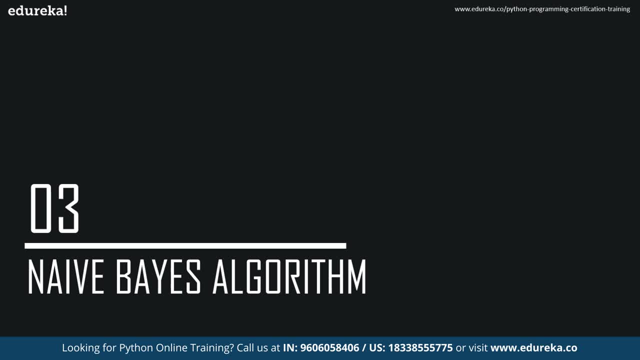 All right, now moving ahead. I hope now you understand why we need to pre-process our data. Okay, So now that we know how to pre-process our data using NLTK, Let's see how classification of text is done. So okay, in order to classify our text, we use something called as NIV bias allocation. 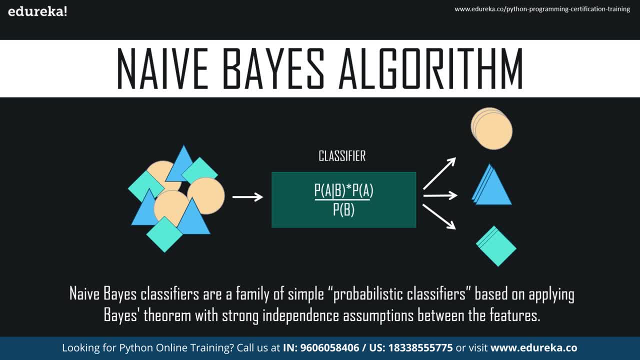 Algorithm. So what is this NIV bias algorithm? You see, before we understand this NIV bias algorithm, right, let us see what is classification. in simple words, classification means grouping of data based on common characteristics. as you see, here We have couple of figures, right? 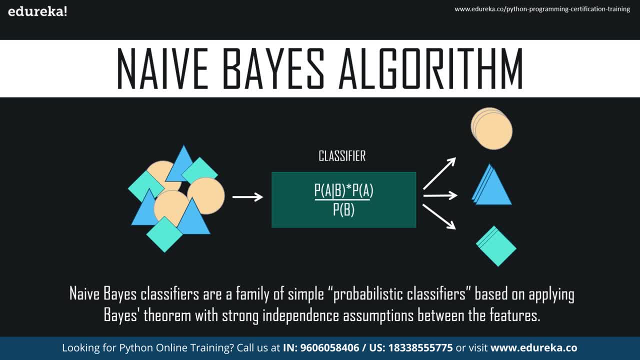 We have triangles, circles and a square and now when we pass this through a classification algorithm, all of those get categorized into different, different classes and it's totally based on the shape, size and whatever other features are. this is a similar way how the NIV bias algorithm works. 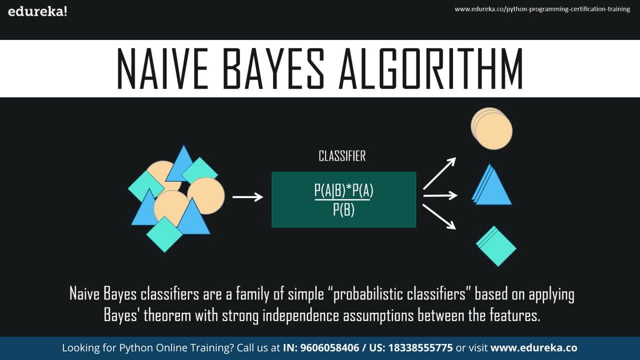 Okay, So the principle that drives NIV bias algorithm is something called as Bayes theorem, and we use Bayes theorem to calculate the conditional probability. So let us now see the match behind our conditional probability. All right, then. as I mentioned earlier, right, we use NIV bias algorithm to perform classification. 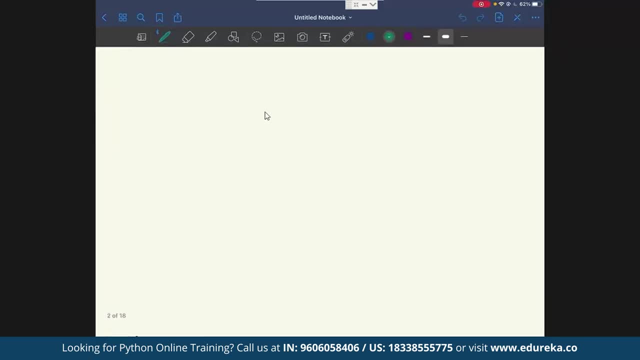 on our textual data and name base algorithm has something called as Bayes theorem. Okay, and the way this Bayes theorem works is that we have to find a conditional probability. So what is this conditional probability? you see, conditional probability- we can say mathematical, like probability of occurrence of event a when event B has already occurred is equal. 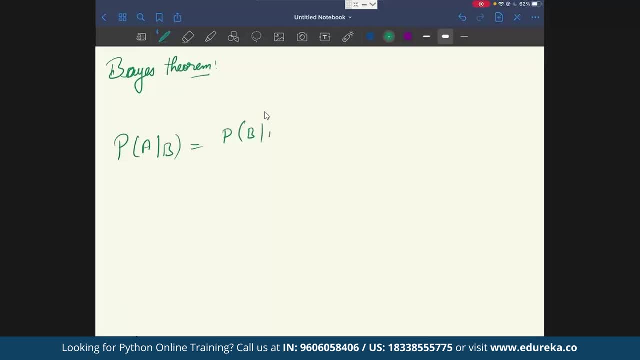 to probability of occurrence of event B when event A has already occurred: times, probability of occurrence of event A and this would be normalized by probability of event B. Okay, I'm sure you might be having confusion like: what is this right? you see this line over. 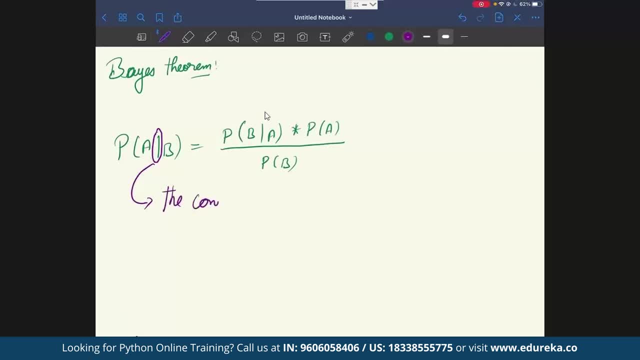 here. this represents the conditional probability. Okay, So this is the conditional probability. Now what we are going to do is: let's understand. what is this right? So probability of event a and B. So let us now take event a, to be like shopping. 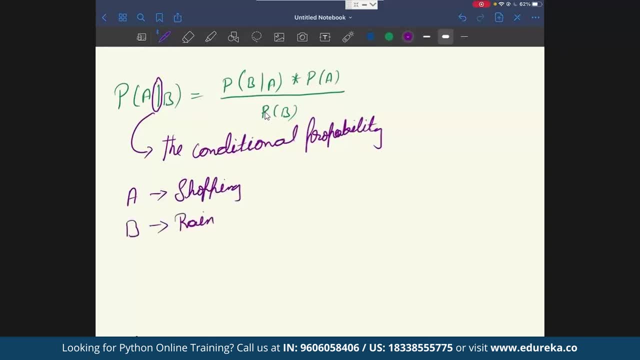 And event B would be something like rain. Okay, So what is the probability of you going to shopping when it has already started raining? So this is what this means. Okay, probability of a, B, right, So this represents and- and you can also say it as conditional probability. 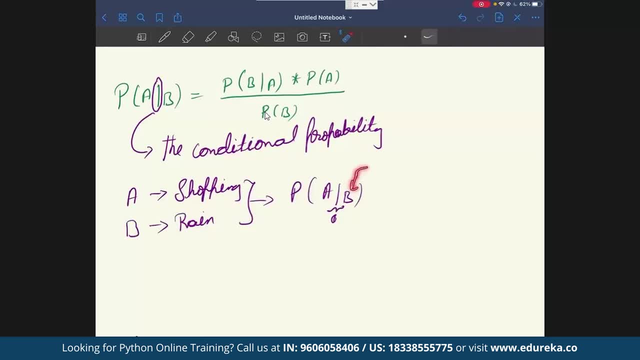 So probability of occurrence of event a When B has already occurred. okay, so when it's already raining, what is the probability that you'd be going down for shopping? and there are a couple of terminologies that you need to know when we are dealing with this. 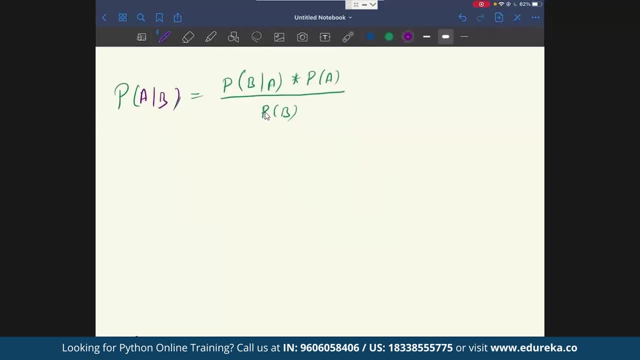 Let's quickly see that. Okay, So when we are dealing with conditional probabilities, we have a couple of terminologies, as I mentioned. So this part over here is referred to as posterior probability. Okay, this is the most important part to be found and is called as likelihood. 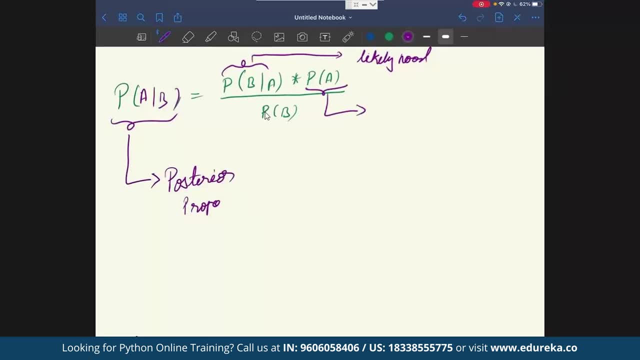 This part over here, The probability of occurrence of event a is called as prior probability. as you can see by the name right, prior refers to something that has already occurred. Okay, and this part over here is the most unused part. that is nothing but likelihood. 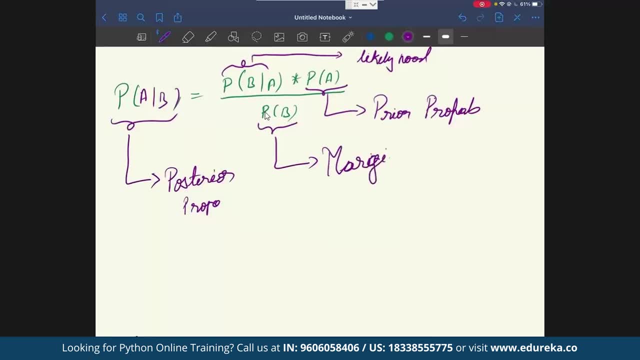 Okay, we call this as marginal likelihood. All right, so now, speaking about probability, let's see how this concept came into existence. So we have probability only because we have something called as random variables. Okay, this random variables give rise to a randomness. 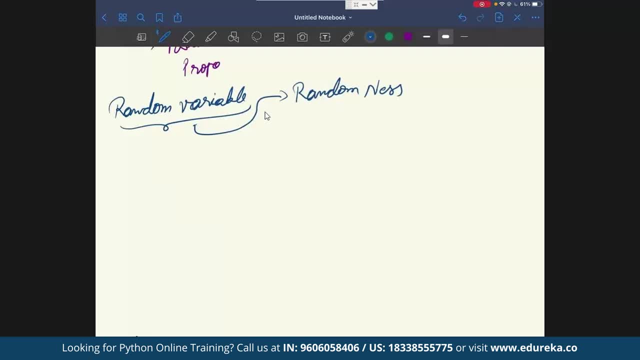 Okay. to give you a better understanding of what I'm trying to say, Let's take an example. Okay, So we have two bags here. We have, say, bag one, and let's say back to: okay, and now what is happening here is in bag one. 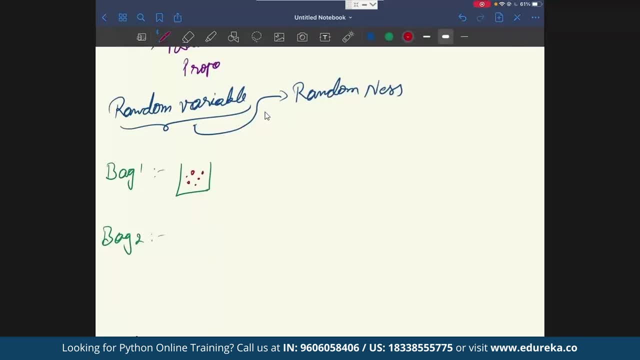 We have balls- Okay. We have red balls- five of them, Okay. So do you think probability exists over here? Obviously not, right? So no matter which of a ball you try to pick out, We're going to get red balls, And randomness over here is zero. 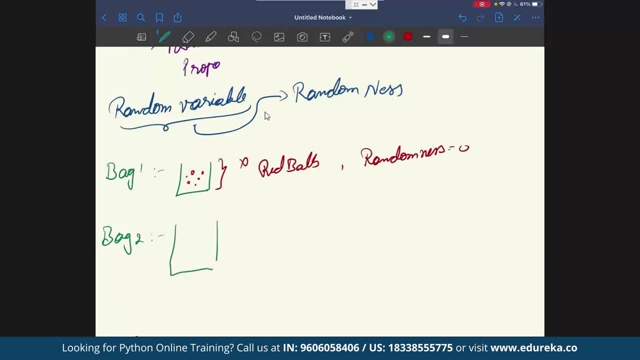 Okay, so let's take one more bag over here. So this bag has like five red balls and then four blue balls. So do you think probability exists over here? Absolutely. Oh yeah, you can see if I try to put down my hand and pick up any ball. 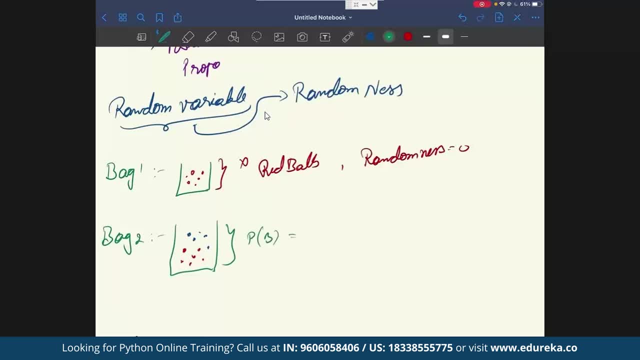 So probability of getting blue is nothing but the total number of elements, right? So we have like five balls and this, so it would be 9 divided by total number of blue balls. Nothing but four. Okay, So this is what is probability. 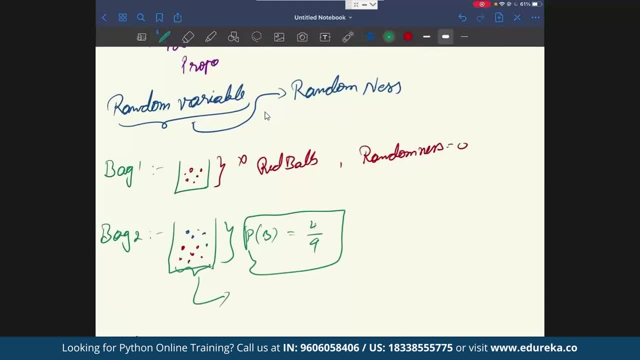 So over here we have more randomness. Okay, This is how probability came into existence. and, speaking about our conditional probability, Let's try to derive this conditional probability equation. Okay, So the way we get this conditional probability is by having P of a intersection B. Okay, 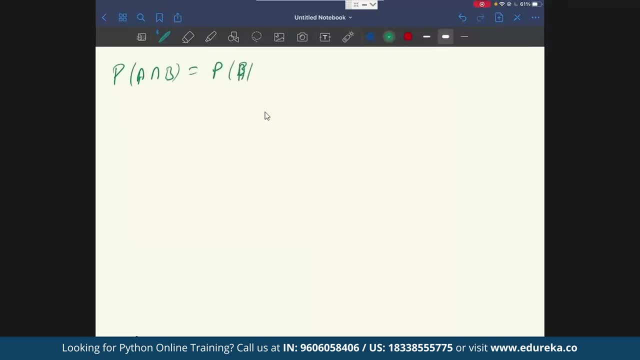 we all know this is equal to probability of a by B when B has already occurred. Okay, So this would be our equation one, Okay. Similarly, We know that it holds good for probability of B intersection a right. the reason for this is because P of a intersection B and P of B intersection is commutative. 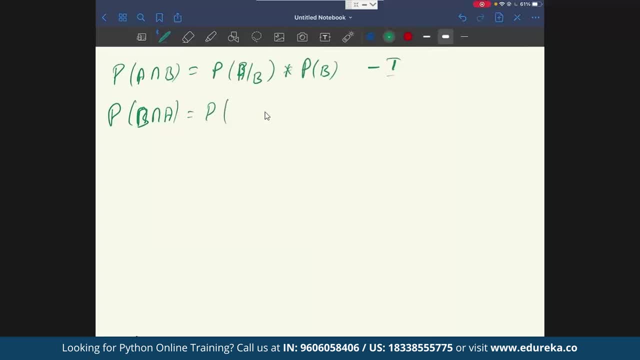 Okay, So this would be similar. only different that we are going to have is the change in the values. So instead of a, it's going to be B here, times P of a. okay, and now when we equate these two right, we are going to get something like probability of occurrence of event 8 when 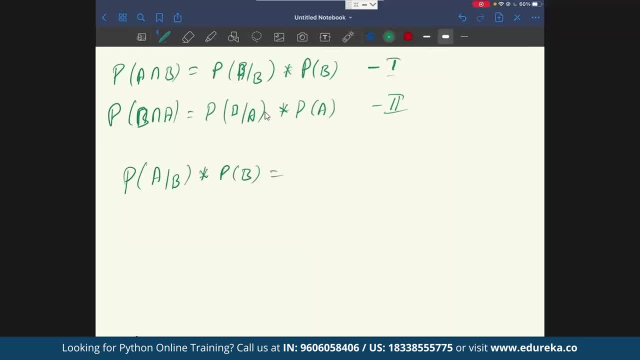 B has already occurred, Times probability of B, and this would be equal to this equation over here. All right, so let's bring this down, and then we'll have probability of occurrence of event a times probability of occurrence of a whole, divided by probability of occurrence of B. 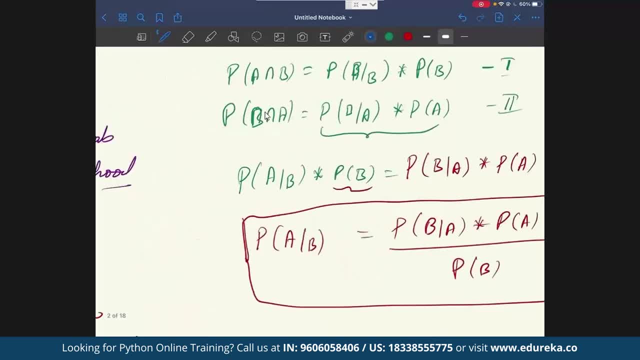 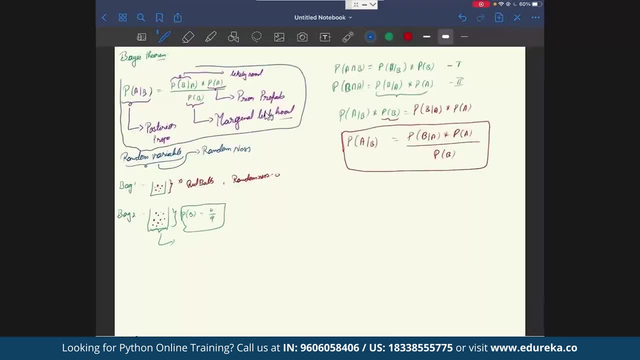 So this is called as base theorem and, if you see right, so this is something which is very much similar to what we had over here. Okay, So this is what is base theorem and this is how we derive it. So now you might be wondering: how can I use this base theorem for classification problems? 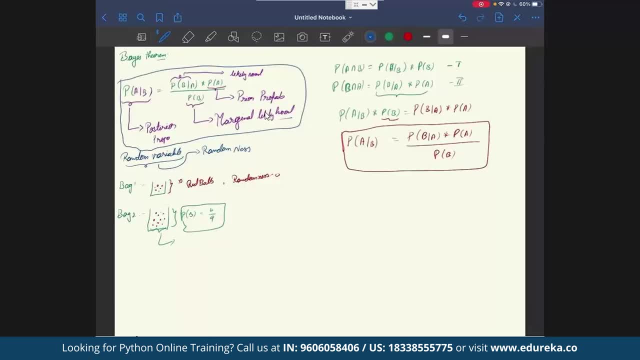 right. So just a quick recap. as I mentioned earlier, classification is nothing, but you know, categorizing a data based on its characteristics, Okay. So here, what's going to happen? here will have something like you say: we'll have a data set, right, So let's take X, so we'll have X data set. 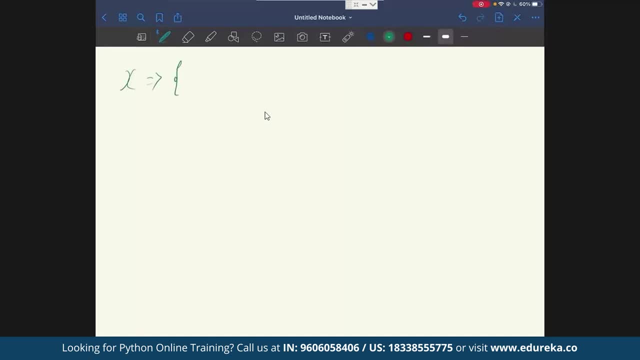 So this would be nothing but group of values- Okay, the text data, and then we'll have Y. Y is nothing but the classes, and Y refers to the classes And what this class means is. it can be like 0, 1 and so on and so forth. 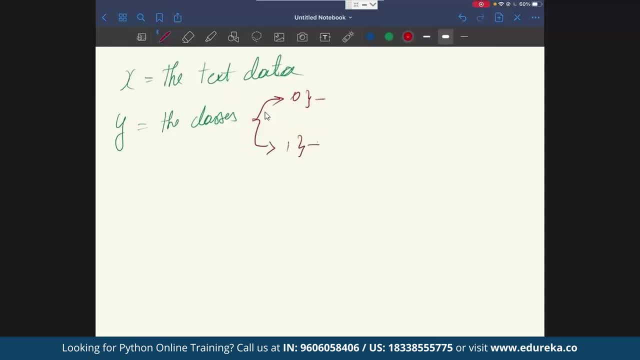 So here let's take something like 0 and 1, and here 0 refers to in being it not spam, And this is spam, and here X would be nothing but group of emails. Okay, So now let's put this in a base theorem and see how it would look like. 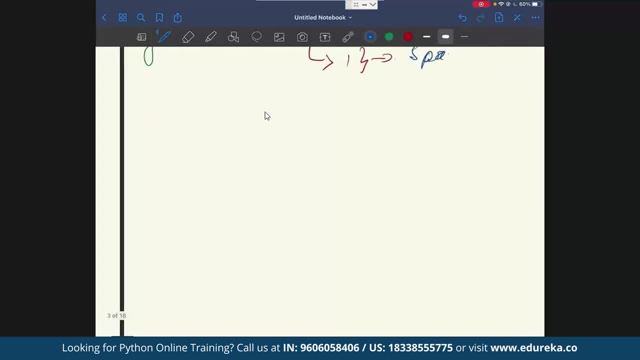 All right, So over here we have for base theorem will have something like probability that an email is spam. Okay, when we already have the email is nothing but probability of this particular email being in spam class times. probability of that email all divided by P of X. 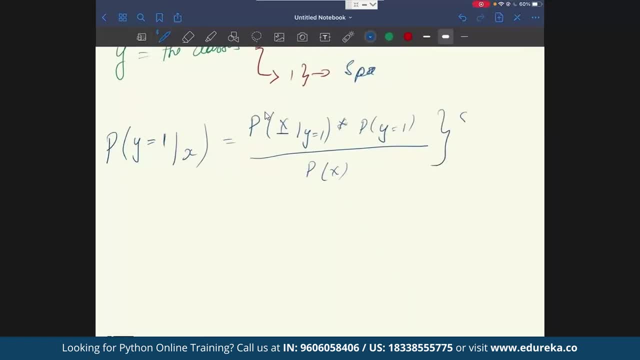 Okay, and similarly, this is for spam email and now for not spam. It would be: P of Y is equal to 0.. Okay, given X, this would be nothing, but given that we have a label of non-spam, and then what is the probability of that email being here? 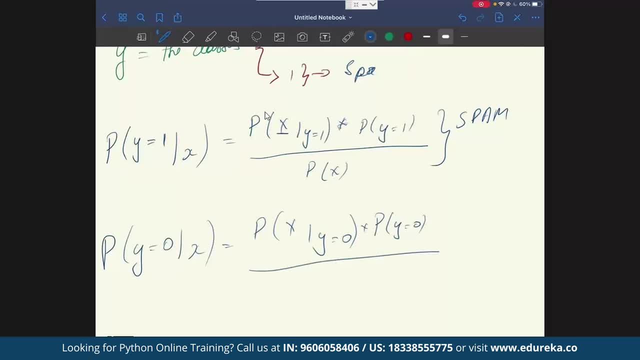 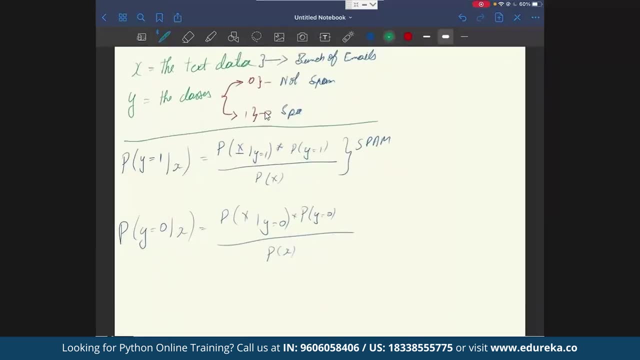 This would be times. probability of Y is equal to 0 all divided by P of X. Okay, So this is how it would look like you know base theorem for finding whether the email is spam or not. So to better understand this right, 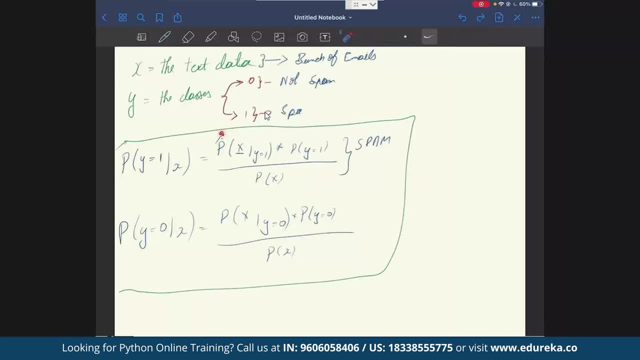 Let's see what each of this represents, Okay, Okay, So let's take this part here. I'm pretty sure you must be confused what this part represents, right? So what this part says is: thing that we have a data set, Okay. 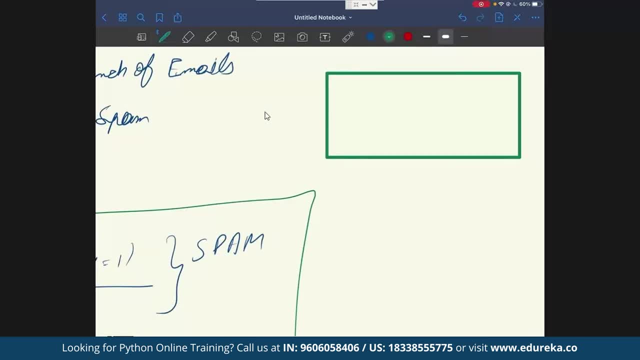 So that's this, This be our data set. Okay, So this is our data set, and we have X values here and then we have Y values. what this X values will have is nothing but emails. Okay, So this is nothing but group of emails and this would be a class. 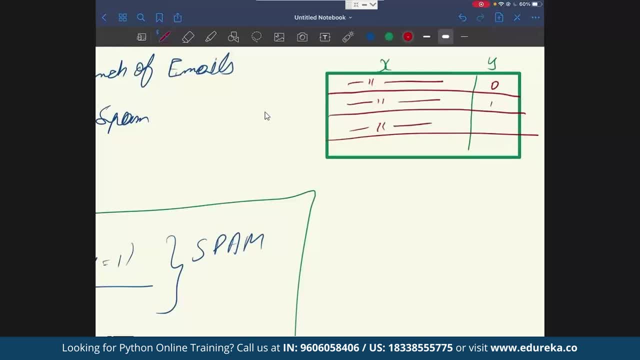 So if the email is spam, it would be 0, for email is not spam, It would be 1, and then 1 and 0, so on and so forth. Let's just take it as an example, and this is something which is an unknown value, right? 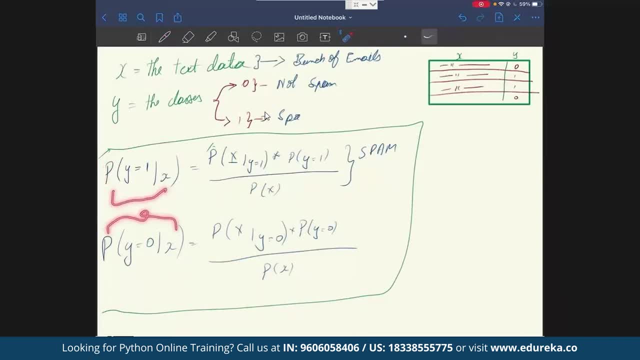 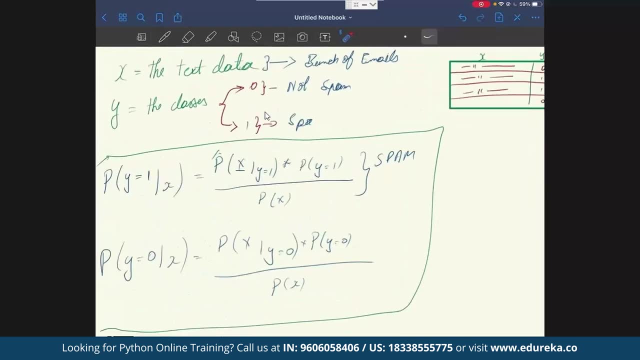 So this part over here is an unknown see. both of these are same. Okay, So, as of now, let's just consider for a spam email. Okay, so we need to find a new email. Okay, so we'll be given like we'll have a test. 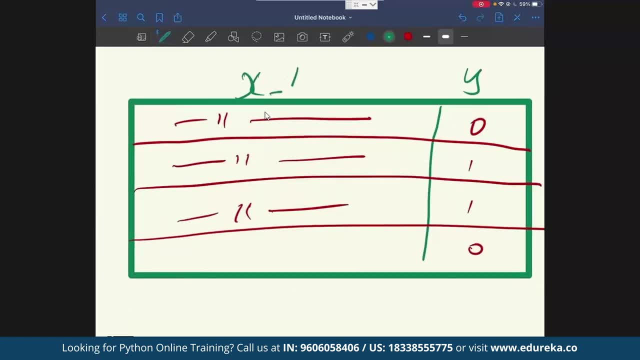 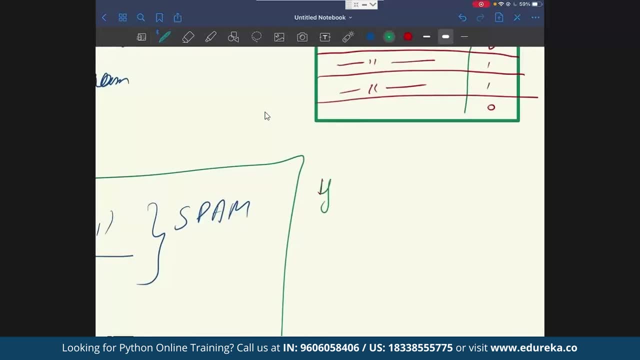 So let's call this as a train data, right? So X train, Okay, and this is the output, is a class. So now what will happen is I'll be given a email, So I'll be like Jeanette, find out whether this email that I'm giving you is a spam, or 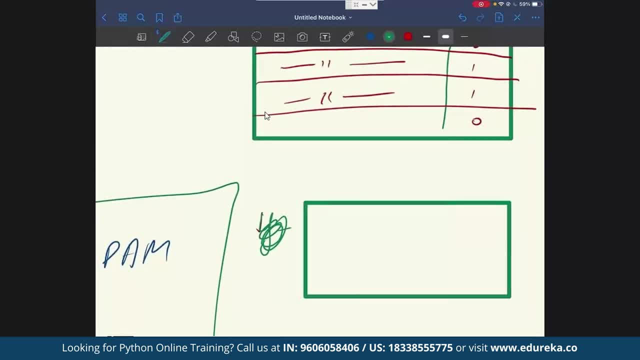 not spam. So this is going to be like this, Okay, and then there will be X test, but only difference is here: We don't know which class they belong to. Okay, So what we're supposed to do here is we are supposed to train our model and figure out. 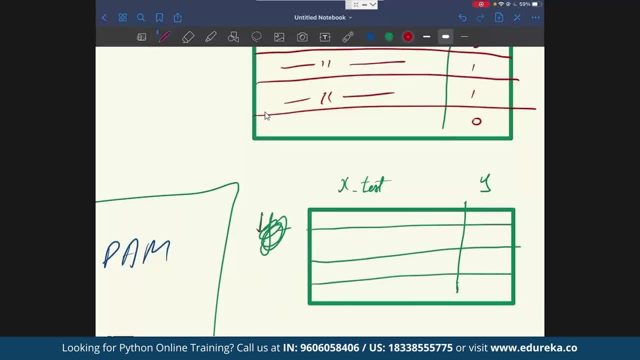 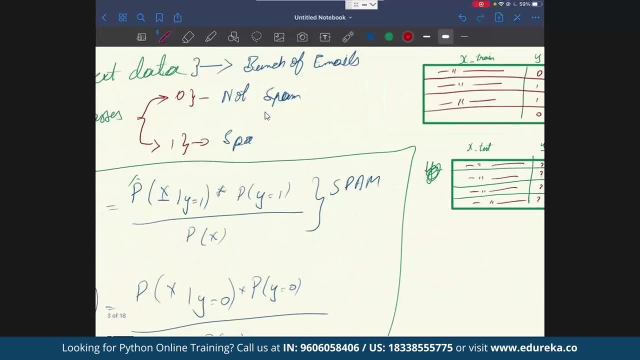 which class this email would belong to. Okay, So this is an email here. These are the question marks. Okay, We don't know what class does this email belong to. So what this P of X and Y is equal to 1 represents is when we are given a class wine. 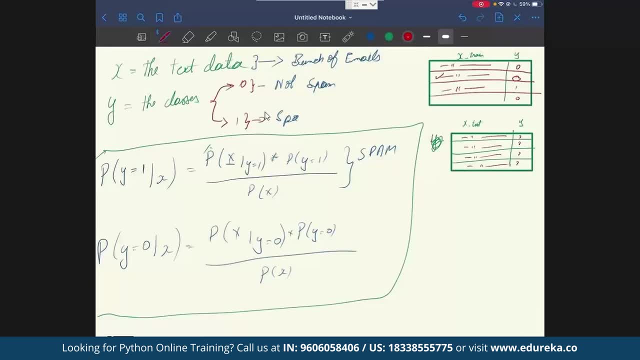 Okay, when we already know that email is spam, that is, this particular email. What is the probability of this email part of being this? okay, and then we compute this part over here And then, finally, what we are going to do is, when we get this test data right- X test- 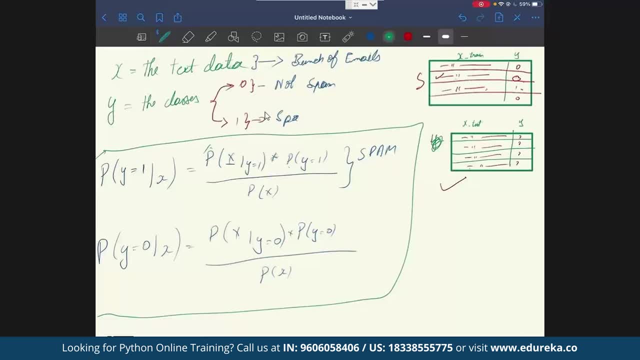 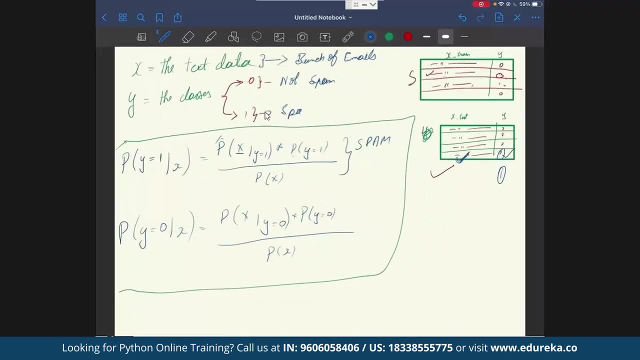 data. We'll just say what is the probability of this particular email being a part of 0.. Okay, 0 means not spam and 1 means is a spam, So we'll basically get a digital value over here. So, for example- now let's take an example over here- 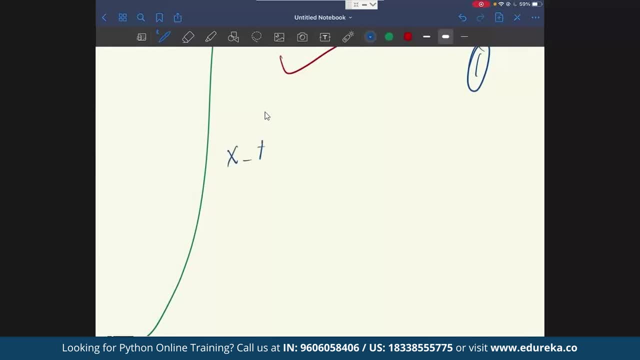 So I got this X test value. X test is something which will be over here, So I got this X test value. say something like free food. So now this would be represented in spam, right? The reason is because spam is a keyword which is usually found in a fake email. 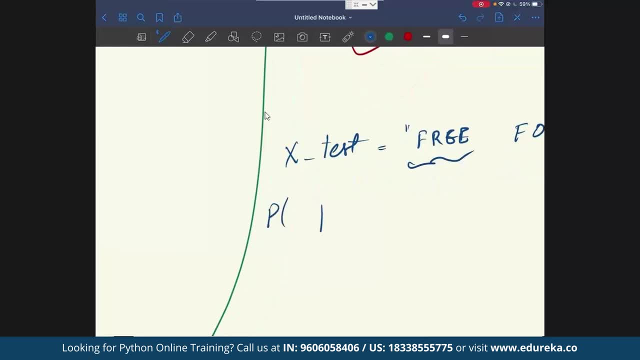 So what will happen over here? So probability that a given email that is X test is spam. Okay. so probability that given email over here- So this email, that is, this email- is not spam and is spam, So this would say something like this- will have a high probability of being in a spam. 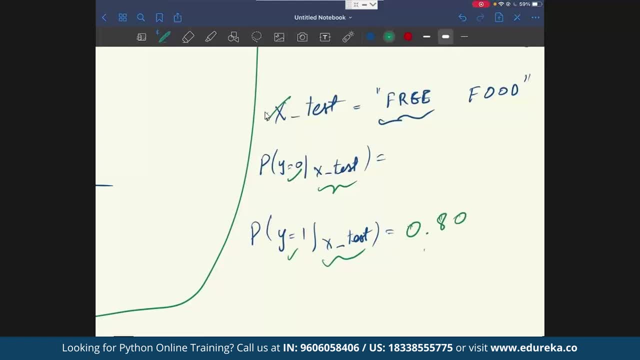 right. So this would give us a numerical value, say something like 80, which refers to 80%, and this would give us, like, say, 20.. Okay, and this is nothing but 20%. so which among this is high? So obviously this particular value is high, right. 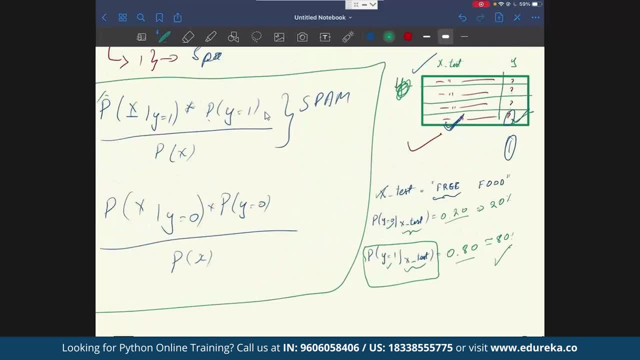 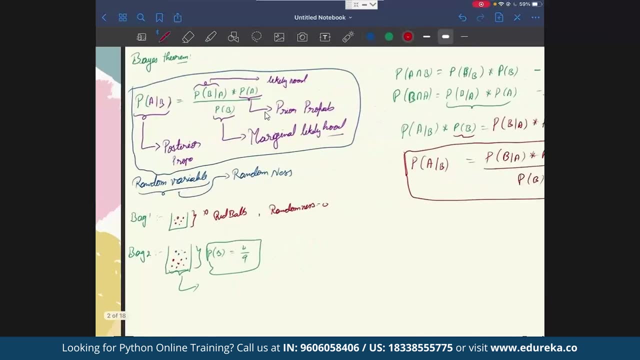 Therefore, this email would be classified as a spam email. So this is how, basically, it works. Okay, So now, in order to find this values over here- you know that that is nothing- but in order to find the value of our posterior probability, we have to calculate likelihood- prior probability. 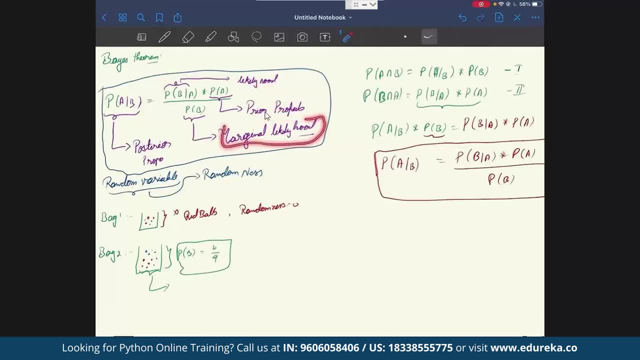 and marginal likelihood. Although we can ignore This, is because we are trying to normalize it, so we can ignore this part. finding the probability of this is pretty simple, because all we need to do is find the total number of spam email, but total number of emails, and similarly I would do it for total number of. 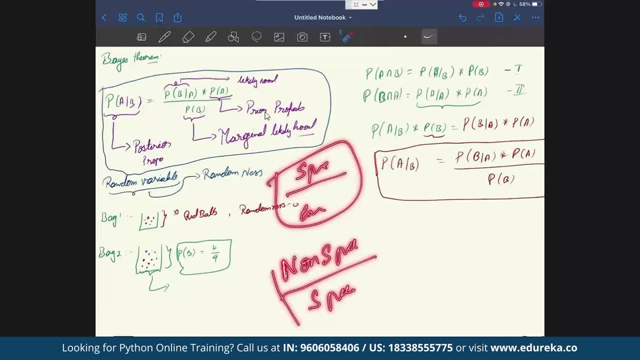 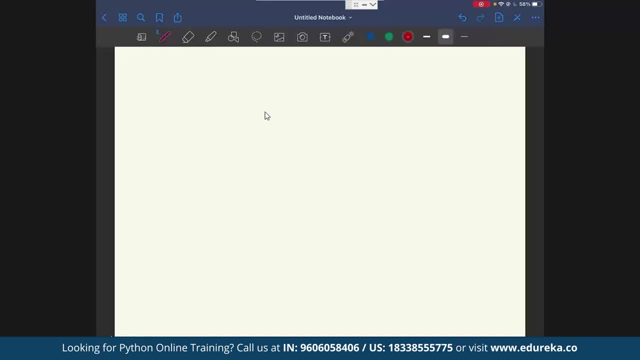 non-spam, but total number of spam. but the only difficult part over here to find is likelihood. So let's now see how we can do that. So to start off, let's say something like we are given some emails. Okay, so we have hundred emails out of this, hundred emails. 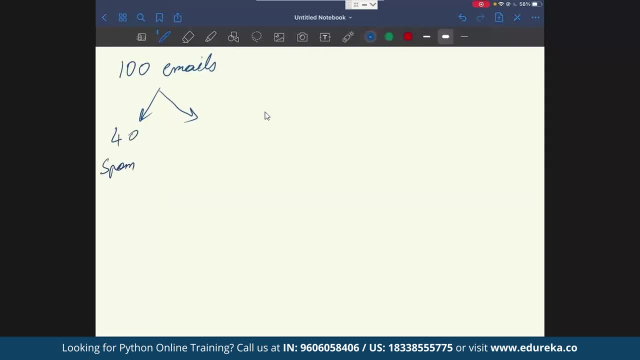 We have, 40 of them are spam. We know that these are the hundred emails and 40 of them are spam and 60 of them are not spam, and this, not spam, is represented by 0 and spam is represented by 1. that is nothing but Y. 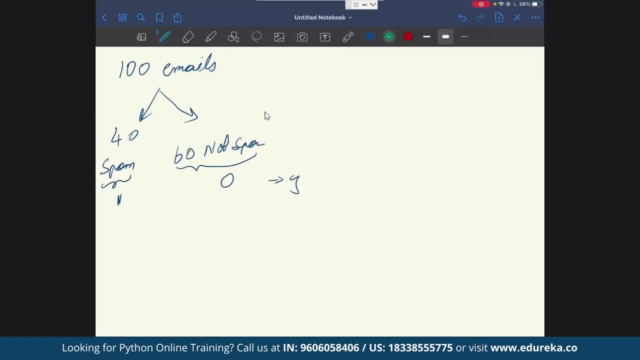 Okay, Y is equal to 0 or 1.. So how this would look like is: let's say, we have a table here and out of this table We'll have, say, X test, which is nothing but the hundred emails. Okay, so we'll have from 0, 1, 2, dot, dot, dot, and this would end up till hundred. and now 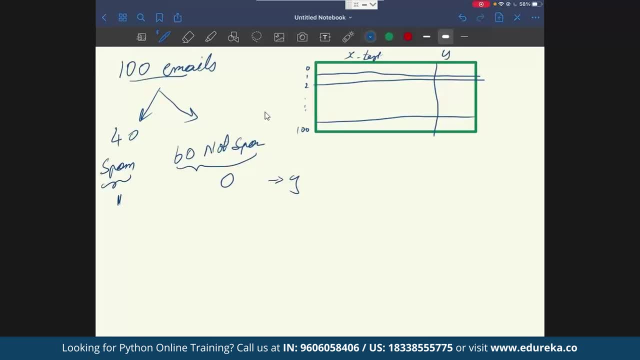 at the same time We'll also have Y. Y is nothing but a class, and these emails over here can belong to either 0, 1, 0, 1 or anything, but it should be either 0 or 1, and here it's going to be 0 or 1.. 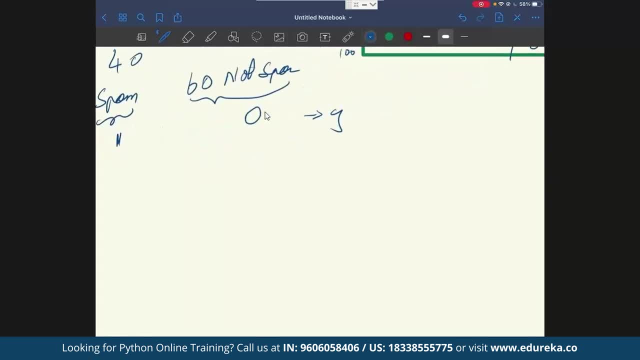 It's just that we're taking an assumption. So now what we're going to do is we'll be calculating our prior probability. So if this is our data set, our prior probability is going to be nothing, but P of Y is equal to 1.. 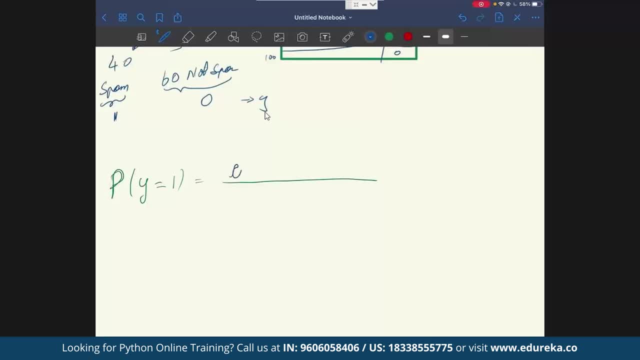 So what this means is: count all the spam emails. Okay, count all spam emails, But total number of emails: Okay, so let's now see what would be the probability for this. So what is the total number of emails? It's hundred, right? 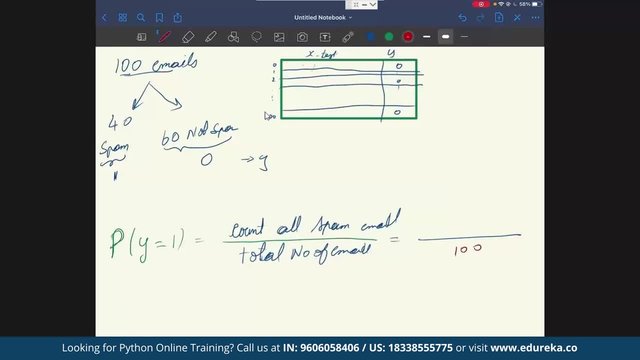 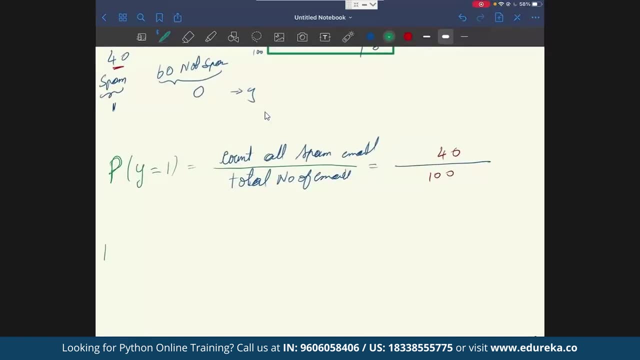 So it's going to be hundred over here. And what are the total number of spam emails? It's 40.. So let's quickly write 40 over here. Similarly, We are going to do this for P of Y is equal to 0.. 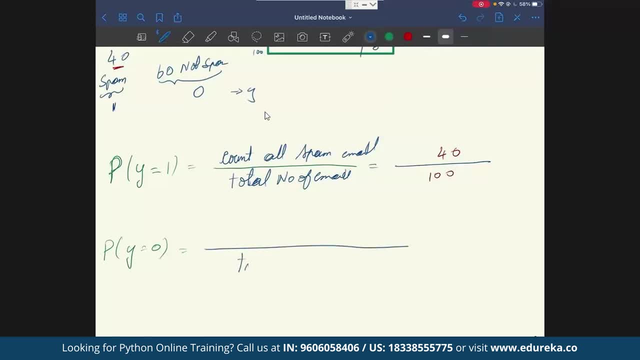 Okay, here is going to be total number of emails, and here we're going to write all the number of non-spam emails. So what would this give us? This would be hundred, which is the total number of emails, and then we'll have 60.. 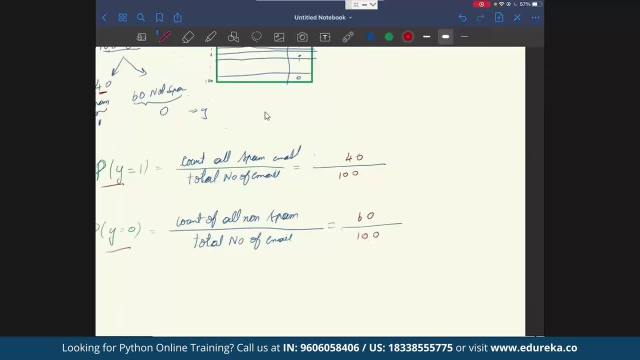 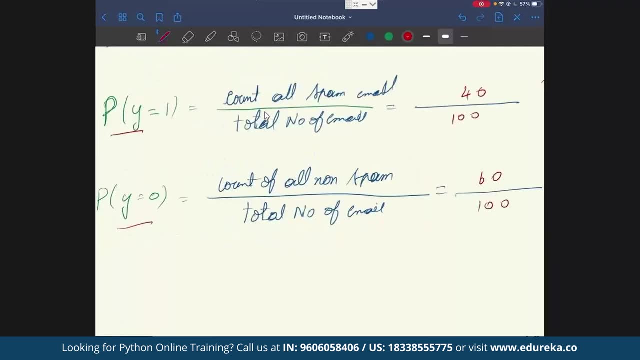 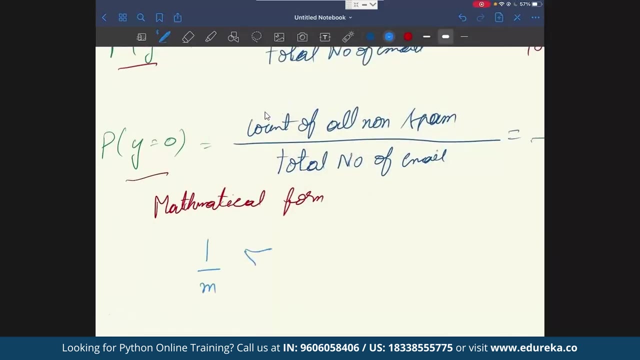 So this is how this particular part would look like, in order to give this in a mathematical form, because you know we obviously will be putting this in the form of formula right. So in the mathematical form. so this is nothing but an average that is 1 by M. summation of. 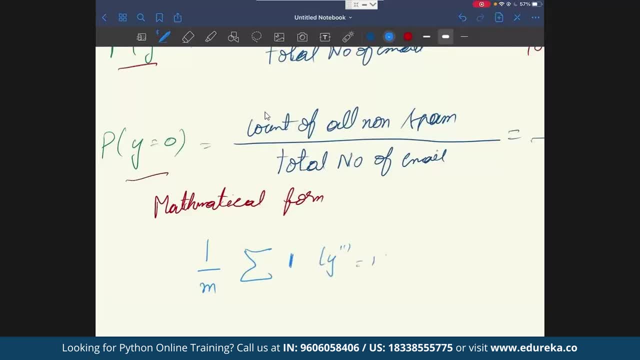 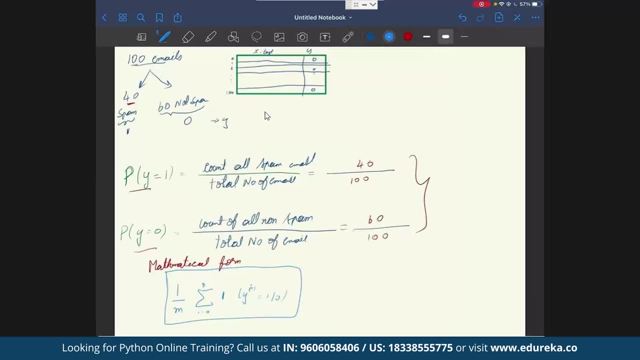 all the ones, for Y is equal to 1.. Y is equal to 1 or 0, and here this I will range from 0 to N. So basically we're trying to add 1, 1, 1 over here. Okay, So this is how we calculate our prior probability and, as I've mentioned earlier, we don't have 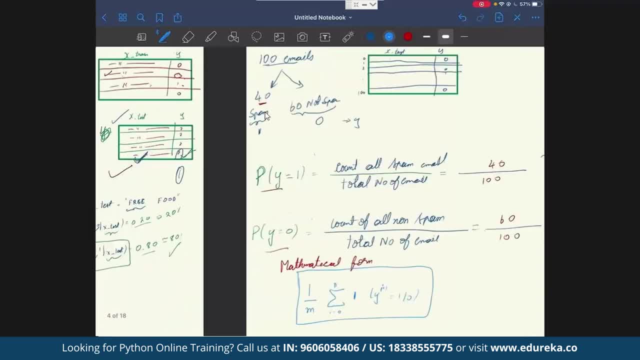 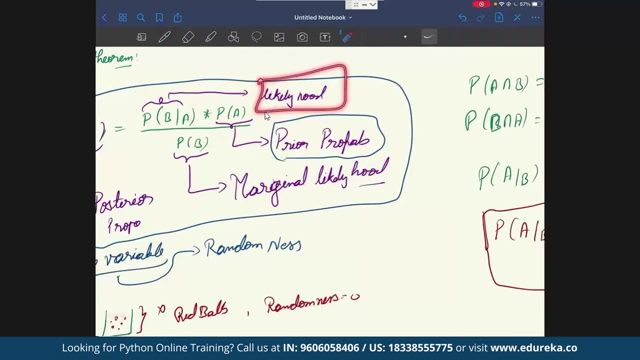 to calculate our marginal likelihood and finally, we are coming down to important stuff. That is the likelihood. Okay, So this is the part, This is the likelihood, which is the most important part and the toughest part to calculate. all this pretty simple. You have to understand the match behind it. 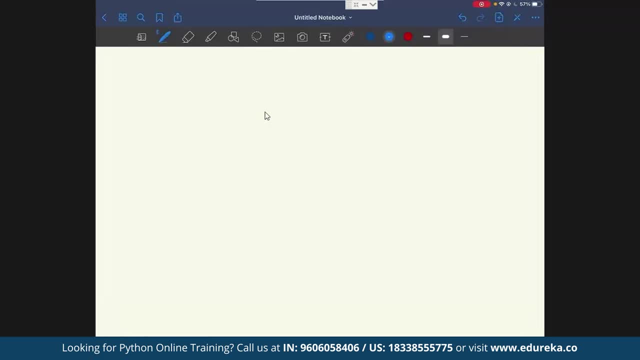 So, in order to calculate our likelihood, What we're going to do is we're going to calculate the probability, right. So let's see how we can do that. So we have this P of X when Y is equal to 1.. Okay, what this means is when we have this email, right? 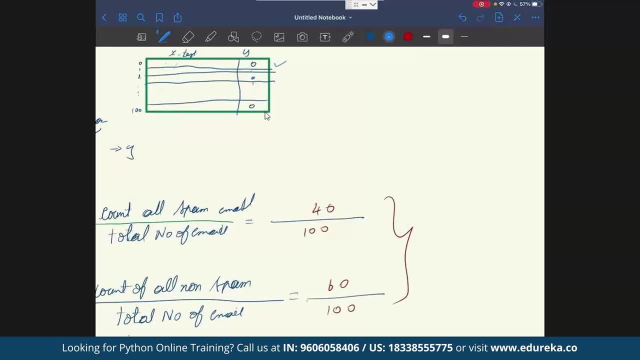 So we already know that email belongs to spam. We already know that email belongs to non-spam, So what is the probability of that email belonging to this particular group? This is nothing but probability that email belongs to class 1.. So probability that email belongs to class 0, fine. 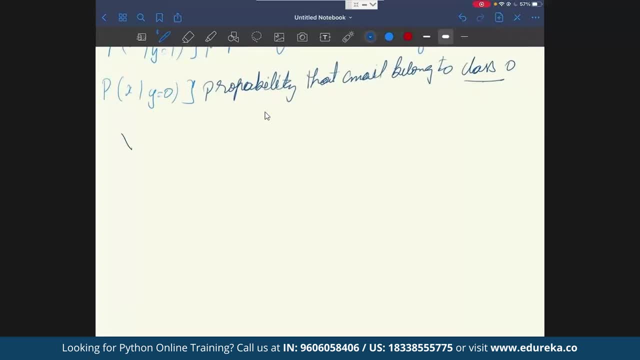 So now how X would look like. so just to give you a brief before we move ahead: X over here would be nothing but a email, So it will have multiple words and somewhere over here in the middle to be like get unlimited 50% off and so on and many other words. 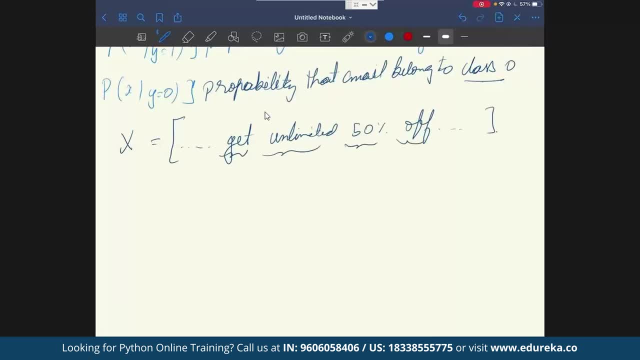 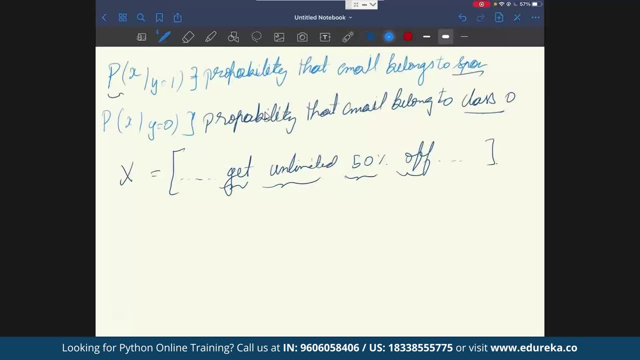 These are called the features and based on these features, We calculate whether this email belongs to a spam class or non-spam class. So how this would work, how this probability over here works, It'll take each of this feature. Let's take something like ultimate. 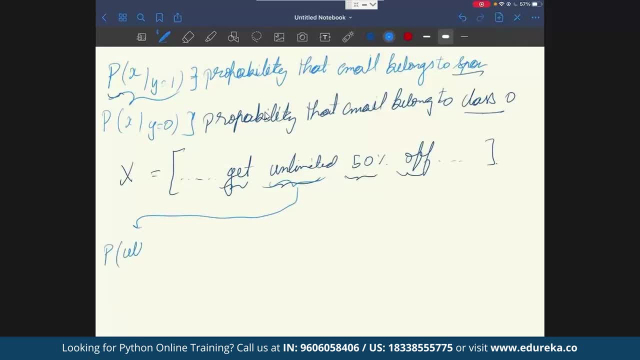 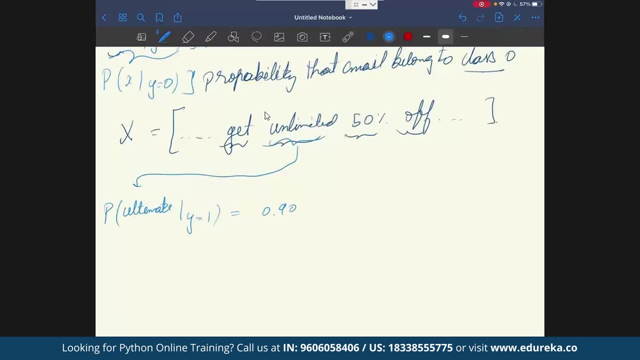 Okay, so it's going to be like probability of ultimate Belonging to spam. This would give me some value, say 0.9%, because it's high probability, right, that an ultimate word comes in a spam email, and then we'll also calculate at the same time probability. 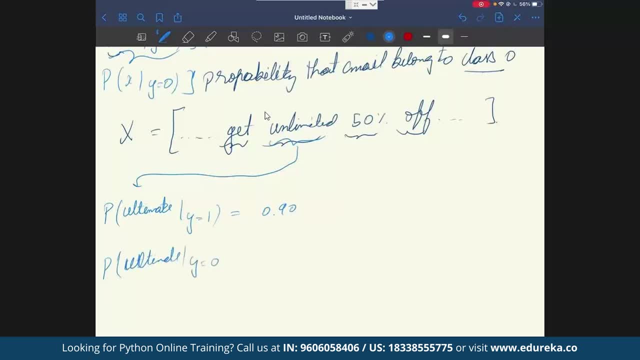 that ultimate belongs to non-spam, So this is going to be less probability. You obviously don't know, You obviously are not going to use ultimate in your day-to-day activities, right, or day-to-day conversation. So this is how it's going to be. 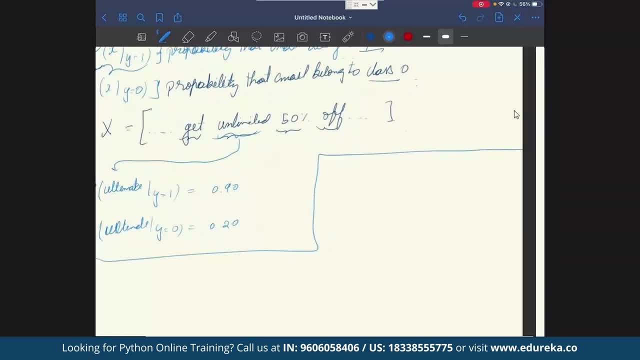 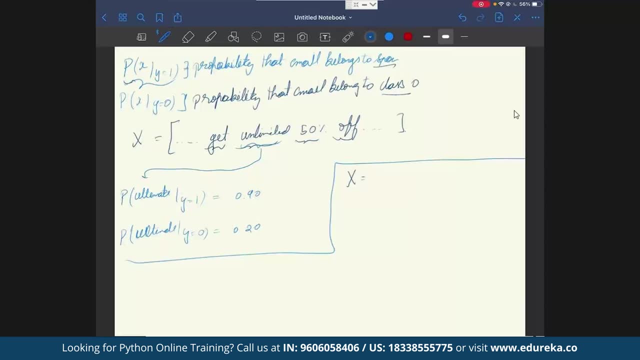 So let's now quickly see how we can calculate for this. So now we have X right. So if X, this is a capital, X is nothing but list of words, Okay. and this is nothing but an email, Okay. and then small x represents the words which are there. 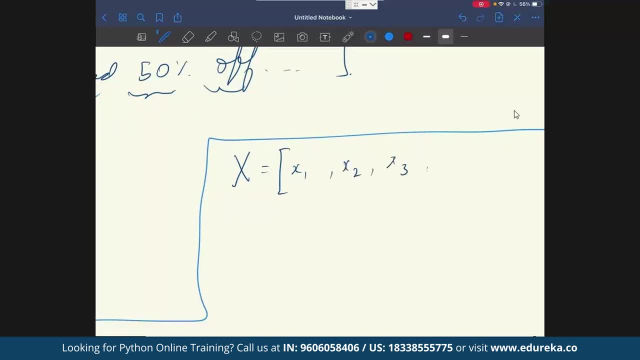 So here can be x 1, x 2, x 3, x 4, and this would end up to X- n. So these are nothing but features or words. Okay, and X is the entire email. Then what we're going to do- find over here is probability- that X, nothing but the capital. 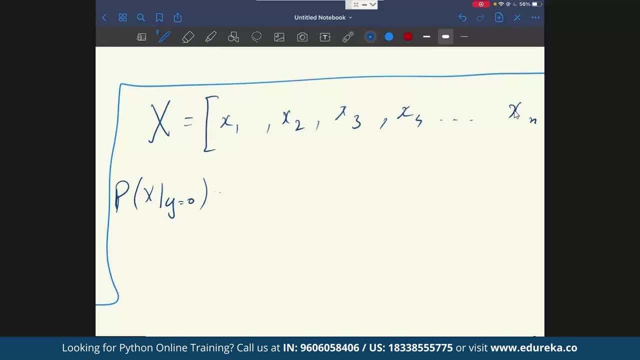 X belonging to y is equal to 0, is equal to probability of all of these individual words over here. So probability of all of these words belonging to a spam, and similarly we can do this for spam. So when we have an entire email, What is the probability that all of the words are the content of that email belonging to? 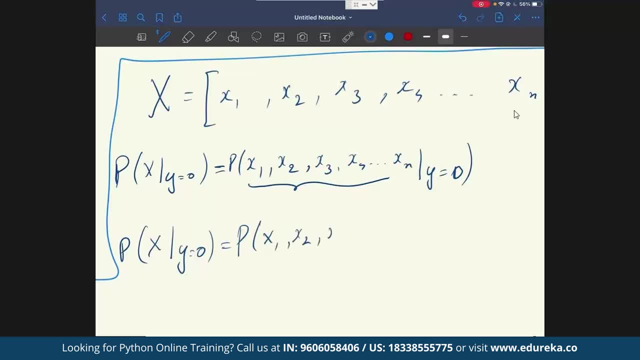 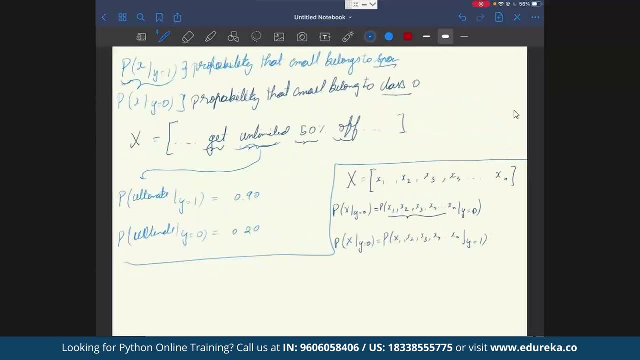 spam. So here we'll have x, 1, x 2, x, 3 x 4, so on. y is equal to 1.. So this is how it works. Let's see the expanded version of this. Fine, Let me copy this entire equation here. 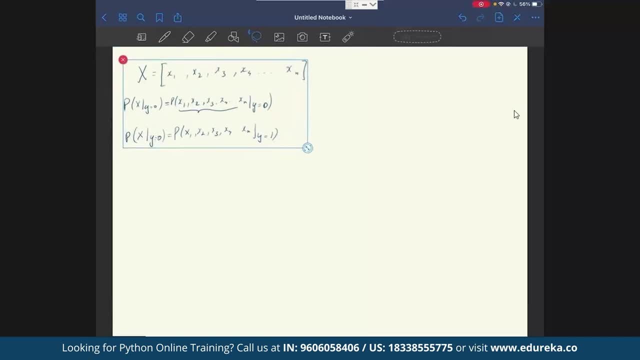 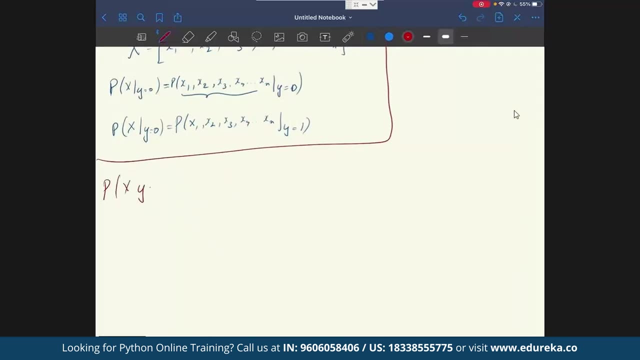 Okay, and let's paste it on a new sheet and let's see how we can calculate each of these right. So what's going to happen now? Probability P of X That Y is equal to, 1 is equal to. I'm just expanding this part over here. 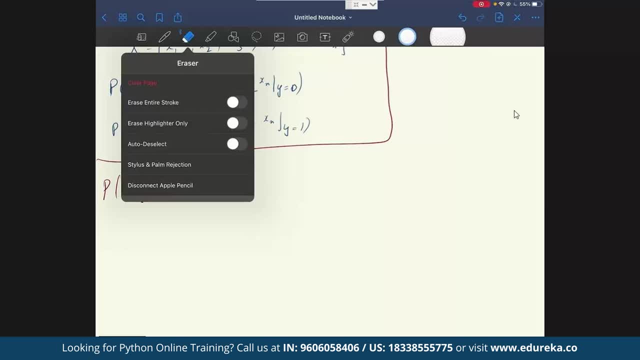 Okay, let me just erase this to give you a better insight. All I'm trying to do is I'm trying to expand this part P of X, 1 comma, X 2 comma, X 3, right, So this is nothing but probability. You see, this comma here represents and okay, it's an and operator. 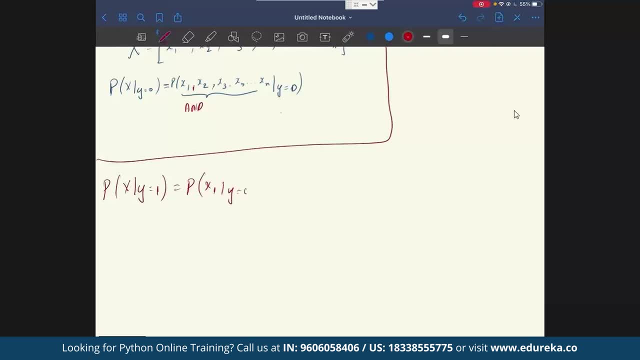 So probability of X 1 belonging to Y is equal to 0, multiplied by probability of X 2 when Y is equal to 0, that X 1 is also not spam. So this is how it works. This represents and, and then we'll perform multiplication, and then we'll do something. 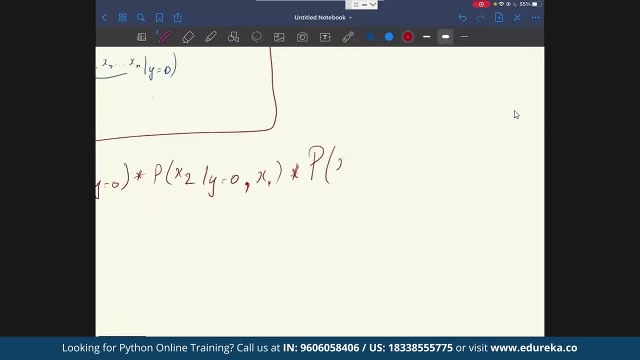 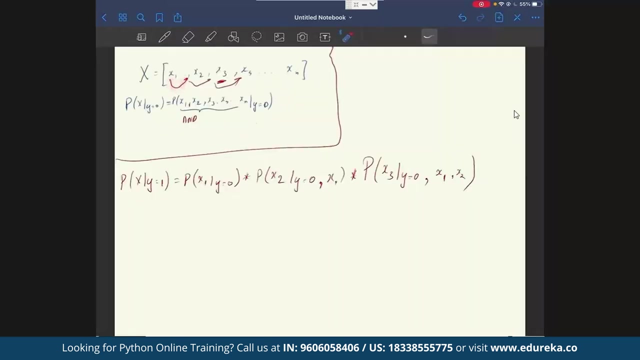 like this again. So for P 3 probability that X 3- that is nothing but the word. this X 3 belongs to non-spam category, when we already know that X 1 and X 2 also belong to non-spam category. What I'm trying to say over here is: each of these words are dependent upon each of these. 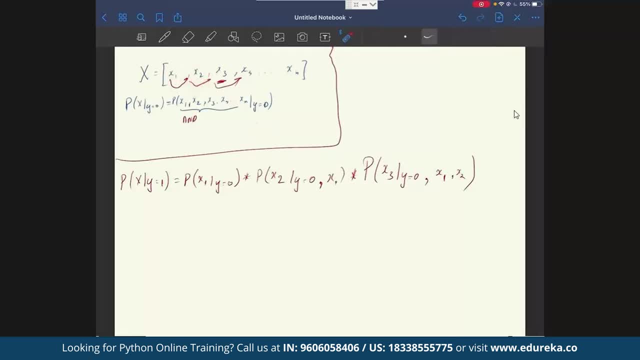 other. only if X 2 is considered as not spam, only if X 1 is not spam. you know, all of these words are dependent on each other and the probability of them is holds true only if the other one holds true. So what's the issue with this is, by the time it reaches this X and right, it becomes pretty. 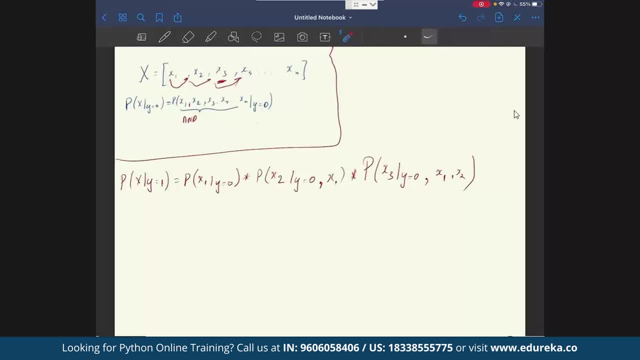 huge value and it becomes competition Very expensive. in order to overcome this, we use something called as naive bias assumption. and what this naive bias assumption says? that when we calculate this probability right here, we have calculated probability of X 1 when Y is equal to 0. 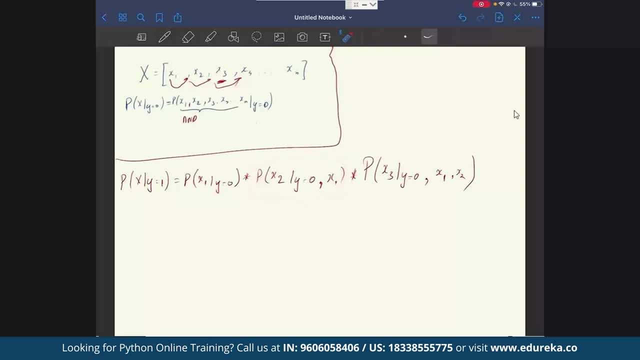 And then we have also calculate the probability for the second word according to the naive bias assumption, This word is totally independent of the first word. So the first word can have higher probability of being a spam and second word can have higher probability of being not spam. but they are totally independent of each other. 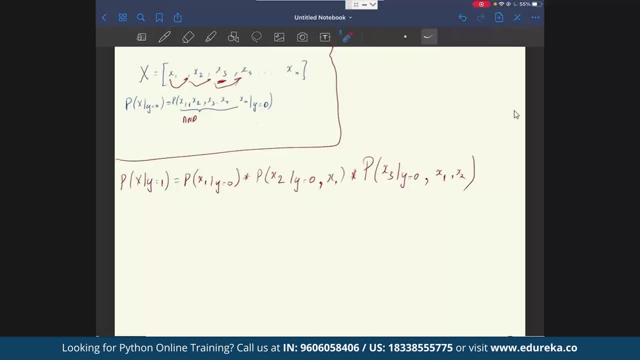 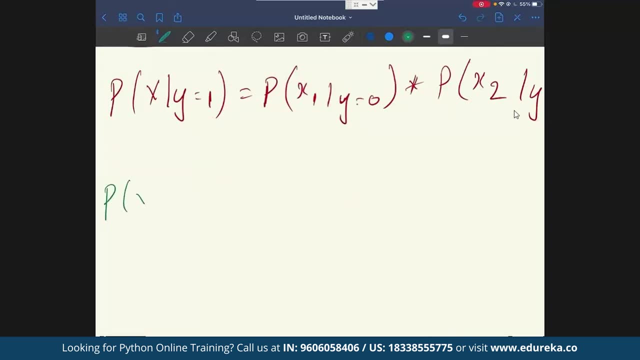 So this is what is naive bias assumption is. so let's now see how this equation would look like after naive bias assumption. So what we're going to do is I'll write one below the other so that we get a better understanding. So, if Y is equal to 1, if an email we can write, 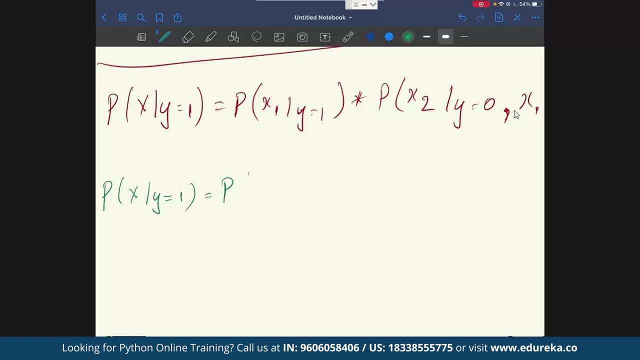 We consider that to be a spam email only if P of the first letter or the first word of that email is spam, is equal to 1. This will give us some probability, and then I'll multiply that with probability of a next word in that email being a spam. 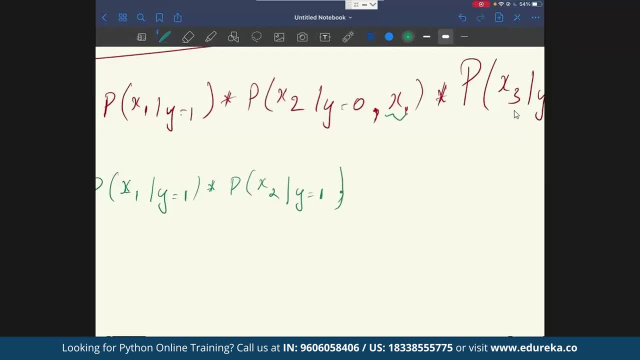 So, and then this won't be dependent upon the second value here, and then I'll multiply this again by the third word, P of X of 3. that is nothing, but the third word is equal to spam, because over here We're trying to find the probability that email. 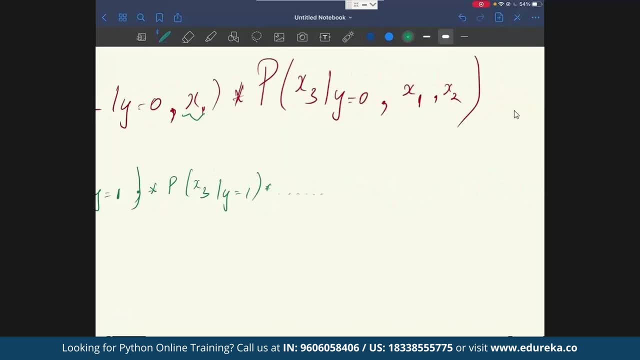 Belongs to spam category, and this would continue for the nth term. P of X. n when Y is equal to 1.. So you see here right that none of the probabilities are dependent on each other. does reducing the computation need? Okay? So in order to put this in a mathematical form, what will happen over here is P of X. 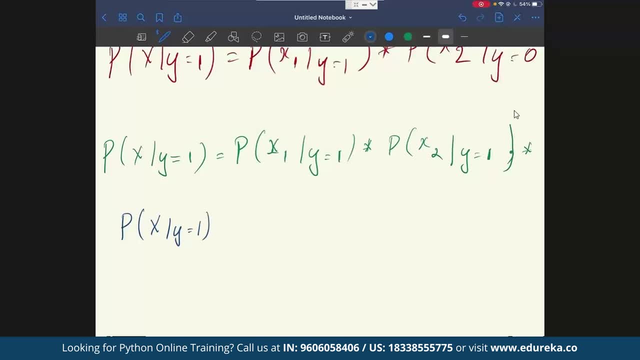 that, or we can say P of email belonging to a spam category is equal to the product. Okay, So this is multiplication, right? So for summation we use this and for product We use pi. Okay, So this is for product, and where I will range from 1 to n and then we'll have probability. 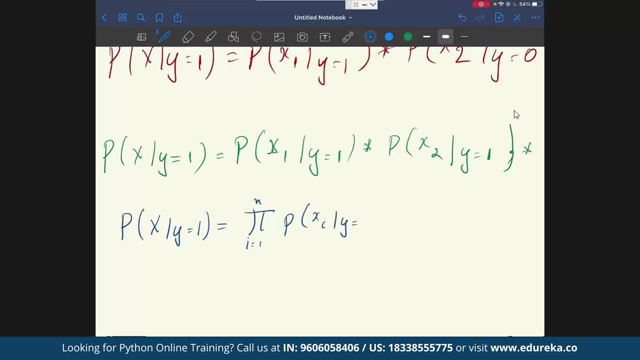 of X of I when we know that particular character or word belongs to a spam category, and same way will have for non-spam. Y is equal to 0.. This is nothing but pi, where I ranges from 1 to n. probability of X I when we know Y is. 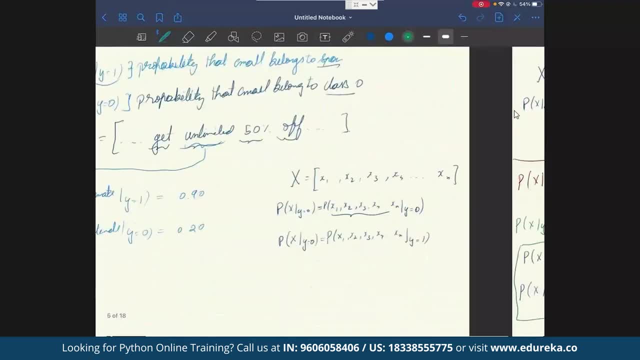 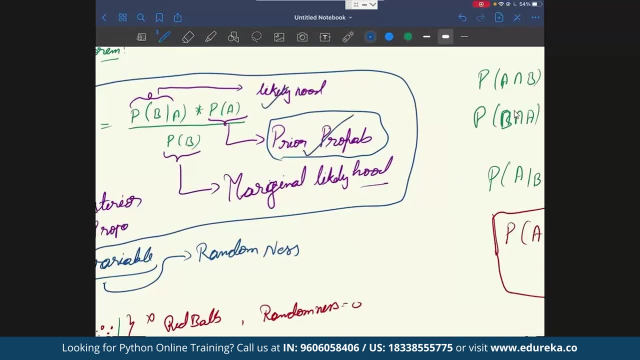 not a spam. This is an equation for our likelihood. So now, as you can see, right, we have found the value for likelihood, We have found the value for posterior probability, We don't have to calculate marginal likelihood, so we can just keep that part. and now, finally, 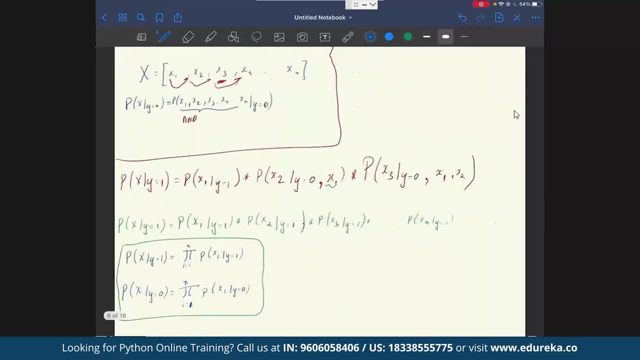 we are coming down to posterior probability. So let's now see how we can substitute our values and calculate our posterior probability. So, posterior probability, that's nothing but P of. we feed an email, right? So P of X. I let's write a generalized version where Y is equal to C, C here refers to the. 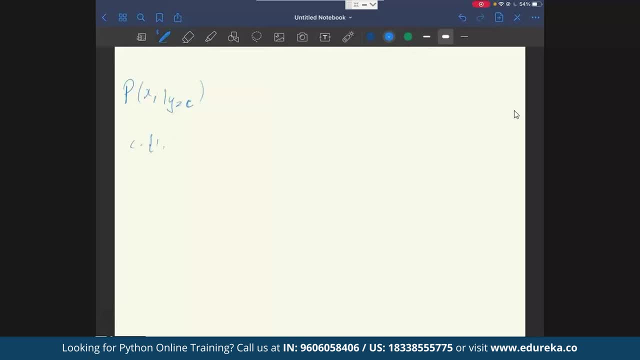 class. So the class here is nothing but either spam or not spam. This is equal to on top will have the likelihood, right. So let's write the likelihood first. So here we'll have something. pi I is equal to 1 to n. probability of X I. that is going. 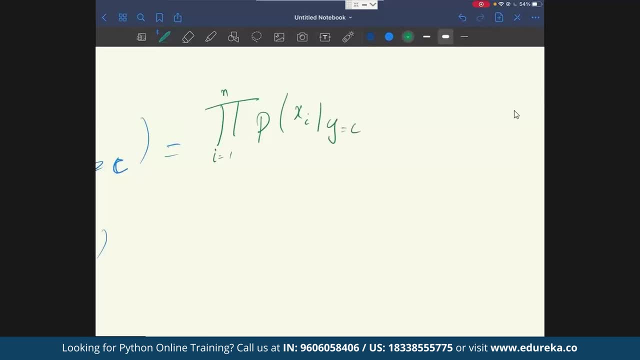 through each and every word in an email. Y is equal to C. C can be either 1 or 0. we will multiply this by prior probability right, which is nothing but 1. by M, I is equal to 1, n here. so it's going to be: Y is equal to C and obviously we have to put the normalization below. but 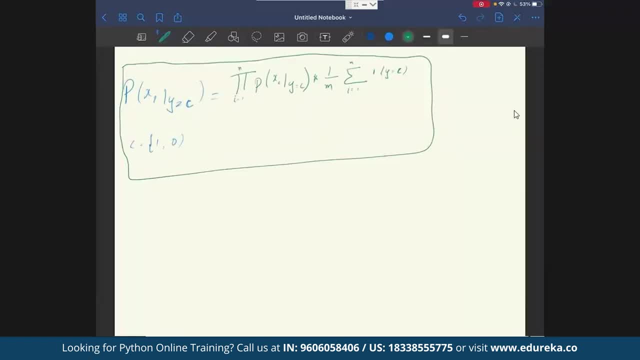 we can skip it because it doesn't make any difference, right? So this is the equation for our naive as algorithm, This is the way how we can classify our text. Let us now go to my code editor and try to code the entire algorithm. 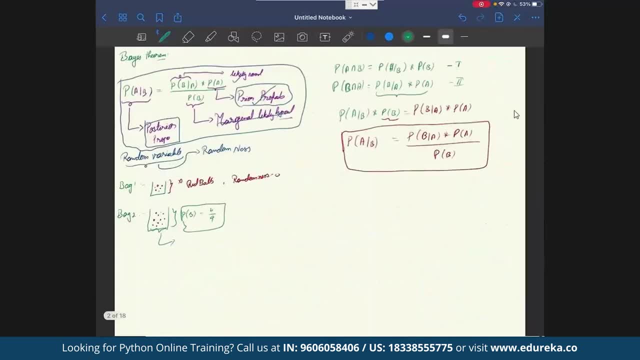 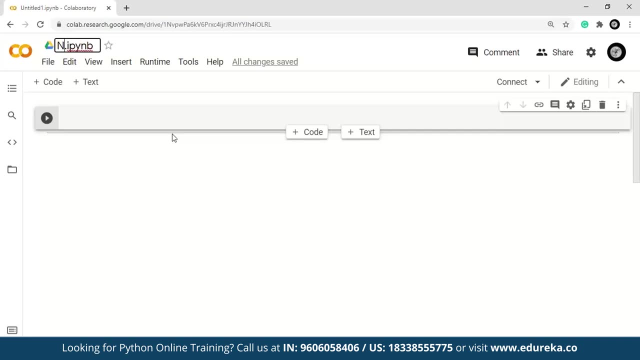 This would help us in understanding how the underlining working of NLTK works. Okay, So, as you can see, I have come here to my Google collab. let me quickly give a name as NLTK, or let's give classification implementation. So let's get started. 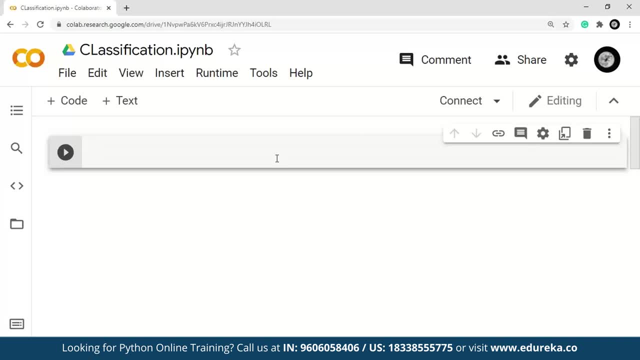 Now a couple of things that we have to import. So let it be import pandas as PD, then let's import numpy as NP and then let's have a label encoder. So basically, we use label encoder to convert our text into numerical form. and if you are, 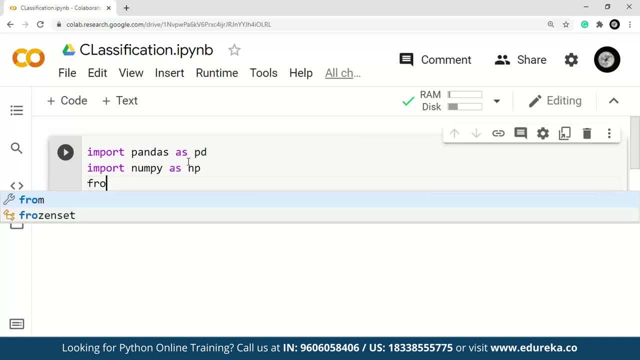 asking why we are going to convert our text. We are going to convert it into numerical form. that's because computer, no matter how advanced it is, It is unable to understand textual form. So it has to take the data in our numerical format, Okay, from sklearnpreprocessing import label encoder. and finally we need sklearnmodelselection. 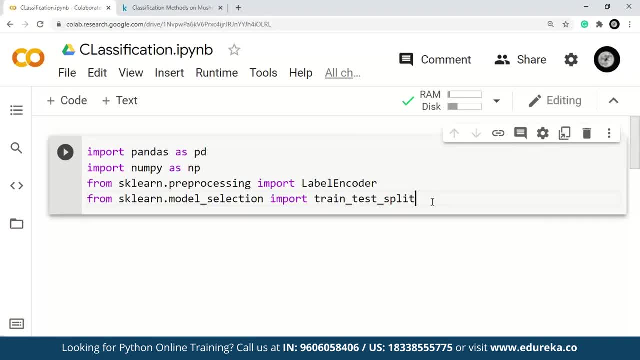 import train test split. All right, so let us now execute this. So in our next stage, right, we will have to get our data set. So getting data set. So here we'll be using mushroom data set. So what we're going to do is DF. 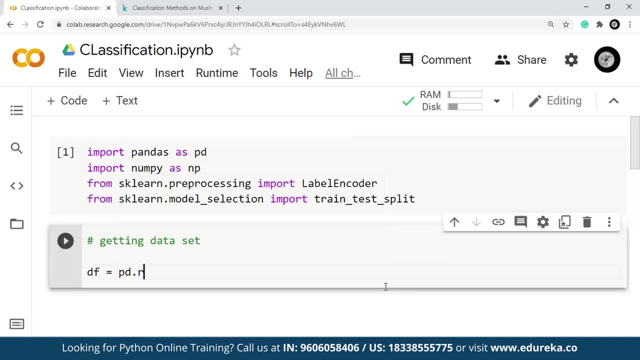 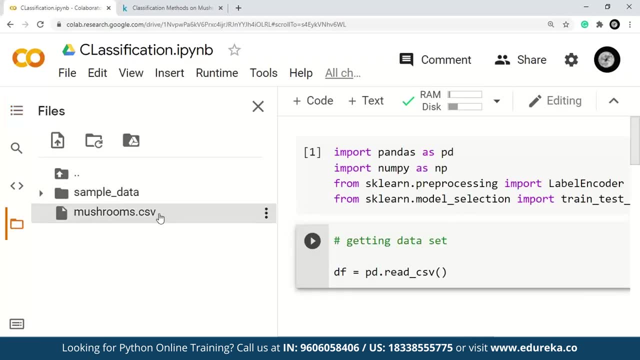 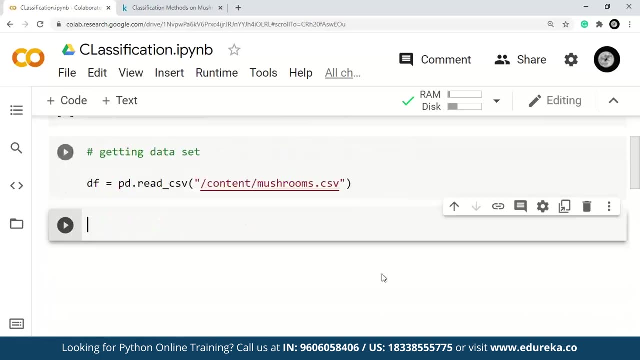 We know it's going to be in data frame, So pandas dot read CSV, and the place where I have my file over here is here, and I'll just quickly copy the path and paste it over here. So let me execute this code. fine, And now let's see the shape of our data set. 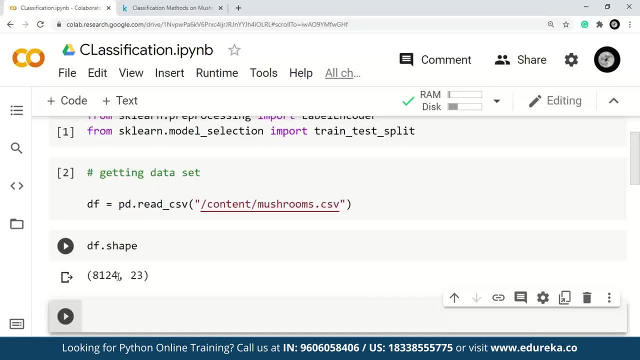 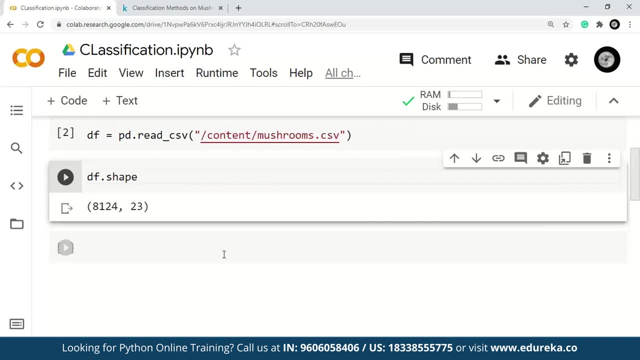 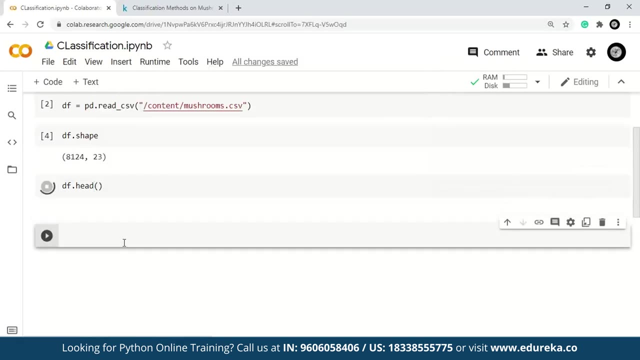 So it's going to be DF. So what this represents over here is that we have 8142 pros and then we have 23 features. So let's now see each of these. So let me just print this DF dot head, Let me slightly zoom it out and let me play this. 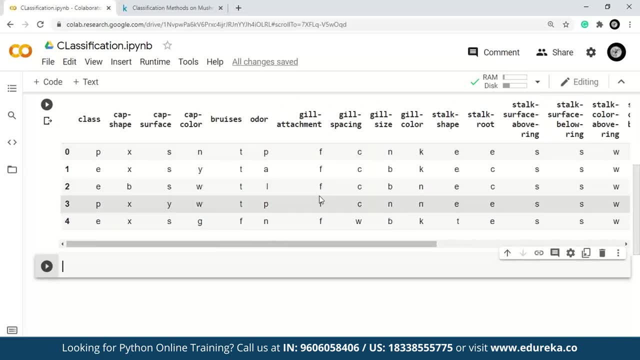 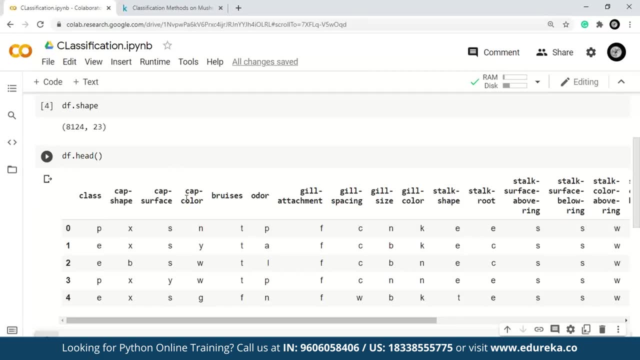 So, as you can see, here we have all our data in a textual format and then we'll have the values, which would range from 0 to 8124, and then the features over here are not the same. but you know, cap shape, cap color, cap surface is nothing but the surface of the mushroom. 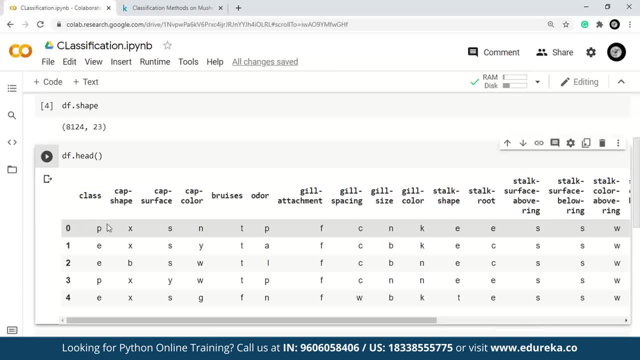 and the class you can see here, right. So this part over here, this class, is nothing but Y, and all of these features over here are represented as X. So now what we'll do is let's try to, you know, encode this. Let's try to convert these values into numbers. 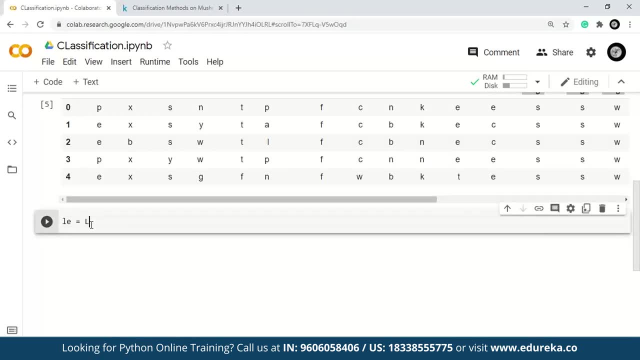 So what we'll do is le and we're going to use label encoder. Okay, so we are creating the instance of this and then we'll have DF encoded. That's the DF standard. That's the transfer data frame. This is nothing word. 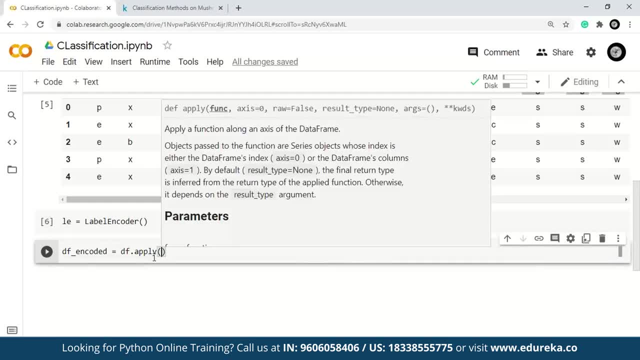 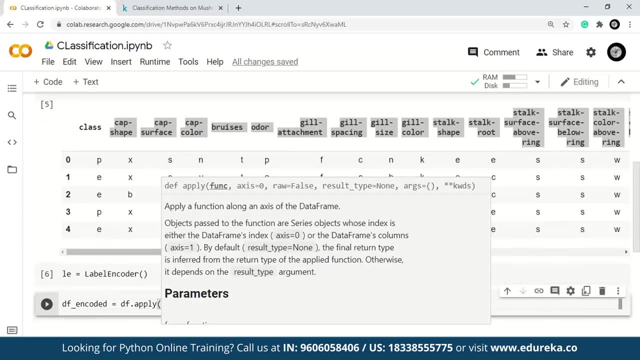 You have got apply, Okay, applies one of the method. what this apply method does is it's like a for loop over here, So it will go to each and every row and each and every column and apply whatever function we pass. and we're going to pass label encoder, right. 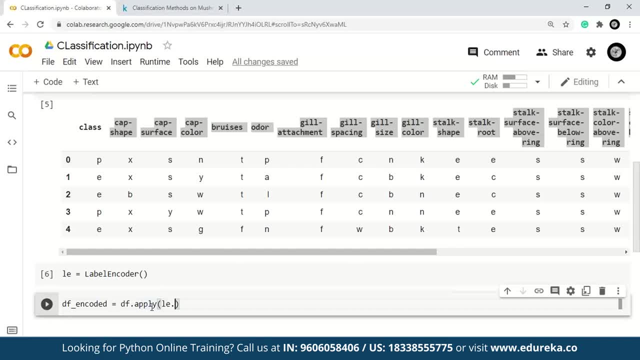 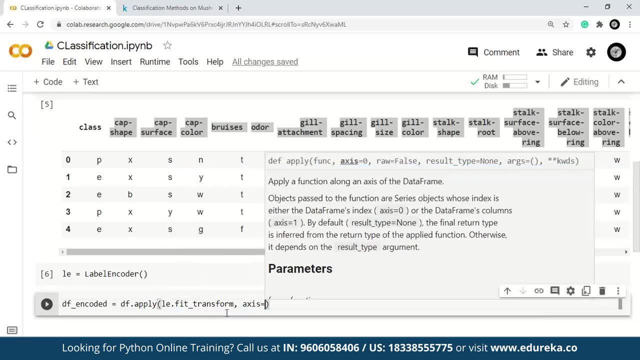 So over here I'm going to pass your le dot fit transform. will we just have to give method name and no method call and then we'll give axis? by default, axis is 0.. We want 0 because we want it to go by every row. 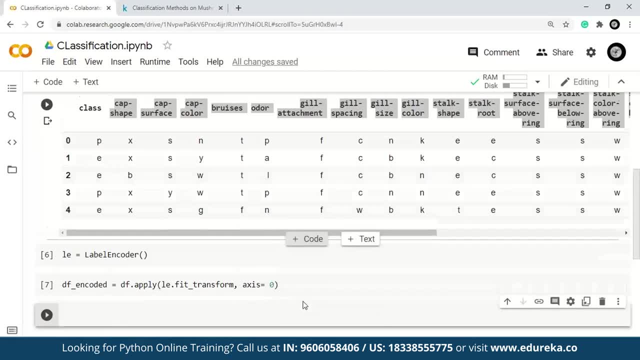 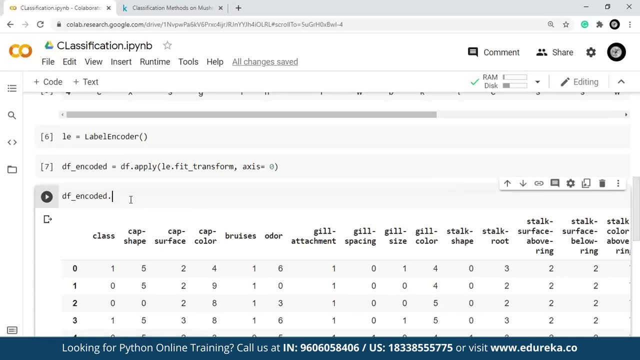 So let's now execute this. So let's now execute this and let's see how our data would look like now. So, as you can see here, this is our data, or let me just give it as head and let me zoom out so that we can compare this data with this. 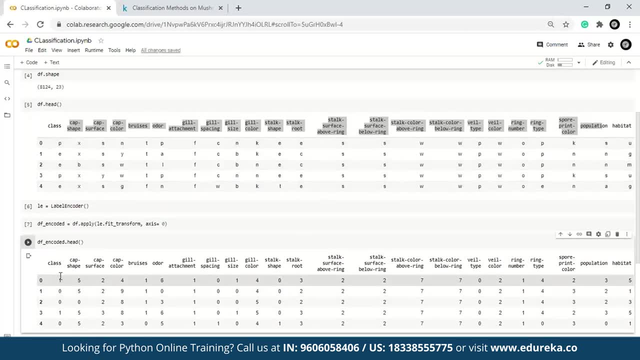 So these both are the same thing. Okay, as you can see, our class class, and then we have cap shape, and all of these are the same thing. only thing: after performing label encoding, all of these values have been converted into numbers, So now what we'll do is we obviously need to convert this into a list of others. 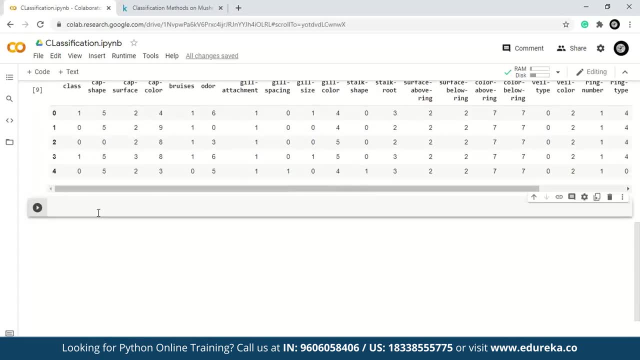 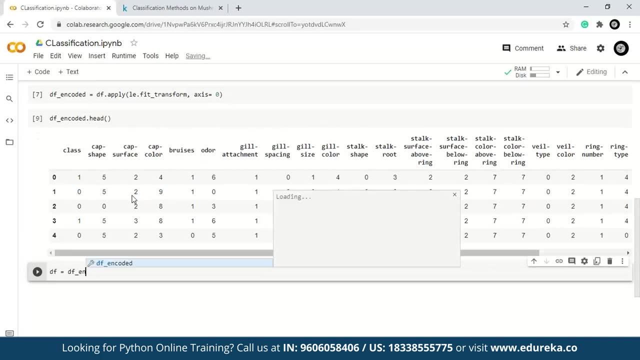 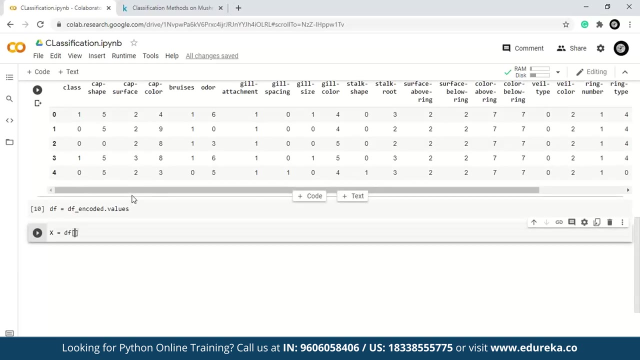 Right. So let's finally do that. So let's, DF is equal to encoded DF. So let's see what it is. Yeah, DF underscore encoded dot values. and now we'll have to define our X. our X is nothing but DF. So, as you can see, right, this is why this class refers to Y and X is all of these features. 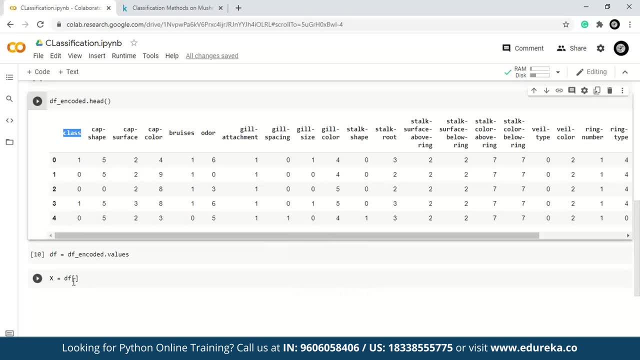 except the first column. We want all the other columns right. So what we'll do is from column 1, because this is column 0. We want it to all the columns. So basically, here we want all our rows, that is, 0 to 8000, some change, and then except first. 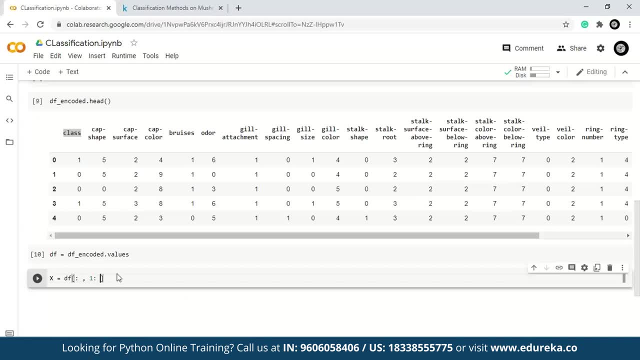 column, the 0th column. We want all of them. Okay. So this is X, and for Y it's going to be all the rows. I hope you understand why it's all the rows, right. So it's 0, 1, 2, 3 and we need it for all the values. 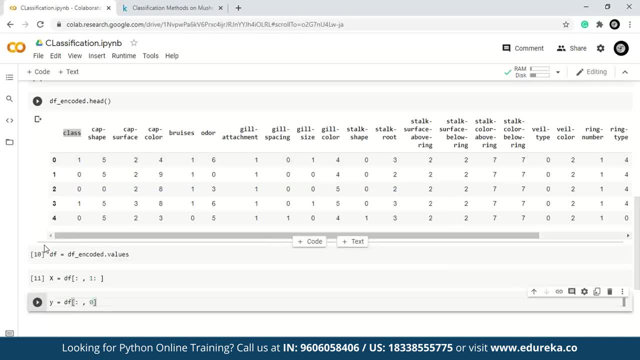 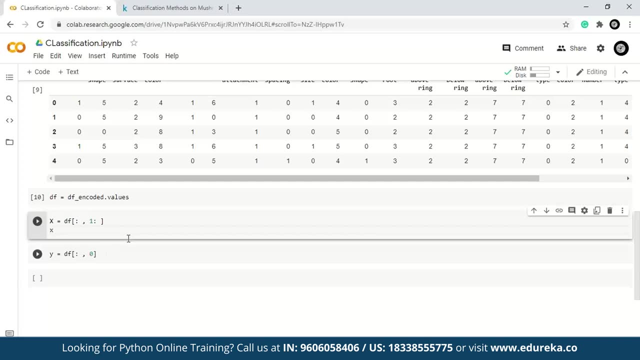 So it's all the rows and only the 0th column, because 0th column gives us the class right. So let's quickly execute this and, just for your satisfaction, Let's see how it would look like. So here out, press X. so you'll see here that, yeah, it's going to be capital X, right uppercase. 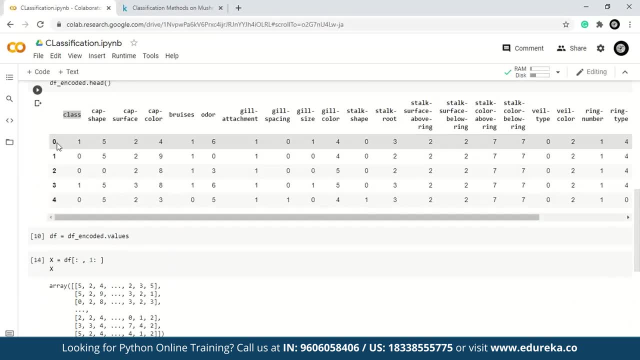 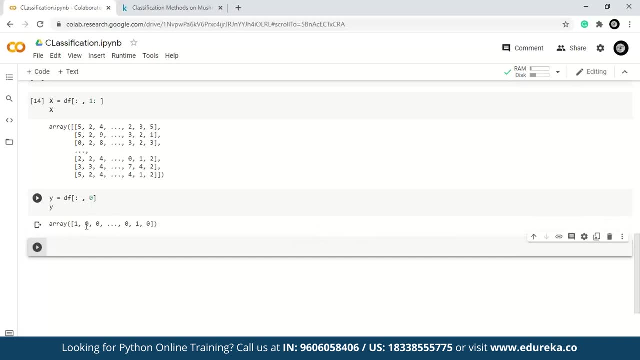 So everything has been converted in an array and except the first part, except this part- will have all other values, and similarly let's see it for Y. So, as you can see, here we have just single column. So now what we'll do is we'll split our data. 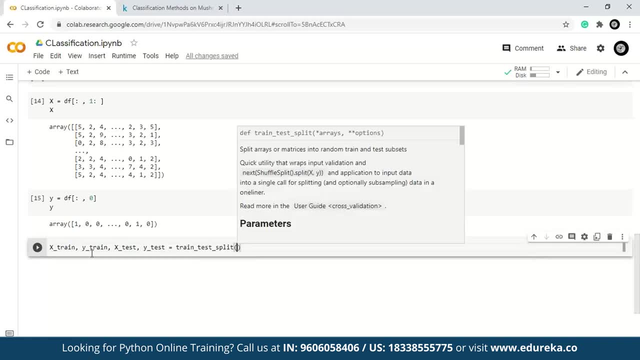 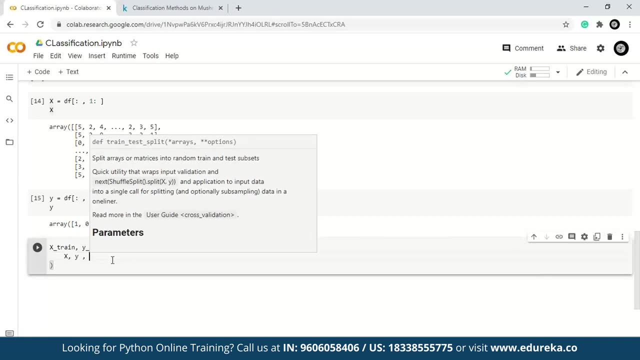 So this is going to be: we are going to use train test split. So here we're going to have the value of X and then Y, and then we have to give by what person we want our value to be splitted, right? So for that we'll give something like this: 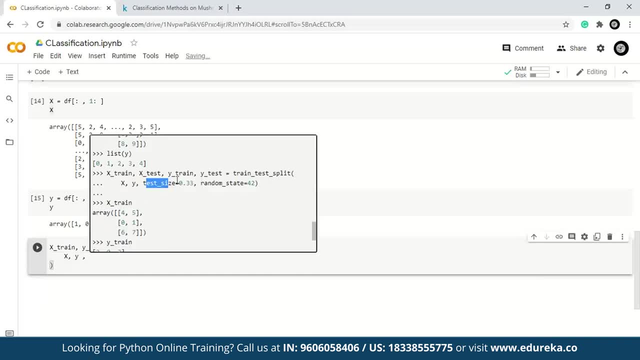 Okay, Yeah. So, as you can see here, we need our test size, right. So we need a test size and a random state. So let me just copy this from here. Now, what this test size resembles is by what person we want our data to be splitted. 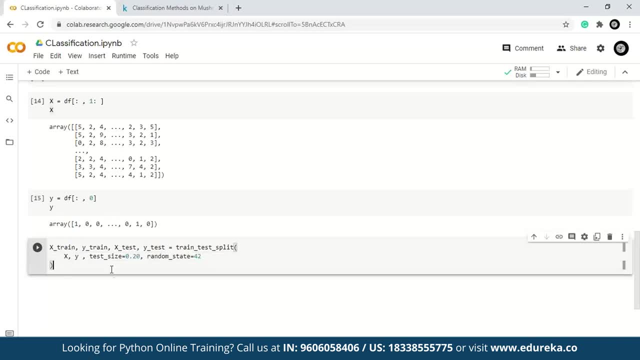 So let's give it as 20% and let me execute this. So, now that we have all the data and every requirement, So let us know, directly jump into having our knife by his classifier. So let me give you a quick recap here: in order to get a knife bass classify, 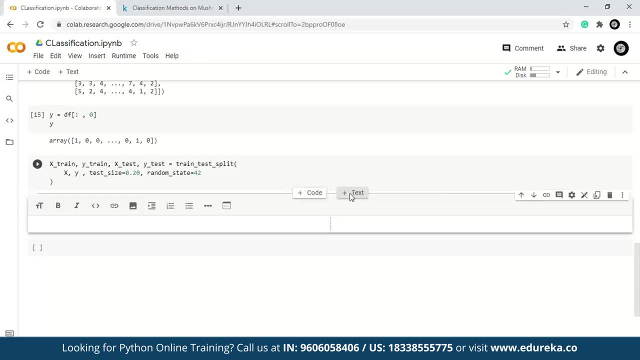 We need to find posterior probability. In order to find the posterior probability, We need to find something called as likelihood and prior probability, And then we're going to have prior probability. So we need to find the posterior probability And then we're going to have prior probability. 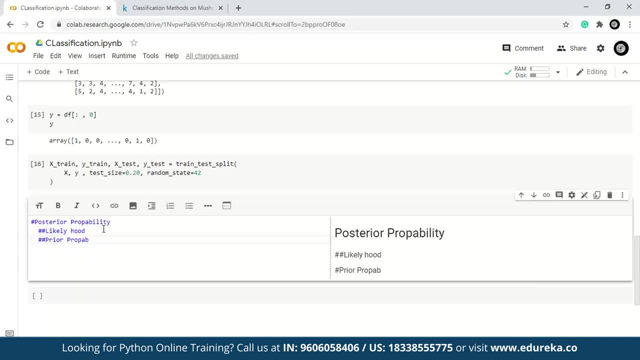 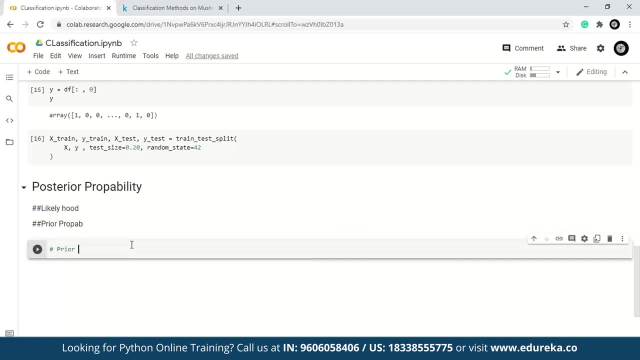 Let's not calculate each of this. and we start this by calculating prior probability. Okay, because probability is pretty simple to calculate. So let's not start off with prior probability. So we'll create a function here: Def prior probability. So this is nothing, but you're going to pass white train. 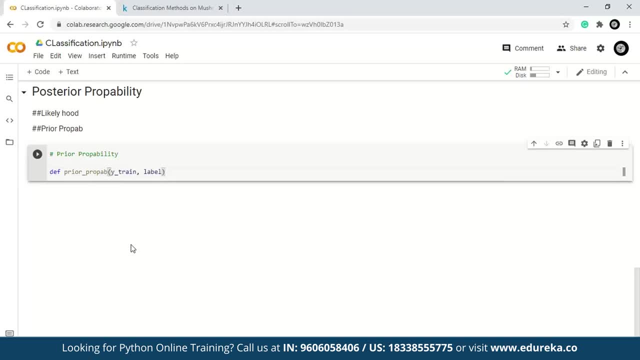 And then we're going to pass labels. Okay, labels over here refers to X and 0 values. Instead of giving white train, that generalize it to give Y. And now what we're going to do is we need to find the size of Y. 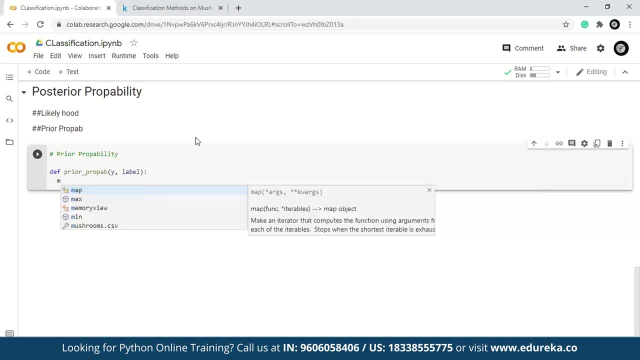 Right, So, because prior probability is nothing but sum of either X or 0, whole divided by the total number of classes. Okay, So what I'm trying to say here is: if you have 100 emails, out of which 40 are spam and 60 are not spam, 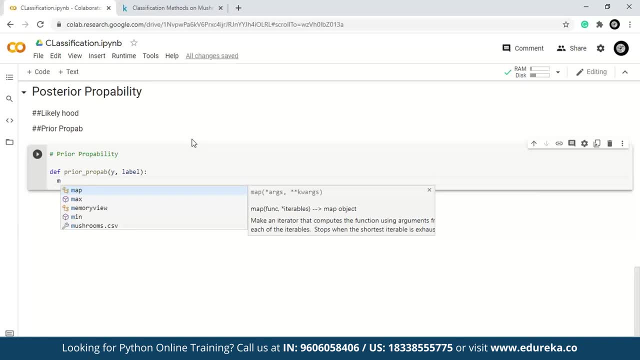 Then probability of email being spam is 40 by 100, and the other one is going to be 60 by 100.. Okay, So for that we need to find the total size Right. So it's going to be y dot shape. 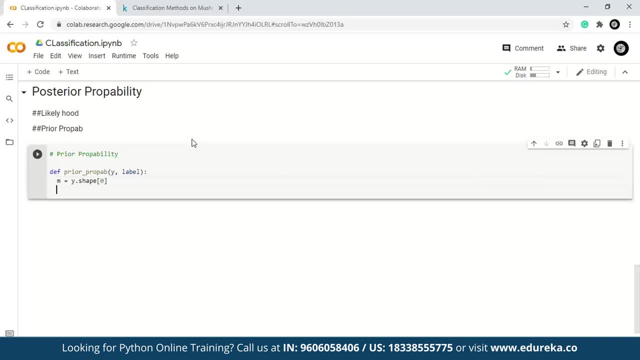 And then this: It will give us an array Right, So we need the first value. apart from that, We need a sum Right, So s is equal to NP. dot. sum White train, or let it be y values is equal to label. 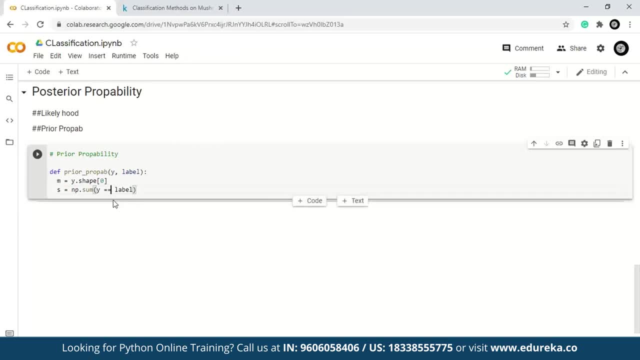 Hope you understand why we are doing this. You see why? value has only class values, Right? Only if the class value and label value are same, you're going to get one. So this is how we are going to do here, and this is going to return us prior probability. 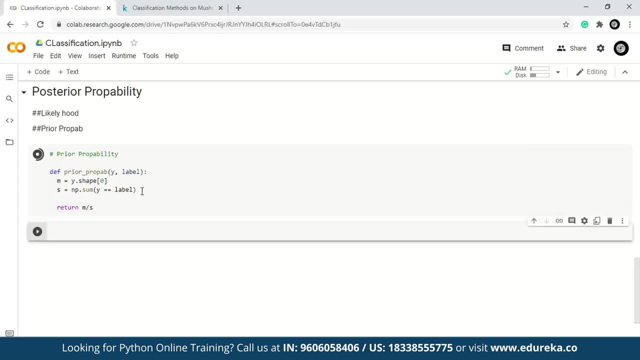 So written M by s fine. So now let's find our likelihood. That's our next task, and in order to find our likelihood, we need to have conditional probability. Okay, so def conditional probabilities. This is going to take a parameters like X and then Y. 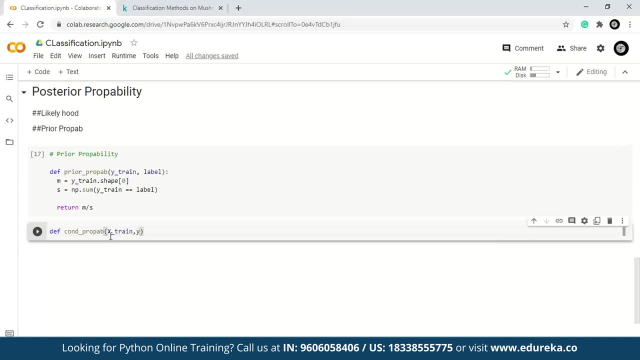 So we give here as X train and not X, and then we'll have white train, And then we obviously need to find feature column, And then we need to have feature label And then finally label: Okay, So what this feature column says is it represents which column we want that particular feature. 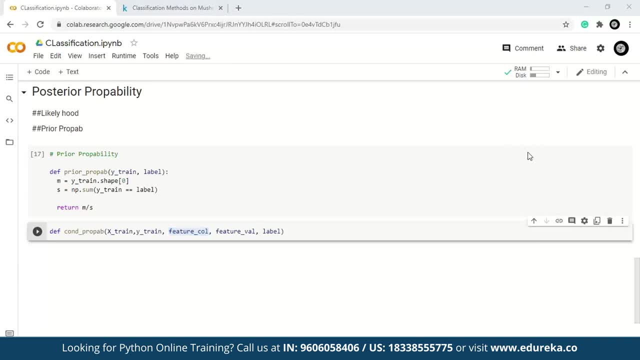 So, as we all know that this is nothing but a tabular data, right? So let me just quickly show you how it would look like. Okay, So over here we have a table, and this table will have multiple rows and columns, Right? 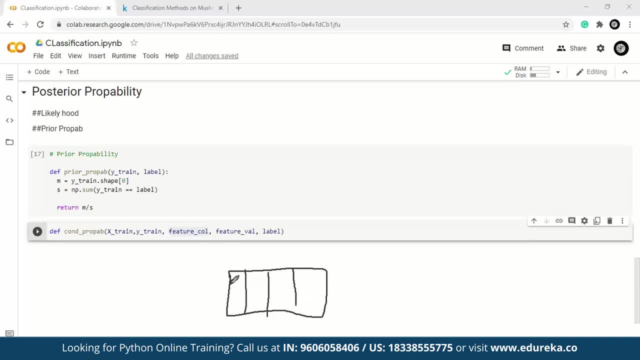 So what this feature column represents is within this feature column. within this column, which value? value represents The values present in the feature columns. Okay, So let me just quickly know it is this and move ahead. So what this will do is we are going to just filter out the value, right? 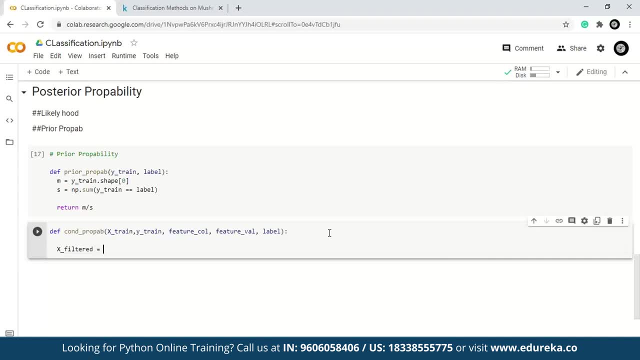 So X filter, This is equal to X train, where white train is equal, equal to labels. So over here we'll just get the email values, which is either spam or not spam. That's why I'm giving here as X filter, and number is equal to NP dot sum. 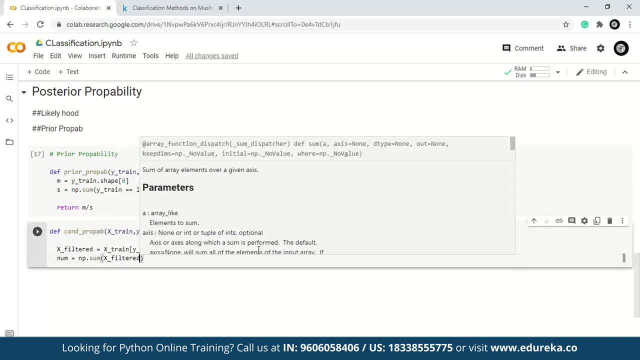 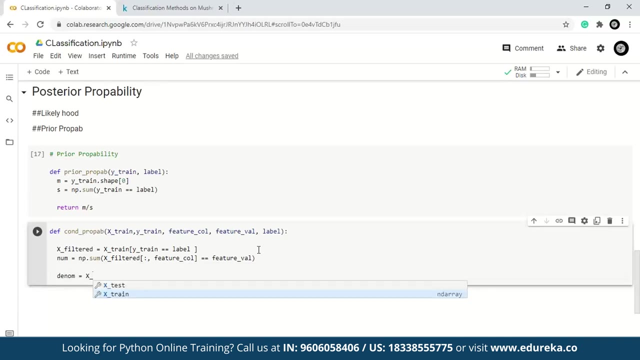 It's going to be X filter, Where we have all the rows and the columns are going to be feature column, Which is going to be equal to feature values. And now for denominator. So it's going to be X filter, Dot shame, which is nothing but total number of values, right? 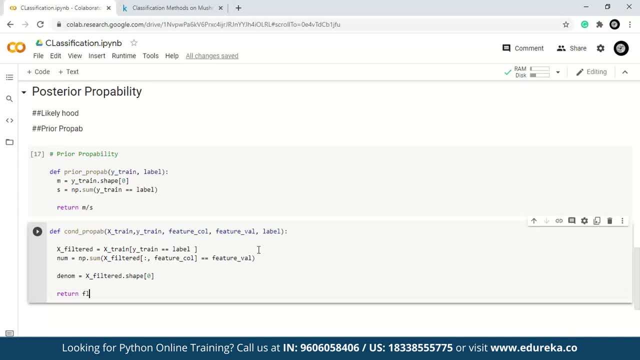 Zero And this would return us numerator by denominator And let's give it as float over here And it's going to be numerator Divided by denominator. Okay, there's nothing but the conditional probability. Okay, I hope you remember what is conditional probability when we were discussing the derivation. 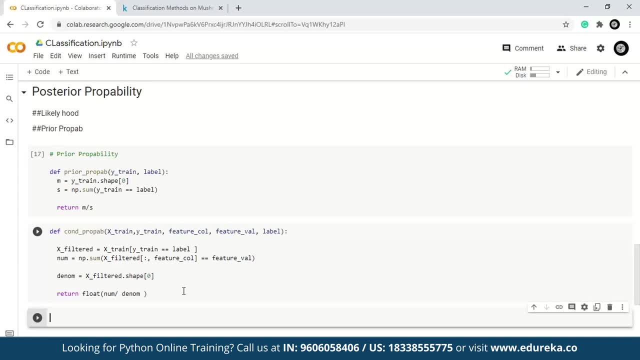 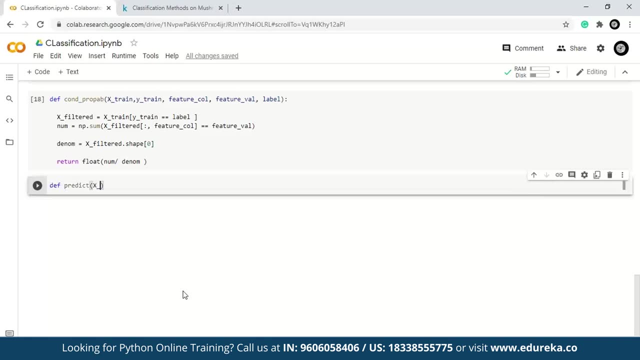 So now what we're going to do is we obviously have to predict our class, right? So let's do that. Let's write this function here: Predict, def, predict. This predicts takes two values: X train, White train. Apart from that, we also need to perform predictions, right? 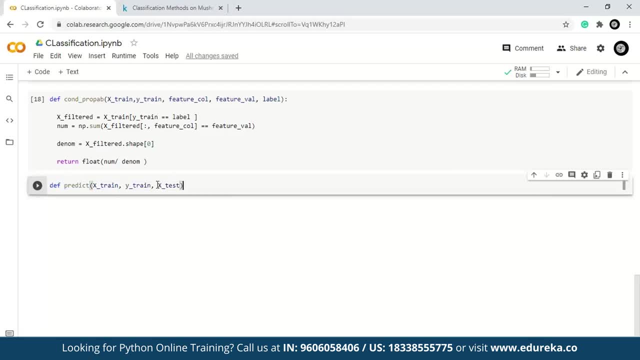 So that's why we also need X test. So now what we're going to do is We'll have classes. classes refers to beat spam or not spam over here. It's going to be poisonous or not poisonous, because here we are taking mushroom data set. 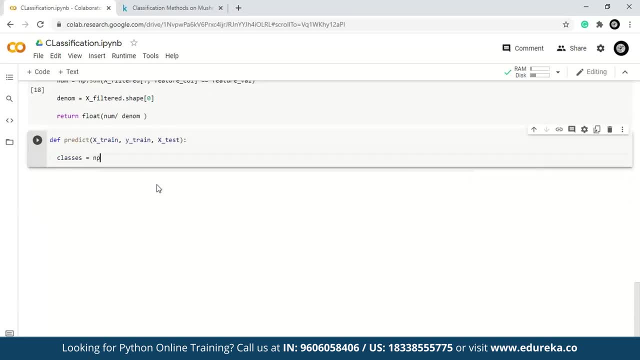 right, So classes is equal to NP dot unique. Why? right, So it's going to be Y train. Okay, What this predict will return is white test values. Whatever value I feed to this, I'm going to get the answer for that. 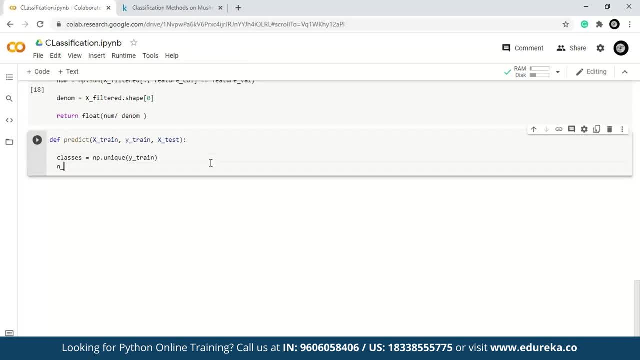 Okay, So now we also need features. So in features This is going to be equal to X train, But shape, All right. so let's not calculate our posterior probability. So, posterior probability, Let's leave it empty as of now. 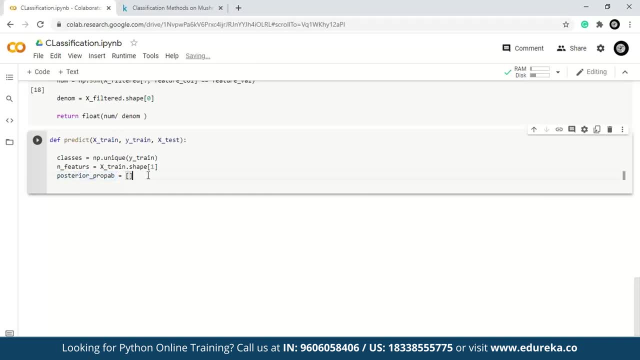 Okay, So for every value of a posterior probability we'll get some percentage. So this percentage represents, you know, probability of that particular word being a part of spam or not spam. So here we're going to have four Label in classes. 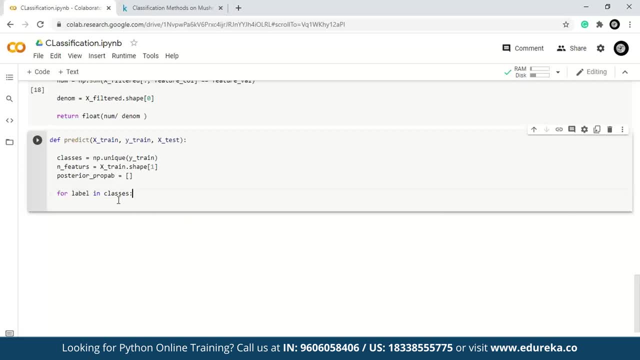 This means that we are going to go class by class. So either spam or not spam on over here It's going to be. either It's going to be poisonous or non-poisonous. So the values of classes can be either 0 or 1.. 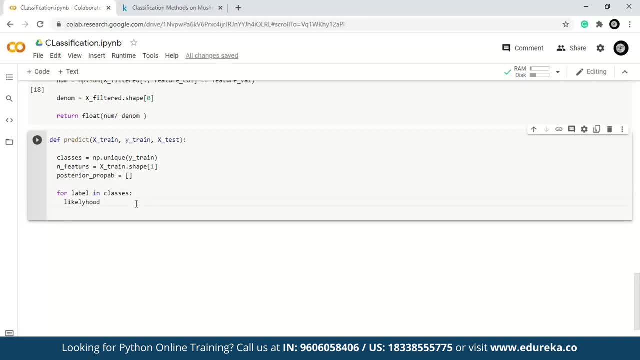 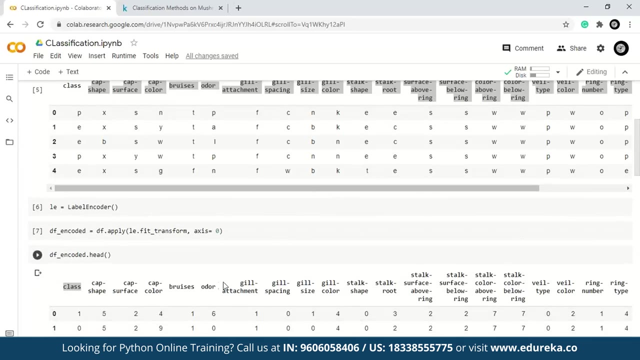 Fine, And then we are going to give likelihood, We'll give it as 1.0 and then for features in range and features: Okay, And features represents the column over here, Right? So these are the end features, except the classes. 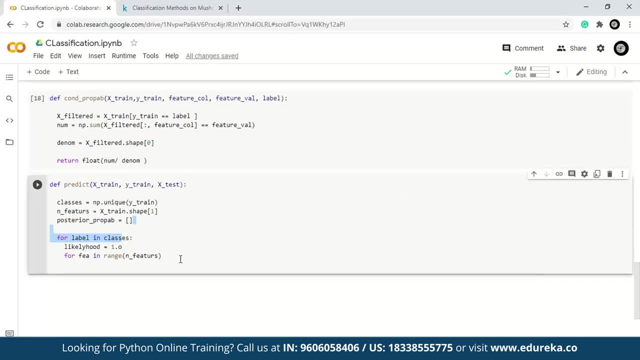 Whatever is that? they are nothing but the end features, right? So yeah, so go through each and every feature, or in short, I can say go through each and every column, and then find the conditional probability. CO and D is equal to conditional probability. 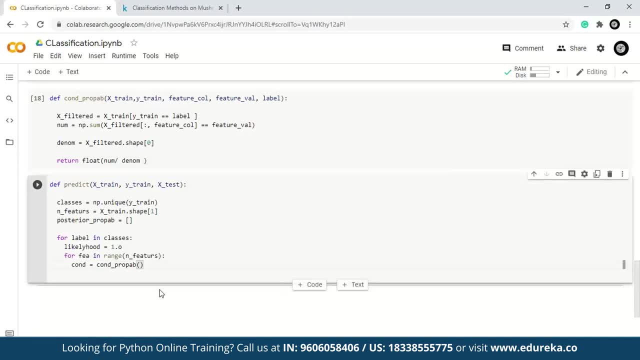 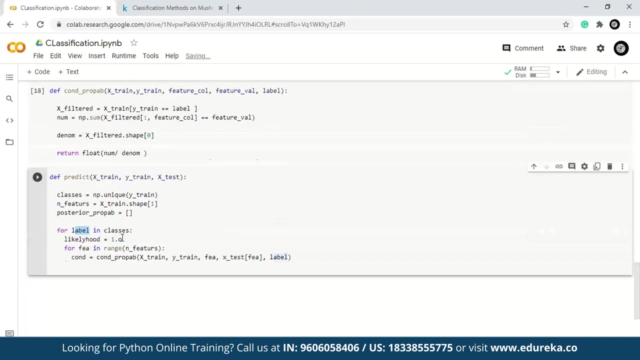 Here We're going to call this function. So now we have to pass our X train values And then we have white train, then the features: if here and within the features which feature you want, Okay, And then we'll have labels, Okay. this label over here represents whether the class is either X or 0. 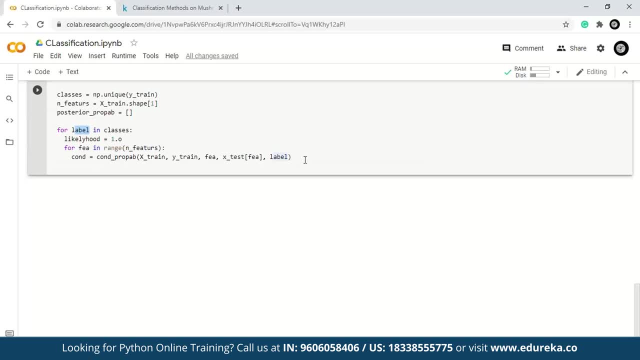 So now what we're going to do is you're going to calculate our likelihood. So likelihood is equal to likelihood plus conditional probability times, conditional probability. So this likelihood over here, We're just randomly initializing it over here and for every iteration of this for loop. 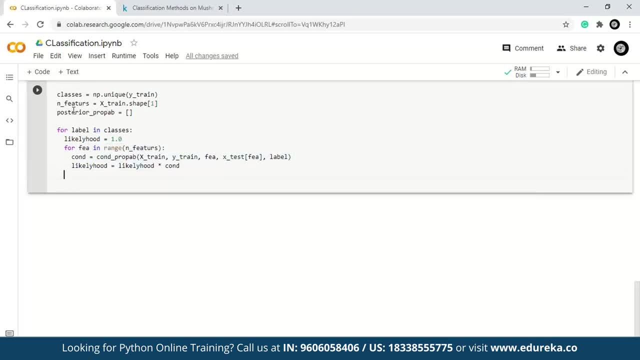 likelihood increases. So now all we need to do is we need to append prior probability, So here. so we'll give here, as prior is equal to prior probability. Okay, this is nothing but this function over here which we have defined where we're going. 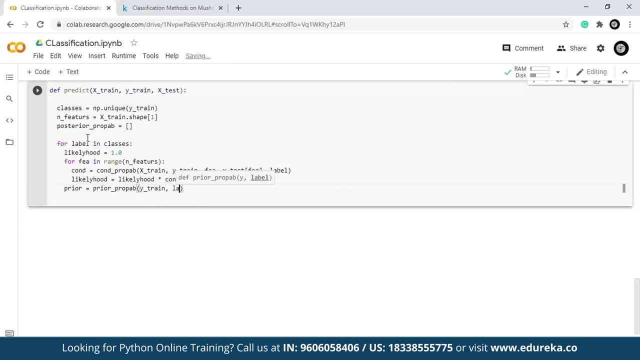 to give white train and then label, and then for posterior probability There's nothing but likelihood. times Prayer. Okay, I hope you remember the mathematical equation for this particular part. So we are trying to find prior and posterior probability for each of this. 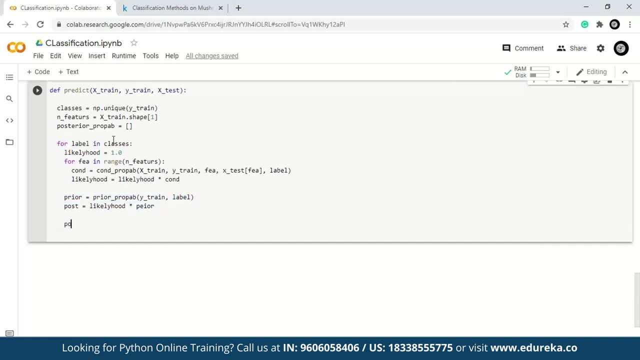 And now what we're going to do is we'll just append these values over here, So we'll have posterior prop dot append and the value that I want to append is post. And now what we'll do is we need to find the probability which has the max one right. 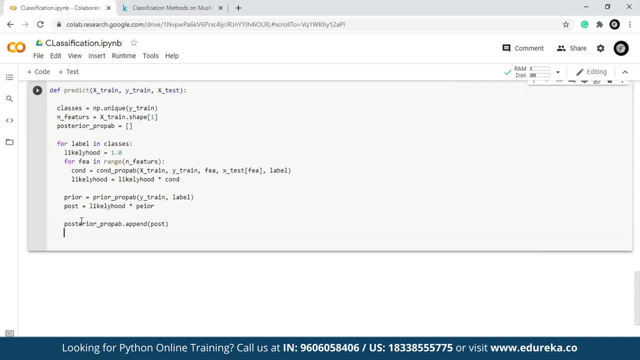 So for that we are going to use argmax over here. So predicted value is equal to NP dot argmax. argmax gives us in which place we have the highest value right. So that's what argmax does, And so we'll give you a posterior probability. that is nothing but this part. 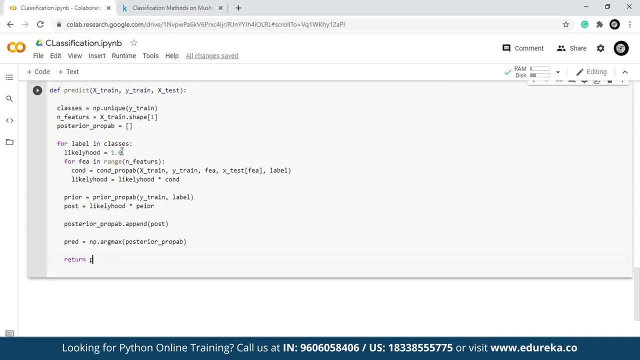 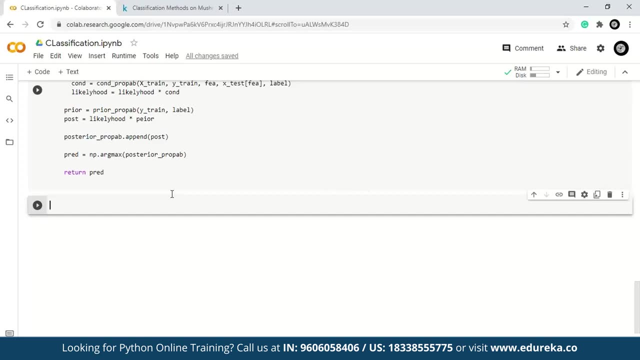 And this would return as the class right. So written predicted. Okay, so this is done, All right. So let us now do one thing. Let us now find out by what accuracy we are finding this value, So let's also calculate the accuracy that will have a correct values right. 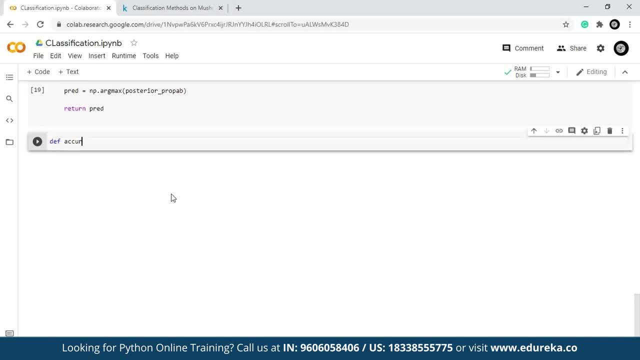 So to do that, Def Accuracy, X train, X test, And we also need to give y train and y test right. So y train And it's going to be y test And within this function, what you're going to do is predicted. 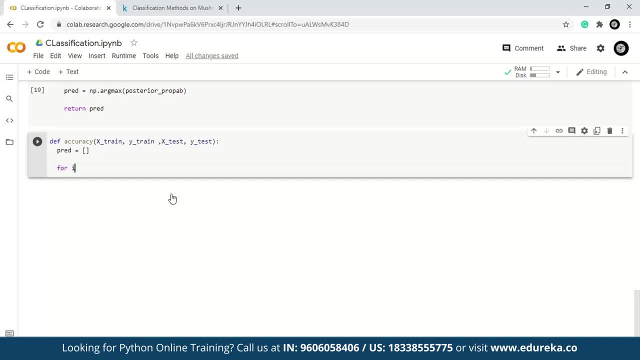 It's going to be an empty list. So for i in range. So it's going to be throughout all the values of x, right, So x test Dot shape. So now here it's going to be. p is equal to our predicted value. 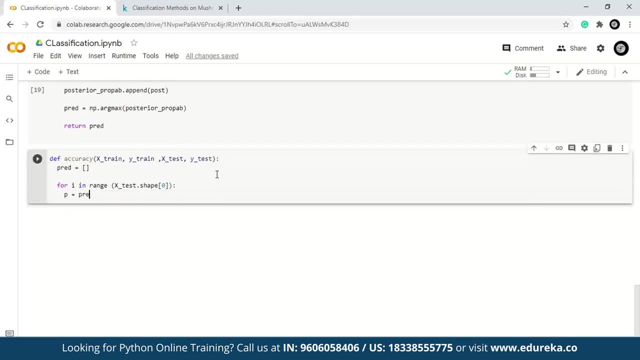 So now we'll call this function here: Predict X train, Y train, And then we have X test And as we are doing this for all the values, we'll just pass here. I, every time I perform this, predict right. 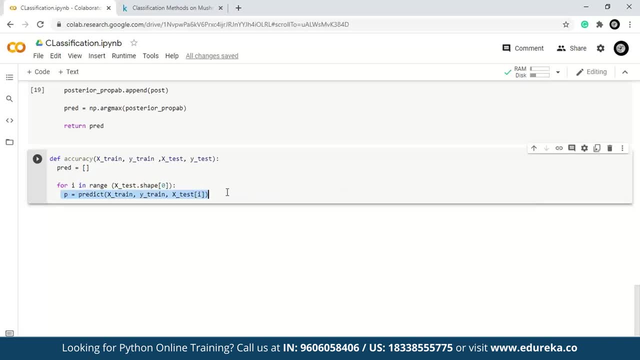 It gives me whether one example belongs to a mushroom class which is poisonous or not. So only reason why I'm doing this accuracy, or I can say, only reason I'm having this fault- Look here- is to find all the values and put them over here. 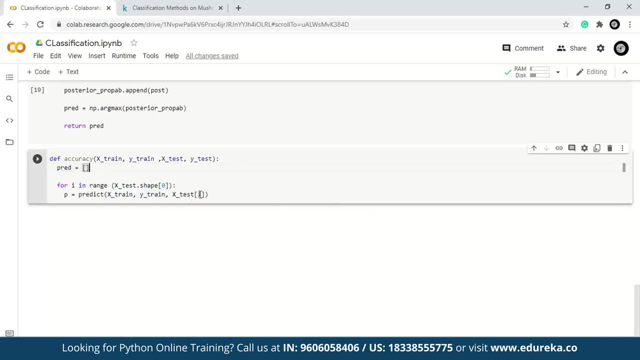 This predict list over here contains the predicted value of each of the test values. Okay, So now what I'm going to do is whatever value I get over here. So print dot, append P. Let's do one thing: Let's give this name as y print and will convert this predicted over here to numpy array. 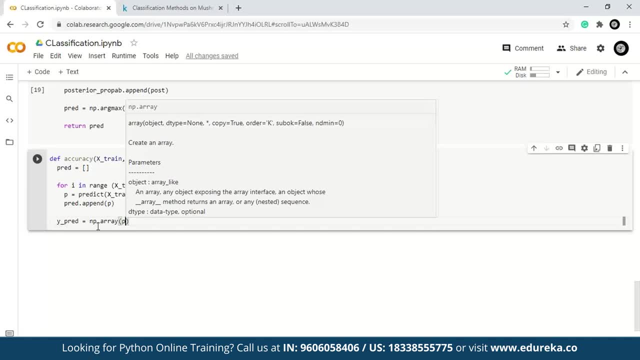 So NP dot array And we'll give you a spread. And now, in order to calculate our percentage, or In order to calculate the accuracy, All we need to do is- accuracy is equal to NP dot sum and we'll just compare this predicted value. 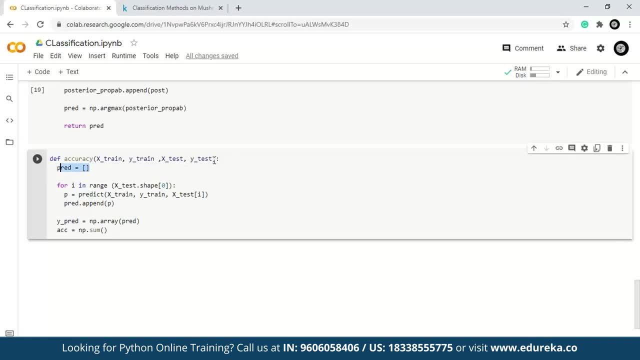 Okay, whatever values, because we get only ones and zeros with the value that we already know. Okay, This is just the way to have you know, testing your data, how accurate it is. So we'll have white bread Has to be equal to y test. 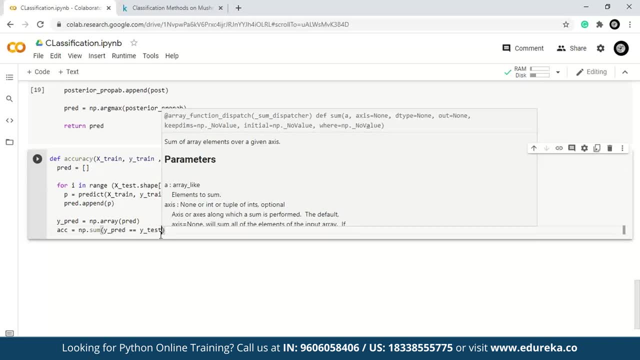 And every time these two values are same right, It will add up one and in order to get a value in percentage, We'll have White bread divided by the size right. So white bread by shape, and will give index is 0 and this will return as the accuracy. 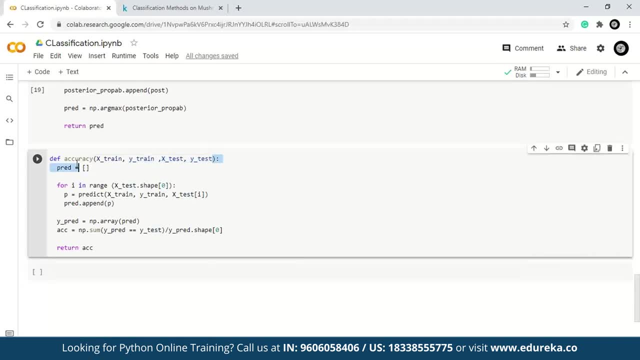 Fine. So let's call our accuracy here and let's give all these values. So before I run this code right, Let me just give you a quick recap. Our main agenda over here was to classify whether this mushrooms over here belongs to class of poison or not. 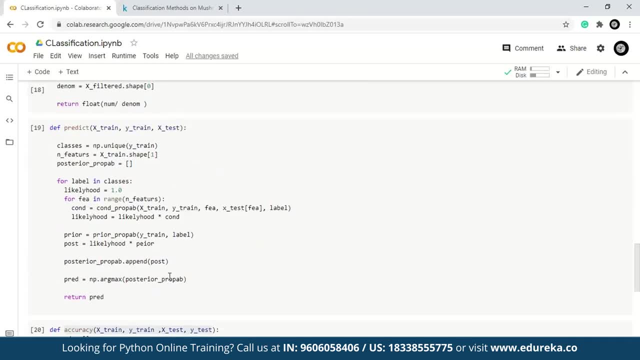 So that's what we are doing here. We have to do that, obviously, using posterior probability. In order to find posterior probability, We need two things. One is nothing but likelihood and another one is prior probability. funding for our probability is pretty simple, because we just need to find the total number of values by total number of other values, right? 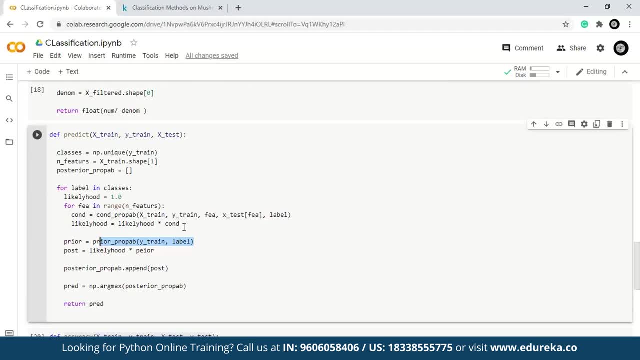 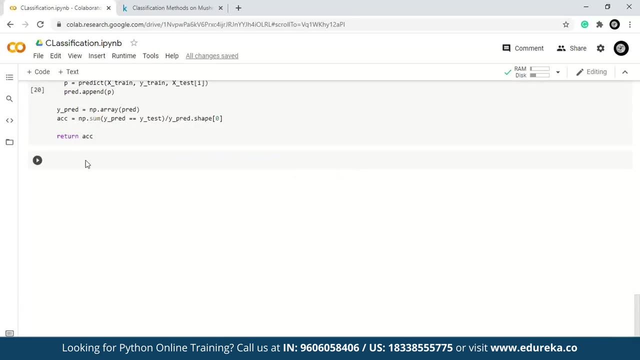 That's what probability does, and for likelihood It's pretty simple. Okay, we have to find the conditional probability, and then this would return us the predicted values. And let me now quickly run this and let's see What is the accuracy of our model. 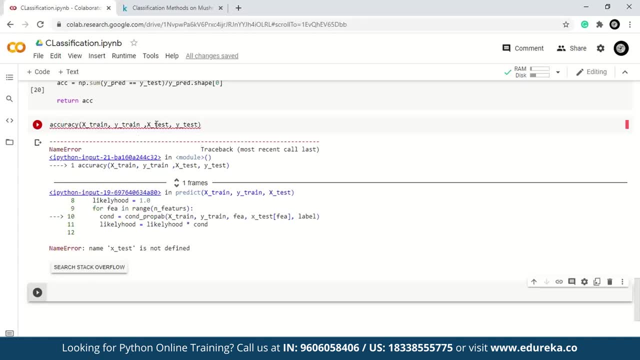 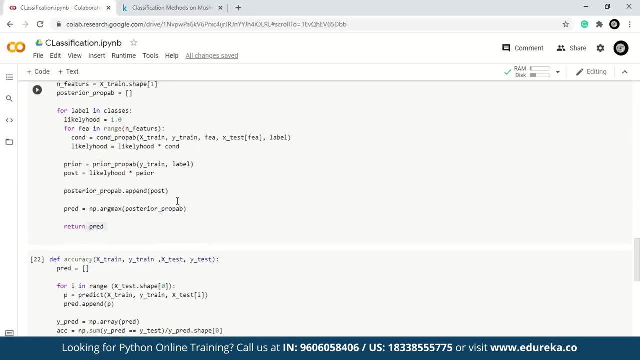 Okay, So it's saying X test is not defined and the reason why we are getting that is because we have given a smaller case value. Oh yeah, So let me quickly read on this now. Oh yeah, we have to give X as uppercase. 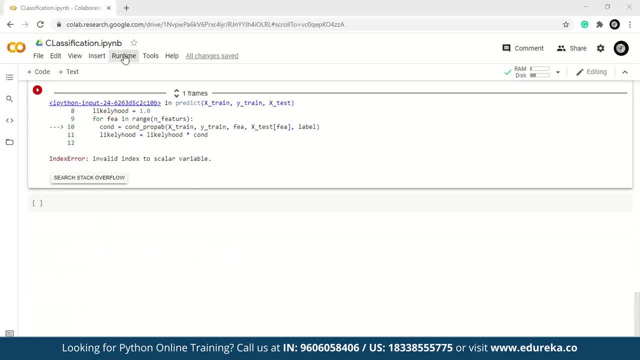 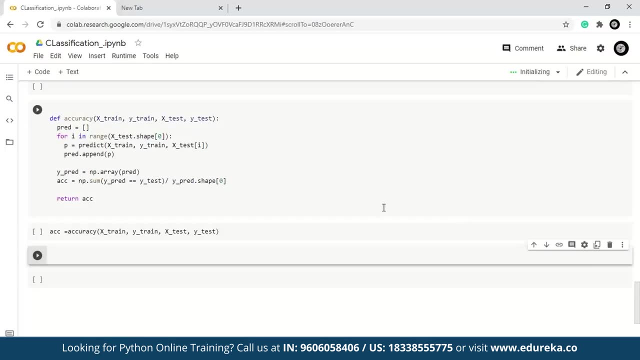 Okay. So, in order to overcome this, what we'll do is we'll quickly run this from the start here. Okay, So let's wait for our data to get a processed over here. Sometimes, what happens is when you're when you're trying to execute. 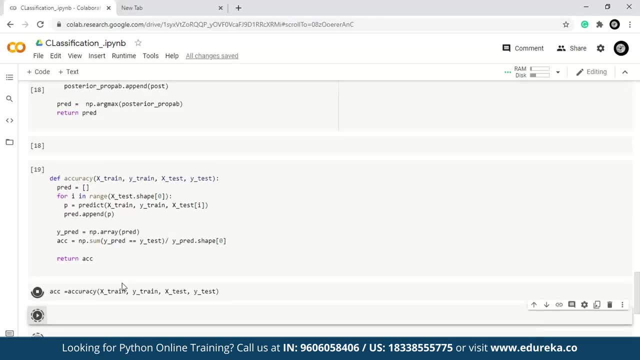 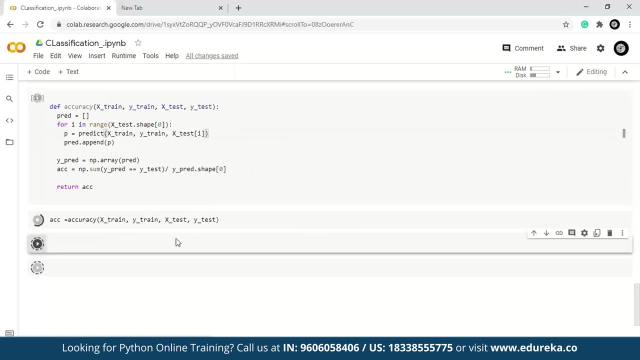 Multiple lines over here, right? You know one block might get executed before and then other later, So let's see if this works this time. have restarted the runtime in order to run it from the beginning, So let's, I hope it should work now. 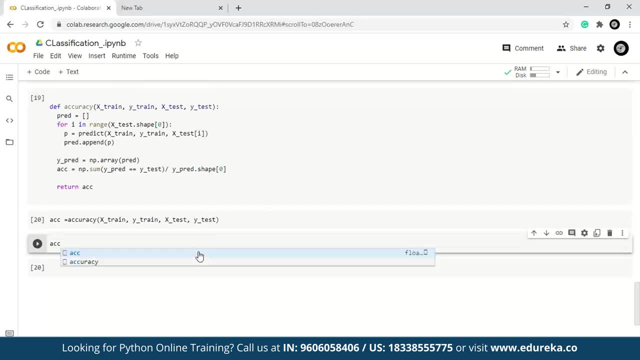 So now we don't have any errors. So let us now quickly see what is the accuracy that we got. So let's now print this. Okay, So we have got 0.99, right? So let me quickly give this over here. accuracy times: hundred. 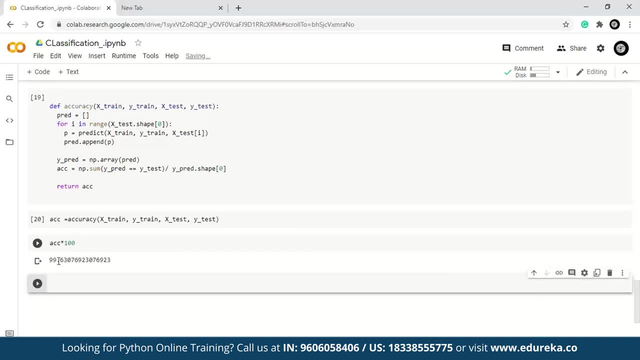 So now, when we perform this classification task here, we are getting 99.6.. 3 accuracy. So this is how we can perform classification task using knife-based algorithm. All right now. So, now that we know how NLP works, now that we know what is knife-based classification, 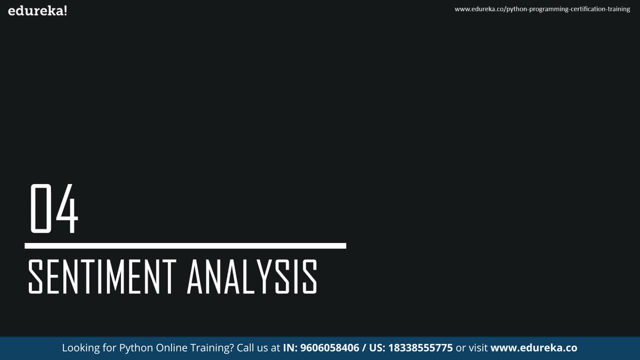 and how knife-based classification works, and we also know how to pre-process our data. Let's do one thing: Let's take certain amount of sentences, Let it be a small sentence and let's see if we can perform any kind of sentiment analysis on them, and over here will be using a library called as sklearn, with sklearn. 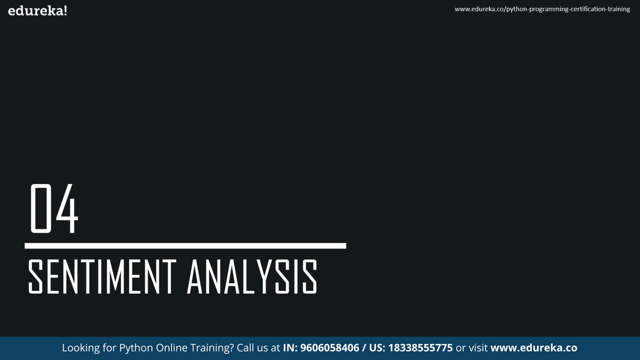 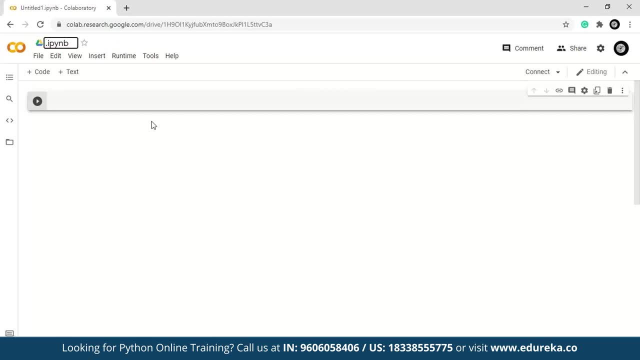 We don't have to write all the number of lines that we wrote now. Let me now quickly move to my code editor and show you how I can implement that. Okay, So now let's change the name here. Let's give it a sentiment analysis. 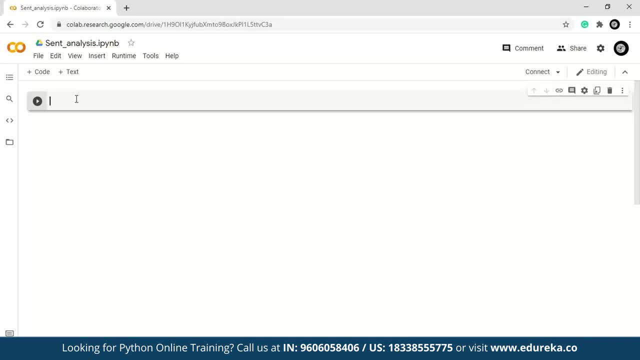 Okay, So what we'll do is I will have a text over here and we won't have a huge amount of data, because if you have huge amount of data, then it would be pretty hard to understand. So let me get this textual data for you. 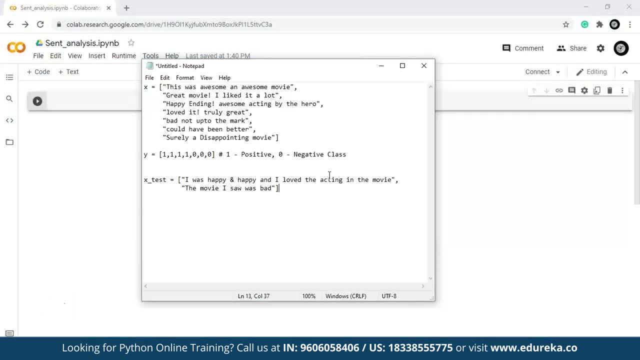 Okay, So over here in my notepad I have some small amount of data, I know So over here, as you can see. so we have X test, So this is going to be X train, and then we have Y train. So let's now analyze our data over here. 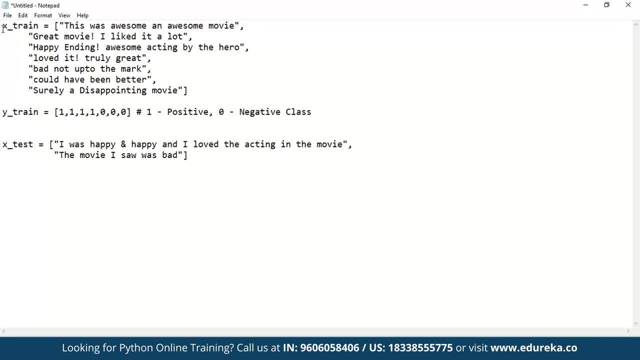 So, if you can see right, what is happening here is we have a data set and we're supposed to train our model based on this and we also have classes over here. This class over here represents that, whether this first sentence is a positive or negative sentence, 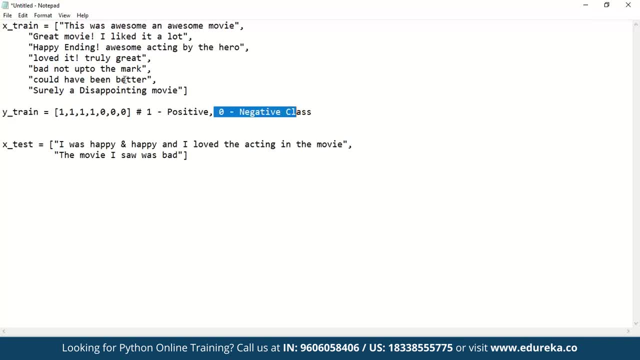 So if it is a positive, it is one, and if it's a negative class, it's going to be zero, so on and so forth. We have it for all the movie rating predictions here. Okay, And now, once we are done training a model, let's we'll test it by passing this values. 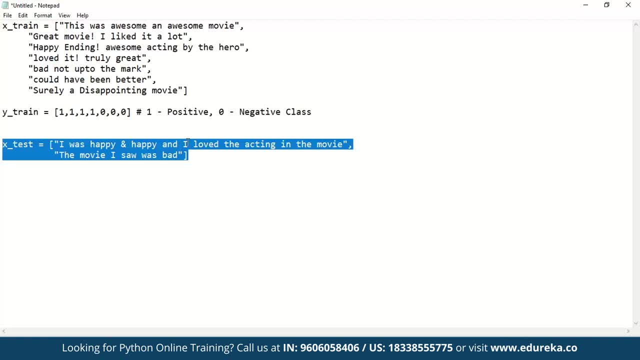 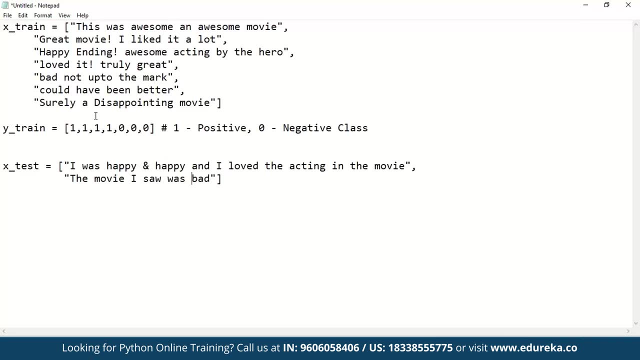 Okay, So over here we have three sentence: I was happy and happy and I love acting in the movie, and then the movie I saw was bad, and we can add some more examples. So what we'll do now is let me copy this part over here X test and let me paste it for our 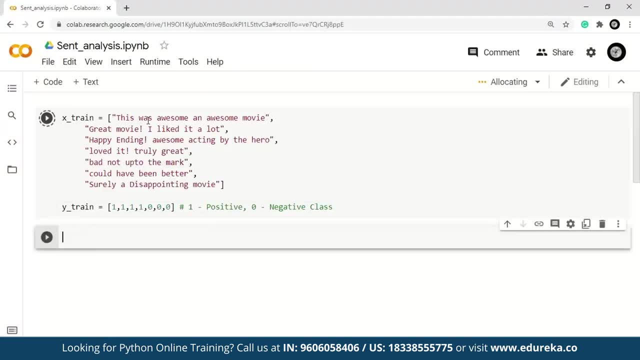 data set. Okay, And let me quickly execute this. Okay. So let's now see the shape of our X. Let's try making this an uppercase, and the reason why I'm using uppercase- your specifically- and lowercase, and why this? because there's a standard in the data science community. 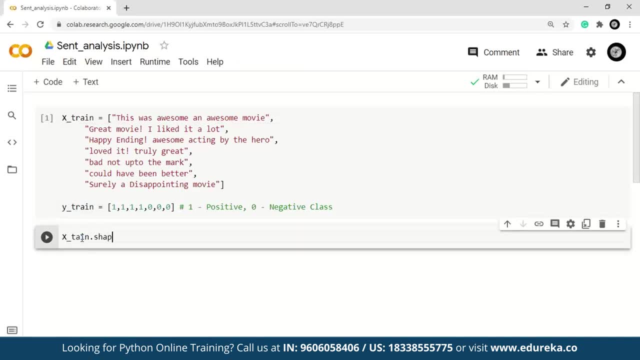 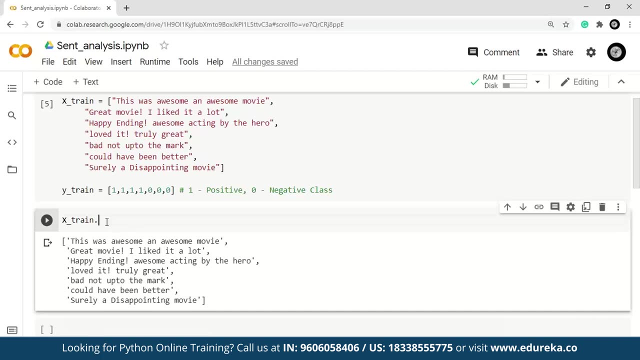 All right. So let's see the shape of our training data set, All right, and then we'll have extreme, Okay. So, as you can see, we have a data set here and let's have shape. Yeah, we won't get the shape here because it's not a numpy array. 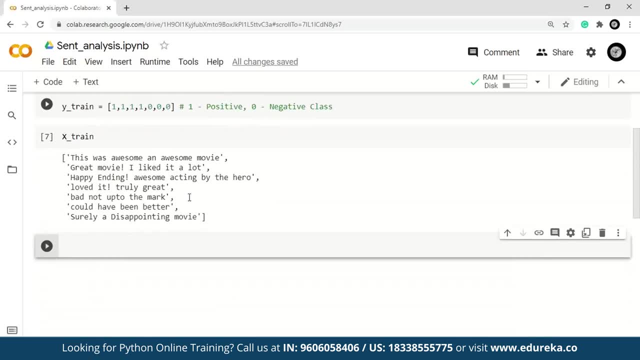 Right, So this is extreme fine. So now what we'll do is we have to clean our data, right, So let's do the data cleaning part, but in we'll be doing all kind of stuff like tokenization, stemming and stop out removal. 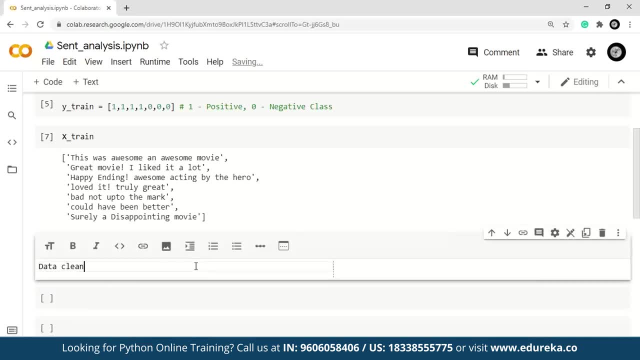 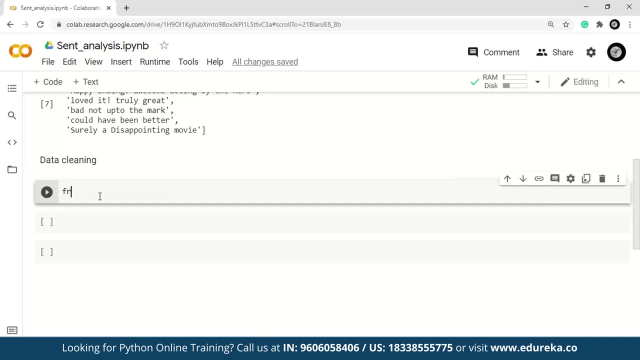 Okay, so let's give a heading here as data cleaning. And now, rather than writing this as an individual function, what I'll do is I'll write it as the entire method. Okay, So let's import our values first from NLTK. not tokenized: import regular expression tokenizer. 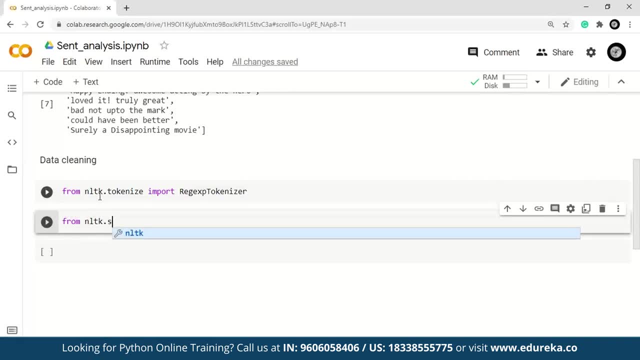 and then we have from NLTK dot stem Port, Let's import Porter stemmer. And then, finally, we have to have a stop word removal Right. So from NLTK dot corpus, Import stop words. So let me now download our stop words. 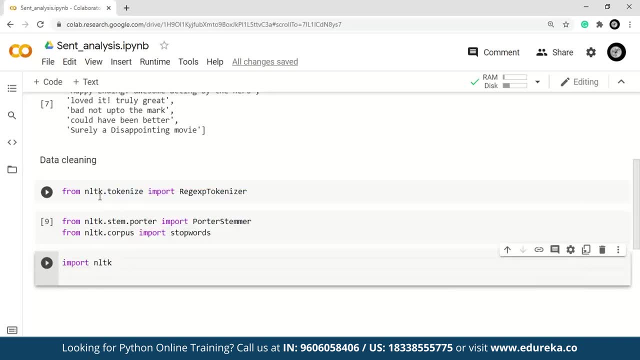 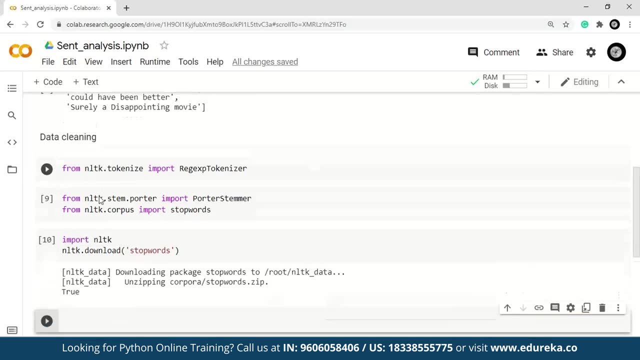 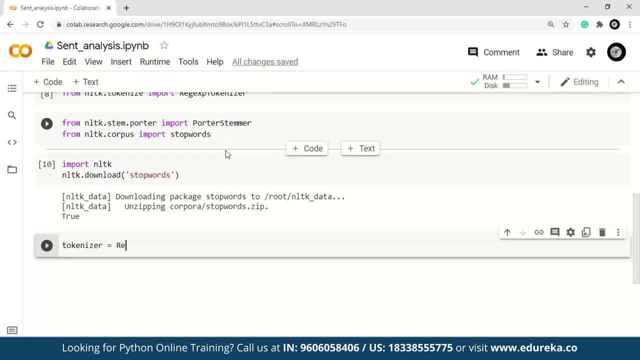 So: import NLTK, and then we are going to have NLTK dot download, stop words. All right, So now, let's now create an object of our Tokenizer, Porter, stemmer and stop words. This is going to be regular expression tokenizer, And then I'm going to pass what pattern I want. 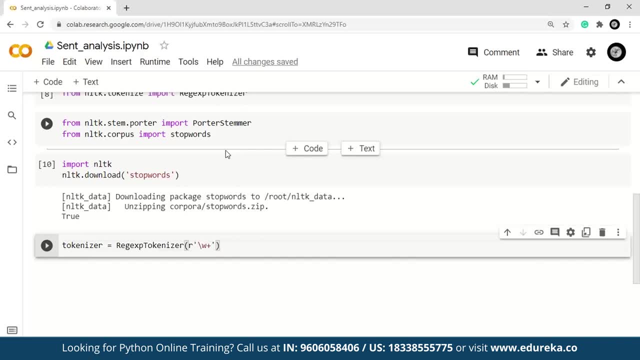 Right. So I want only the words, and then I also want to concatenate those words, And then we have stop words. So which language I'm using? I'm obviously using English. So stop words. This is going to be a city. stop words. 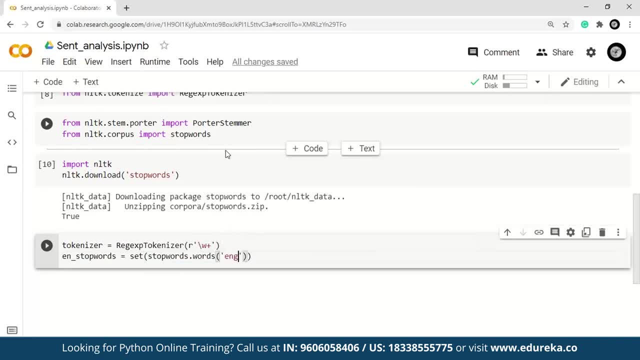 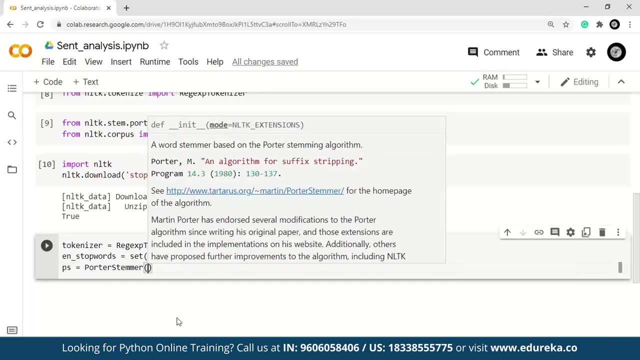 Dot words. It's going to be English, And now we have Porter stemmer. That's PS is equal to Porter stemmer. All I've done over here is just creating the object of our classes over here, So let me quickly execute this. 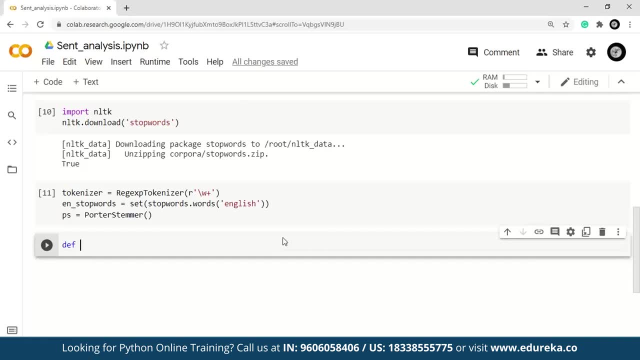 Fine, And now we'll create a function or a method- Def- Get clean data- And then we're going to pass here as text: Fine, And what we'll do is we'll convert our text into lowercase And now we'll perform tokenization. 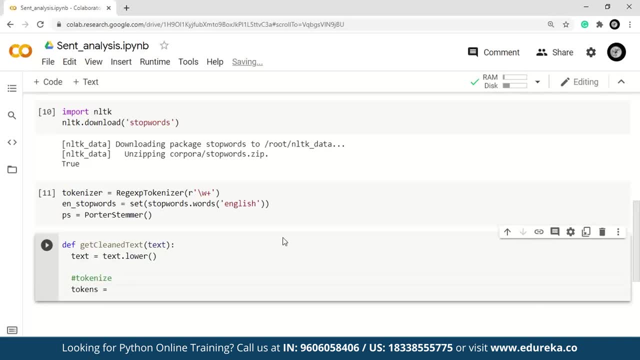 So there's nothing but tokens There'll be is equal to tokenizer. You're getting this tokenizer from here. Dot tokenize- Do we want the text to be tokenized? And then new tokens. They call to token for token in tokens, Because we are getting a list over here, right? 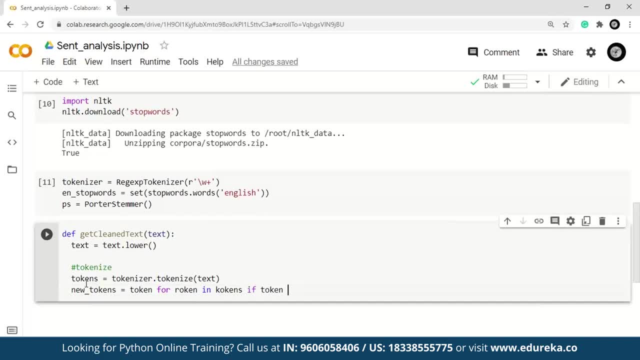 For tokens in tokens. What I'm trying to do here is I'm just combining stop word remover and tokenizer, Right, So that's why I'm using another for the list over here. So this part over here for token: Okay. for token in tokens, right. 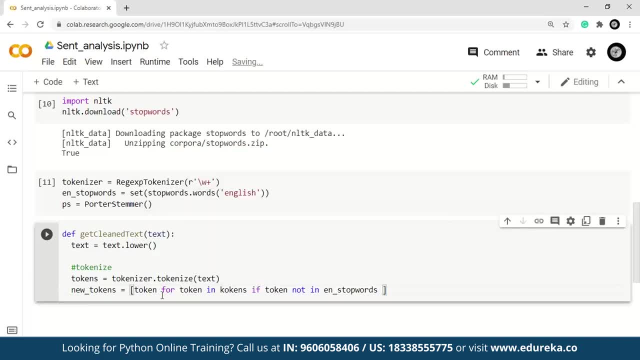 Okay, this part over here gets me the list of tokens, And then what I'm going to do is I'm going to compare this tokens with stock word list And if that word isn't present, then I print it. Basically, I'm performing tokenization. 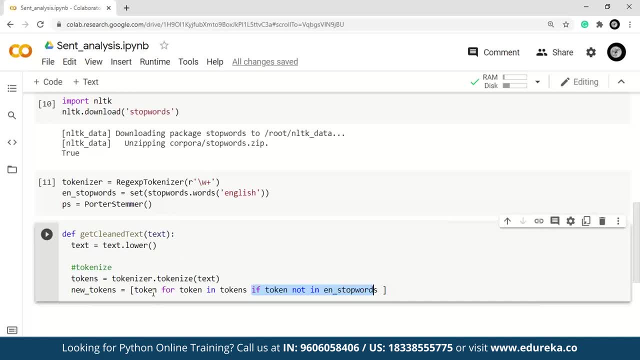 And then what I'm going to do is I'm going to compare this tokens with stock word list, And if that word isn't present, Then I'm performing tokenization as well as stop word removal at the same time, And now we'll perform stemming. 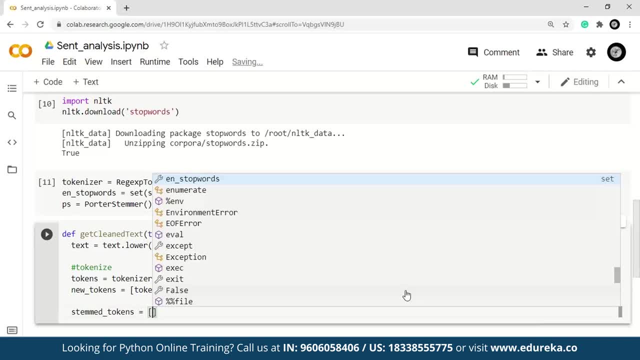 Same way like before, I'm going to give less comprehension. So PS. PS is the name that we have again. Porta stemmer dot stem. Obviously, it's going to be words, right. So for tokens in new token. 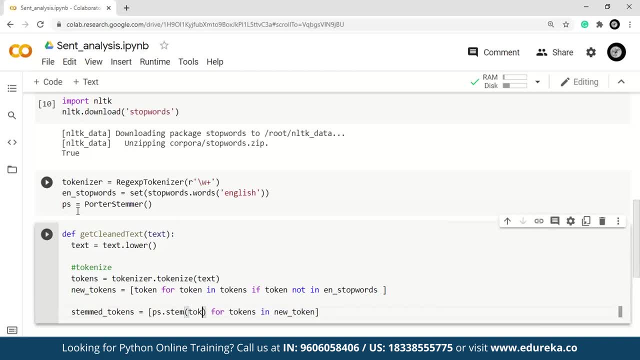 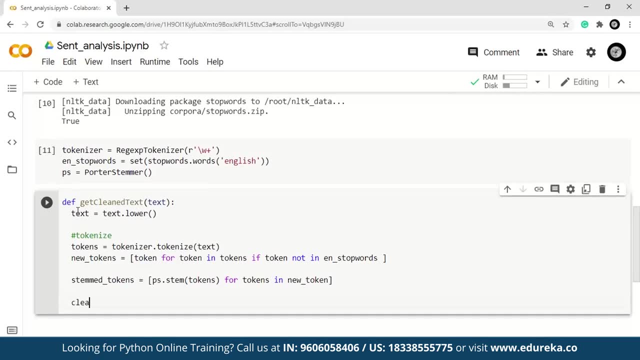 What I'm going to do is I want them to be stemmed Token. Okay, And now what's going to happen is Here I'll have sentence, or let it be like clean text. This is going to be join Stem tokens, right. 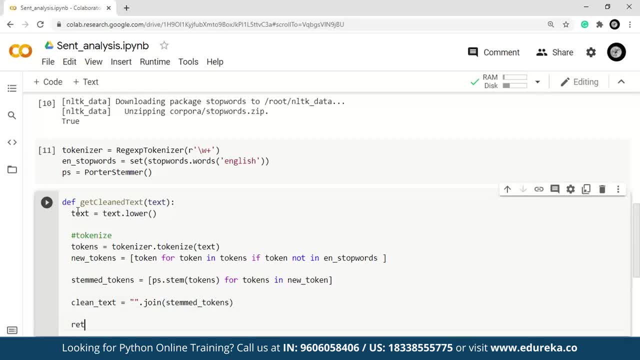 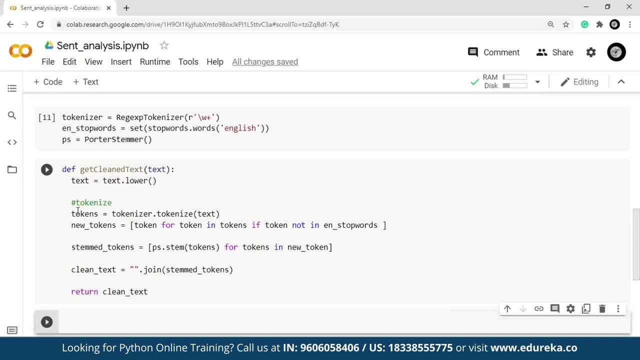 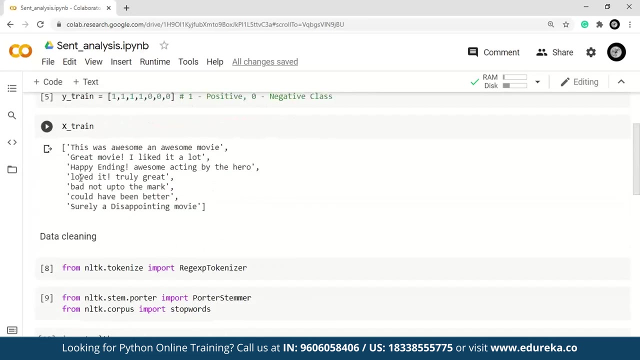 And what this method will return is the clean text. So let me quickly execute this now. All right, So this is done from our end now. All right. So now what I'm going to do is I'm going to use this get clean text to clean our text data and train data right. 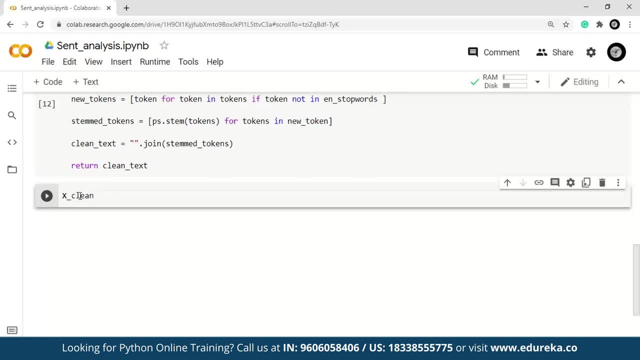 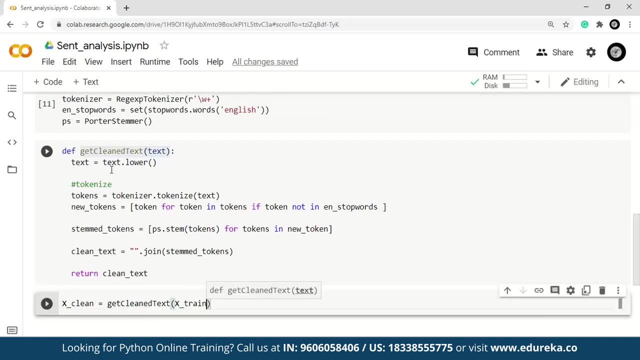 So what I'm going to give here is X clean, Okay. X clean is going to be get clean text, Okay, And I'm going to pass X train. Similarly, I'm going to do it for X test. So for that, I'm going to do XT underscore clean. 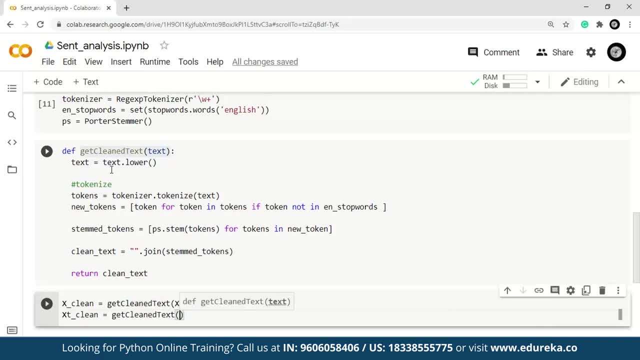 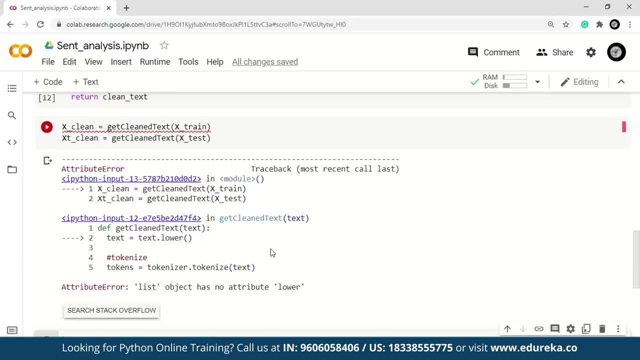 And this is going to be get clean data And it's going to be Y- Sorry, X- test, All right, So let me now execute this. Okay, So we are getting an error over here saying that you know, this word over here has no attribute. 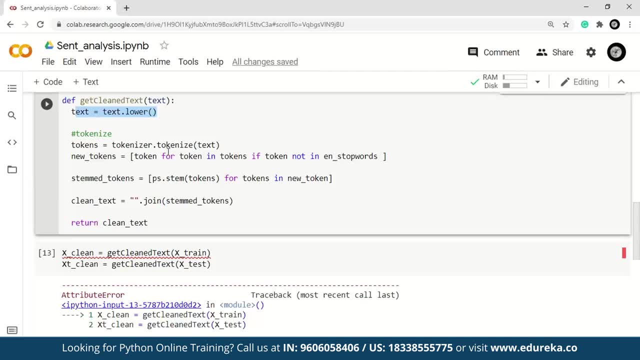 That's very true. The reason why we are getting this is because I'm just passing the value right, So we don't want that. So what I'm going to do is I'm going to put this in a form of a list here. 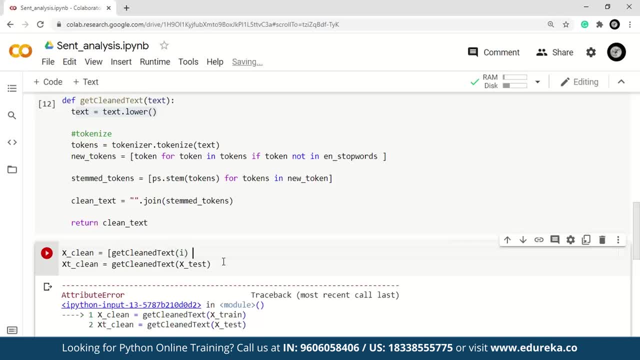 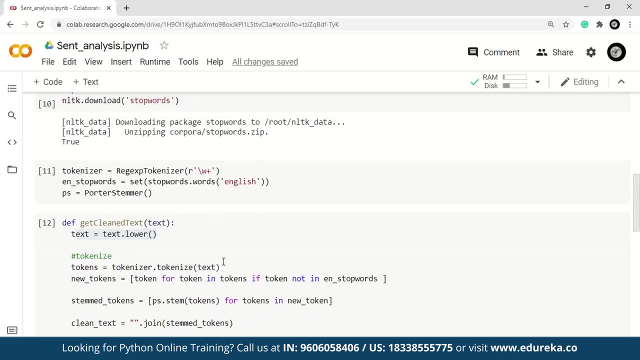 And rather than passing the entire extreme, I'll just give one word and pass for I in extreme. Sorry. And now, similarly, I'm going to do here For I in X test. So, yeah, Okay, We haven't defined our X test yet. 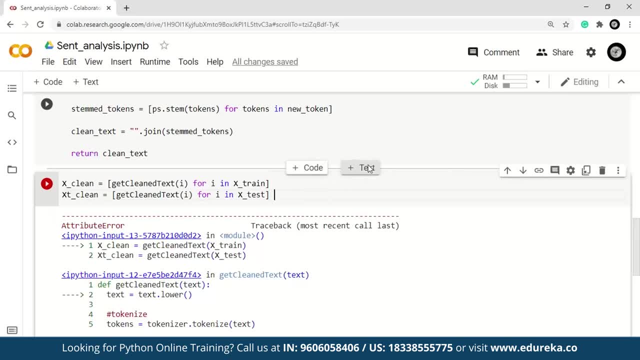 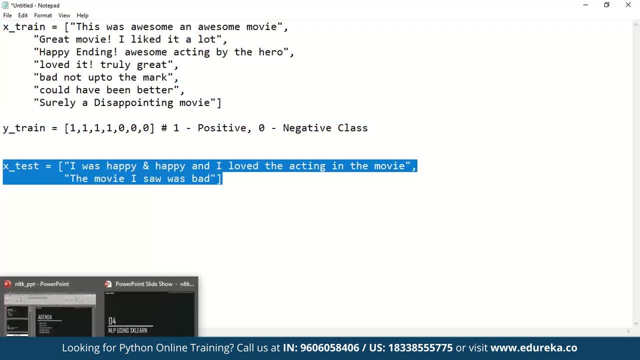 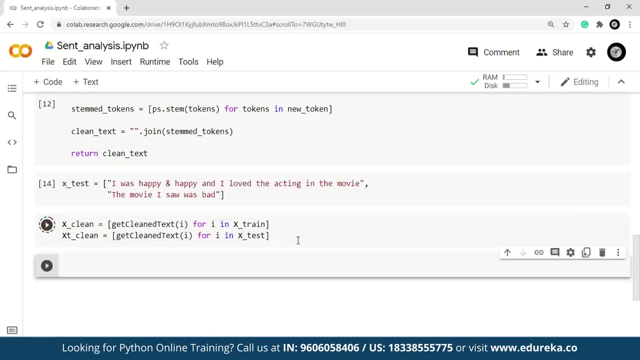 So let's quickly define our X test, All right, So let me get this coding part over here And let me get my X test. So I'll copy the X test from here And let me paste it here. Fine, So let us now execute this. 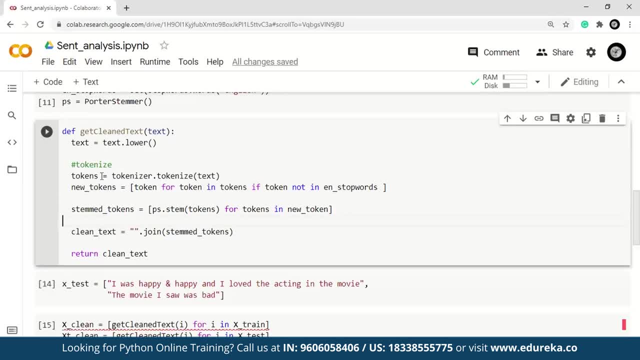 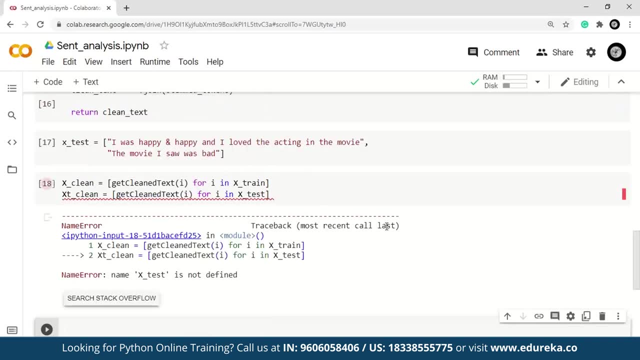 Okay, The reason why we are getting an arrow here is because over here I have defined as new tokens And here it is new token, right, So let me quickly fix that. And then this: once again it says X test is not defined. 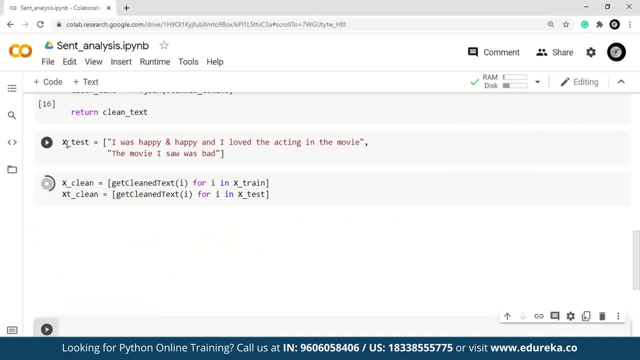 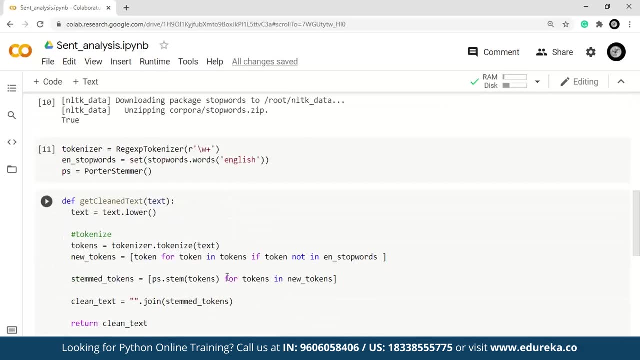 Yep, So we will fix this and rerun this again. Most of the times when you're trying to do this program right, You'll encounter a lot of issues, And only when you encounter these issues you're going to learn a lot. 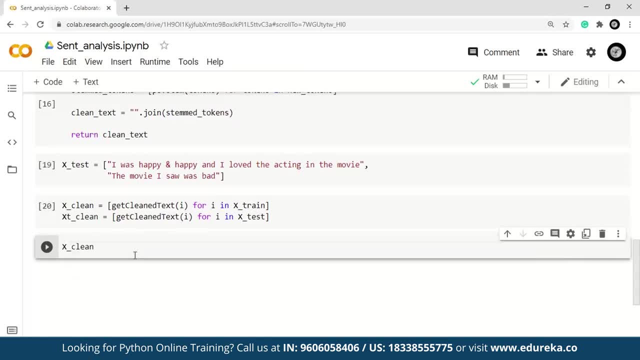 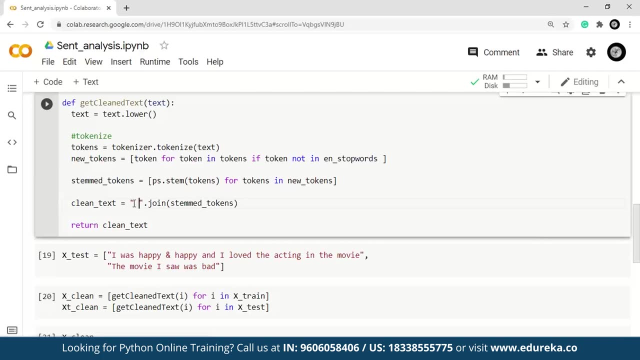 So now we have our clean text, So let's just compare it to and see how it looks. Okay, So, as you can see here, our text has been reduced, And yeah. So, in order to get this better, what I can do is I can just pass some space here. 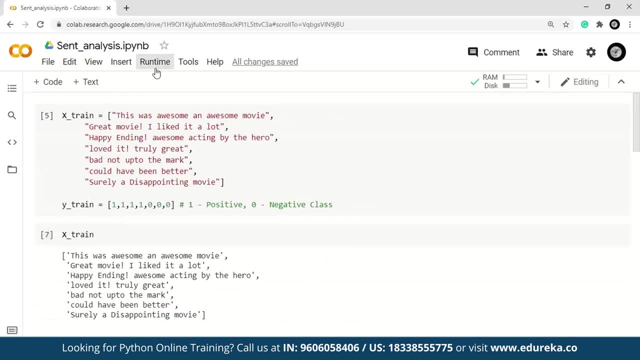 And then run this here. Let me do one thing: Let me rerun this from the start here and restart the timer, And let me run it all. Okay, So, as you can see here, now we are getting some spaces, All right, 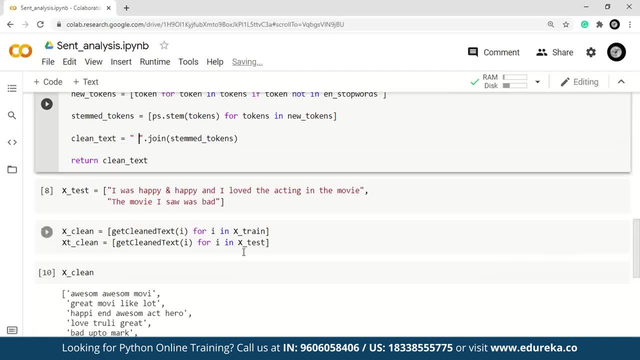 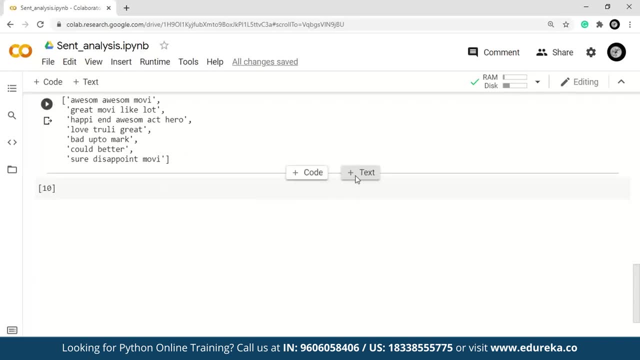 So the reason why we weren't getting any space is because I had not added any space. So now let's perform our classification task. Let's we'll be using an RTK. right before that. We have to vectorize our text, as I've mentioned, in order for us to perform classification. 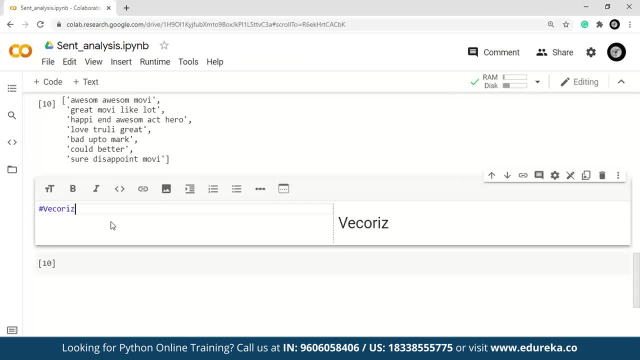 We need to vectorize it, So vectorize, Okay. So now what we'll do is from sklearnfeatureExtractiontext import countVectorizer. All right, And now we'll create the instance of our countVectorizer. cv is equal to countVectorizer. 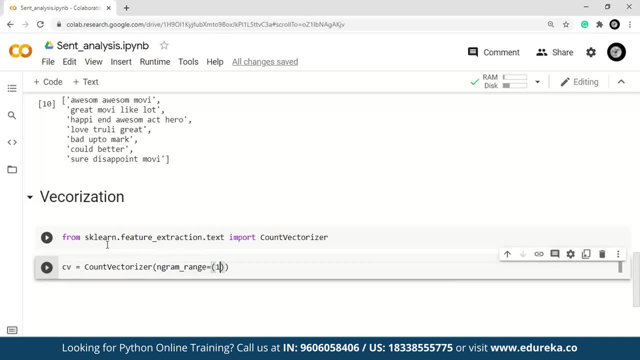 And we'll give our n-gram range. It's going to be 1 and 2.. And now to vectorize our input. So xVectorize is equal to cvfitTransform. And now we're going to pass this value, right. 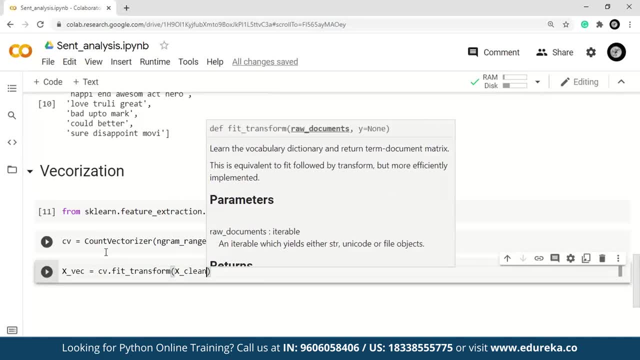 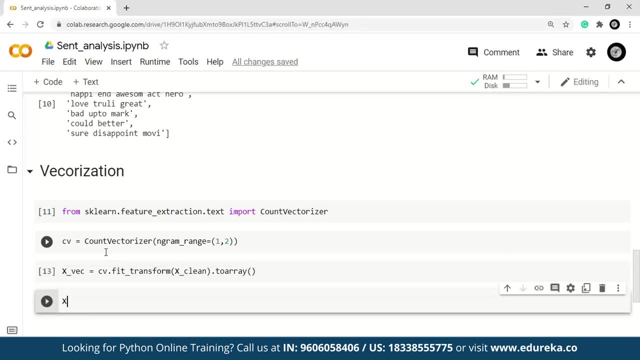 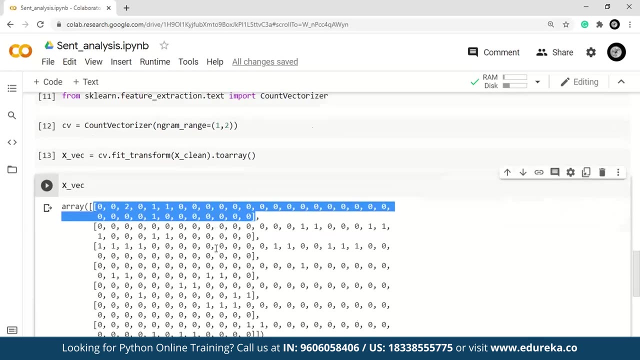 So we'll pass xclean And then we want to convert this into an array. So let us now execute this And let's see how this xVector looks like. Okay, So, basically for every word, you know, we are getting this vectorizer over here. 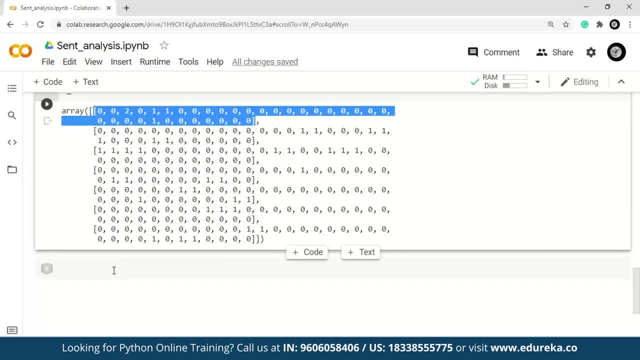 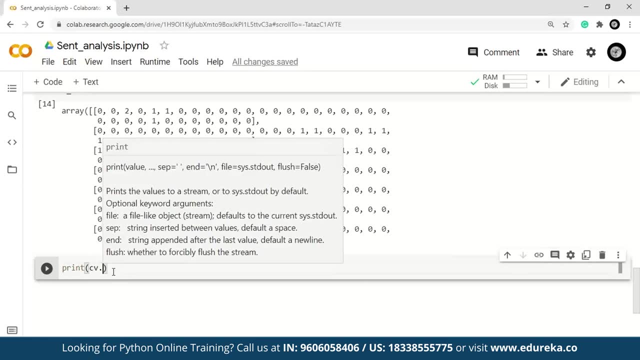 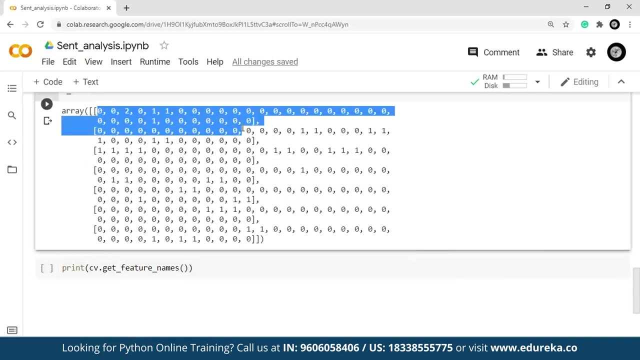 All right. So now what we're going to do is we are going to perform our classification task, But before that, let's get our feature names. Okay, So print cvgetFeatureNames. Okay. So what does getFeatureNames does is? we don't understand these values, right? 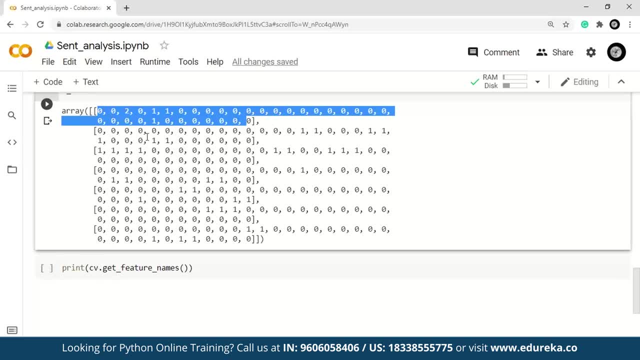 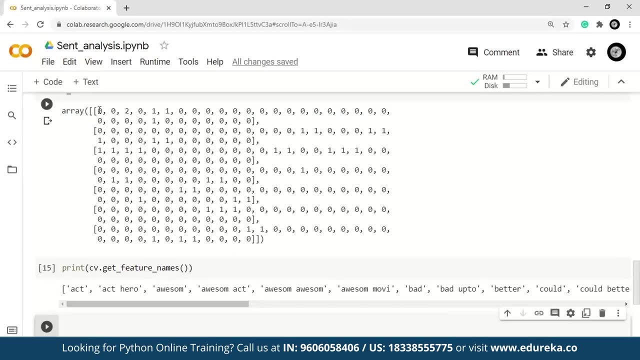 So you don't know what 0, 0, 2 here represents. So in order to know what values over here represents, all we need to do is getFeatureNames And, as you can see here, this first over here represents act. 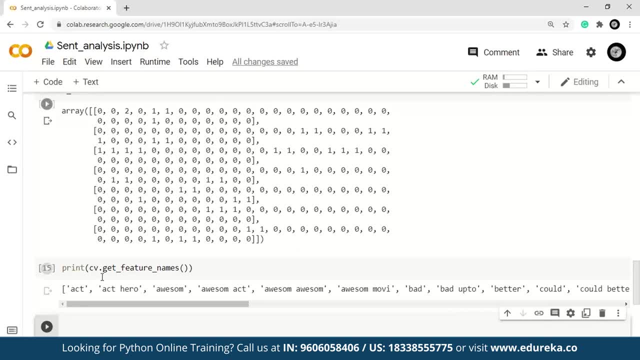 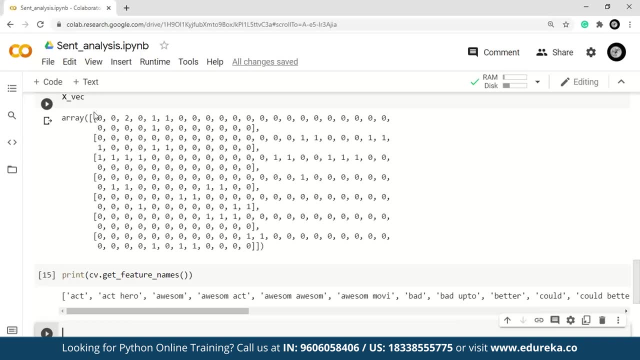 And it's the same for all the five arrays over here. So what, basically, this countVectorizer tells is that this word act- how many times has it repeated in this sentence? How many times it was present in this sentence? This is what vectorizer does. 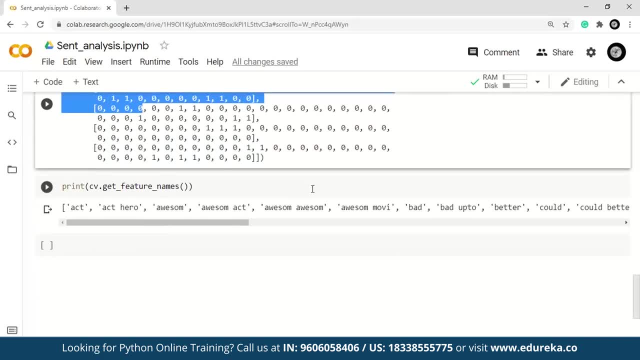 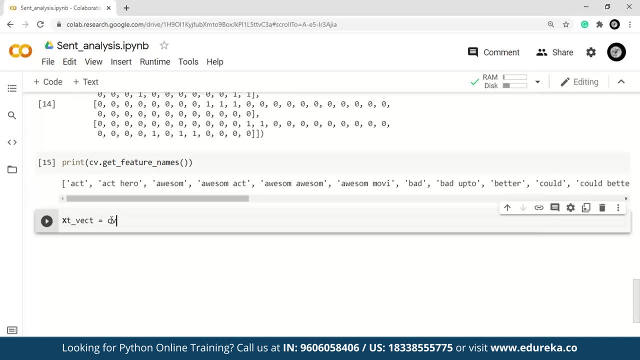 And this kind of model is usually referred to as bag of word model. Similarly, we'll perform a vectorization for our test value, So xtest, cvtransform, And now we have the clean text. And now we also want to convert into an array. 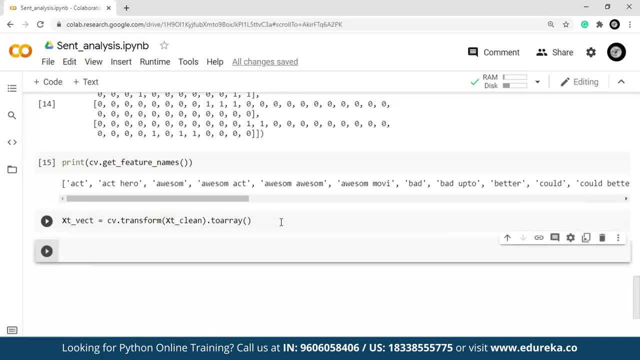 All right. So now let's execute this part here, Okay? And finally, we'll perform our classification task And we're going to use multinomial knife base here, Okay, If you don't know, there are multiple versions of knife base that are available. 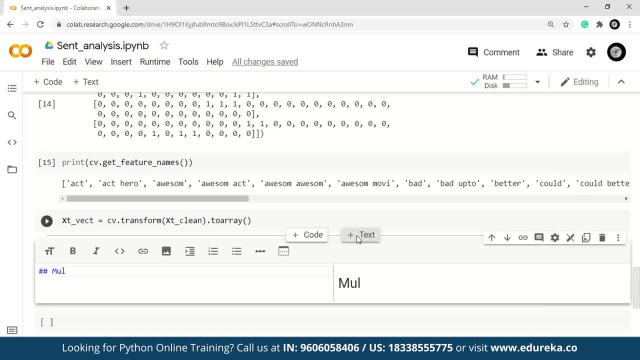 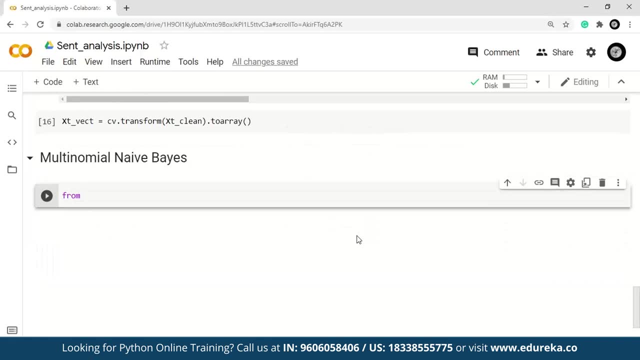 In order to perform text classification, we use multinomial knife base. Okay, So multinomial, All right. So let me import that from sklearnknifebase: Import multinomial knife base, And now we'll create the instance. So for that, so mn, and we'll give multinomial knife base. 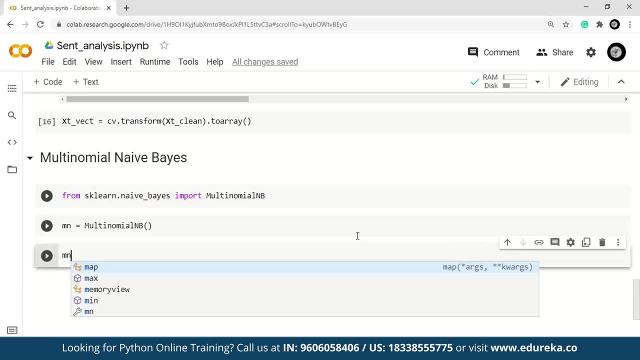 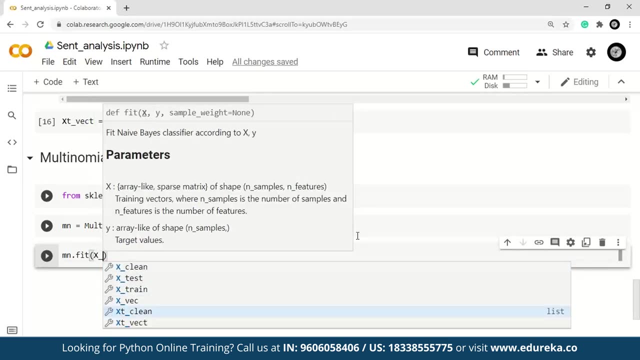 So we'll fit our model. So it'll be multinomial knife base, Dot fit And we'll give values. Okay, So it's going to be x vector. X vector is nothing, but in our vectorized form, which is nothing but this x vector. 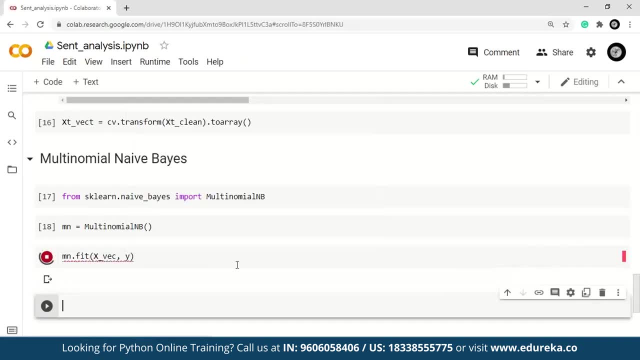 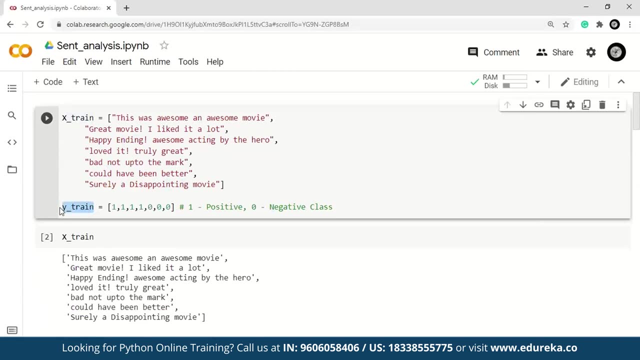 And then we're going to give y values, All right, And let me execute this. So it says y isn't defined. So let's go back here and see where we're going wrong. Oh yeah, It's not y, It's going to be y train. 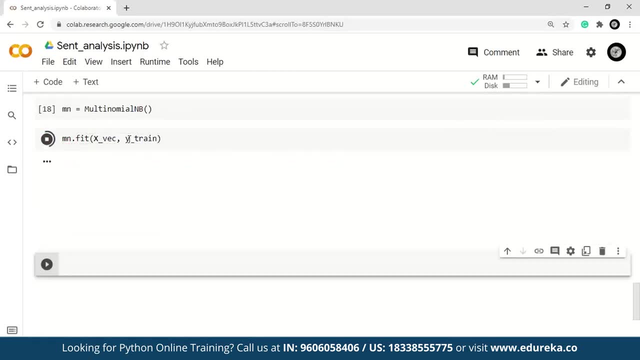 Right? So let's copy this and let me paste it over here And let me execute this program. So now we have our multinomial knife base And let us now perform prediction. So mn will return this value, Right, So it'll be like y pred. 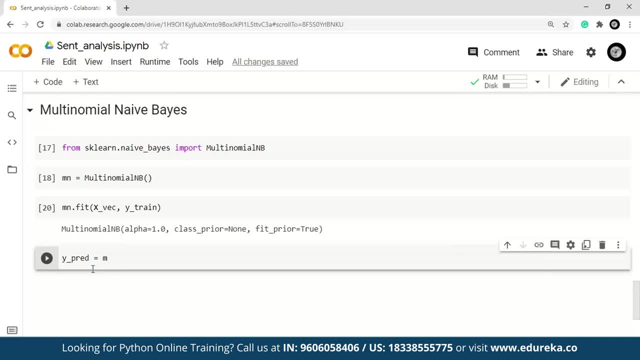 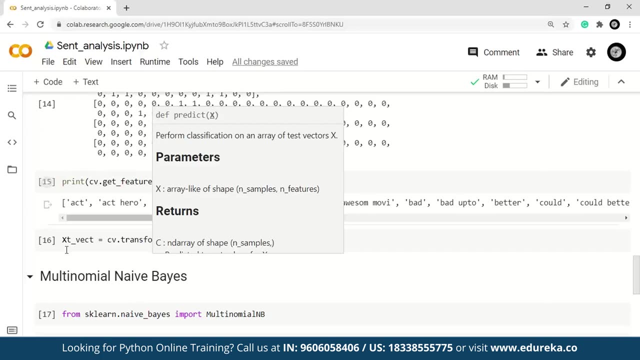 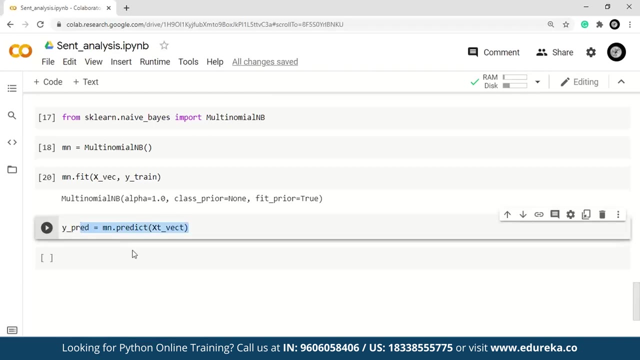 This is going to be mnb or mn- multinomial knife base dot predict. And over here we're going to pass the test value Right. So x text vector, Xt vector- Fine, So let's now see what will be the output for this. 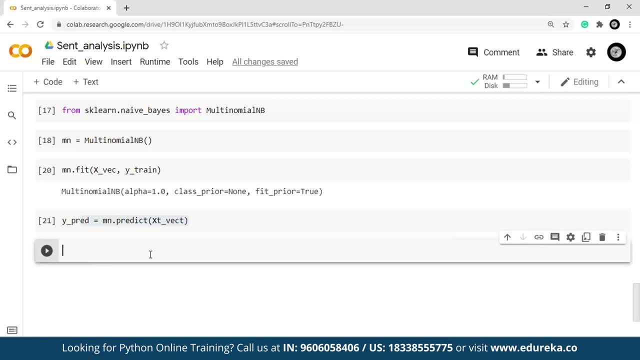 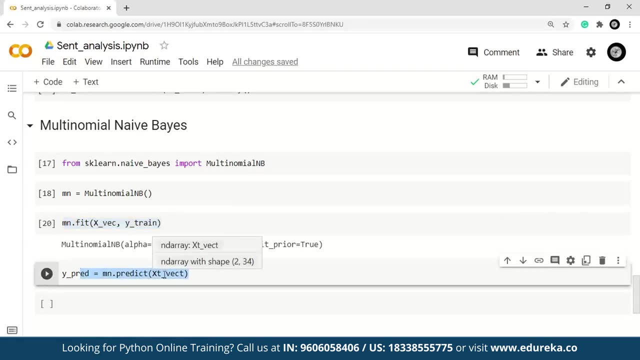 But before that, I would like you to guess what can be the output. Okay, See, we have performed classification task And now, by doing this, predict the value of Xt. All we are trying to do is predict whether that sentence belongs to class A or class B.